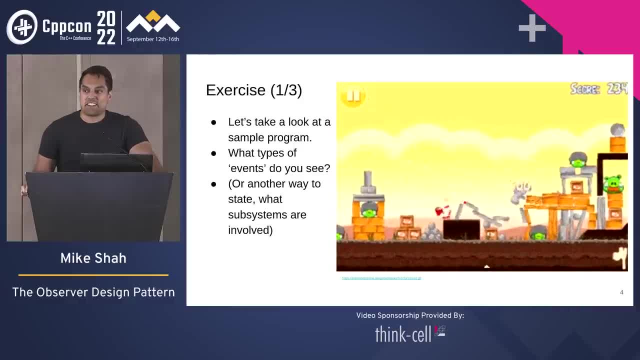 this bird crashing into this stone here? What else? Camera's moving? Yeah, camera's tracking the bird. What else Scores? You see them popping up here or on the right, tallying up What else. There's no sound in this clip, but we could imagine the bird screaming. 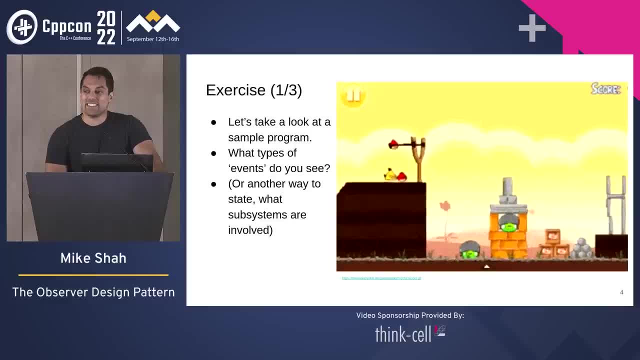 for those who have played. So anything else, I mean that's a pretty good list there, More than one, certainly right, Lots of things are happening in games, Usually pretty interesting systems to implement. You have a lot of things going on. You have a lot of things going on. You have a lot of. 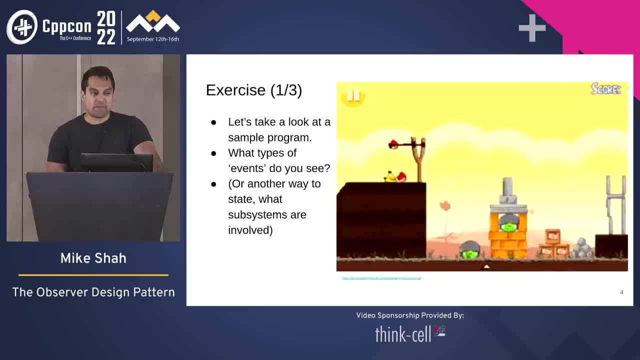 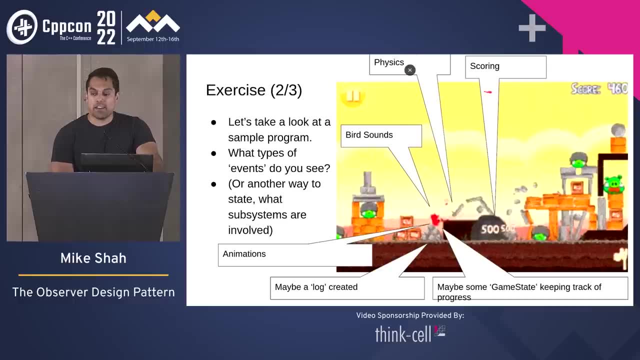 other types of requirements to build these types of games. So here's the list that I came up with. I think you folks had most of these right. There's physics going on with the collisions, scoring the birds animations. Maybe there's some logging also happening behind the scenes. 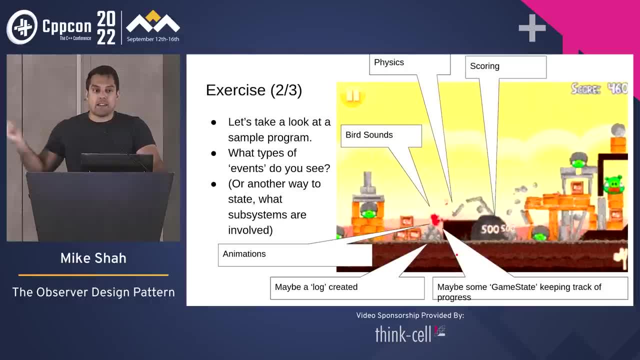 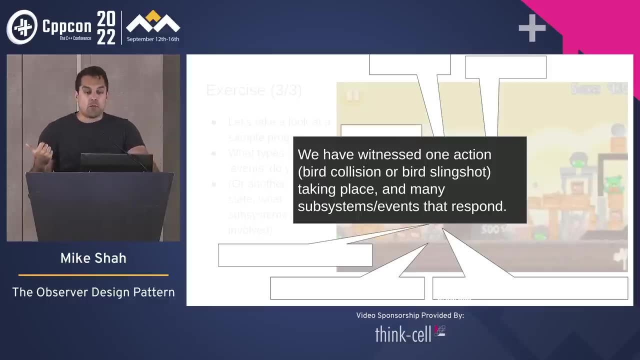 And maybe there's other types of game state and stuff being hidden in the background as well, Keeping track of how many birds you've shot or what level you're on, or these types of things. So lots going on here. So another way to look at this is we've just witnessed one action that's occurred or this sort. 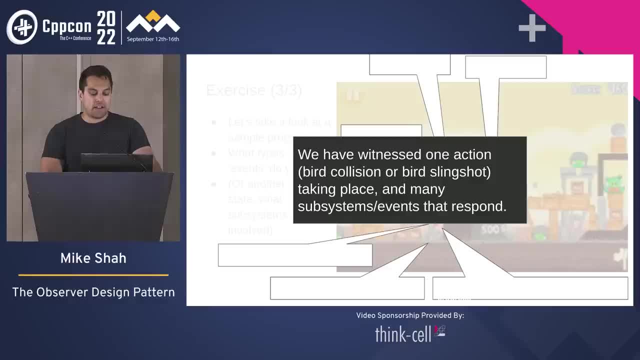 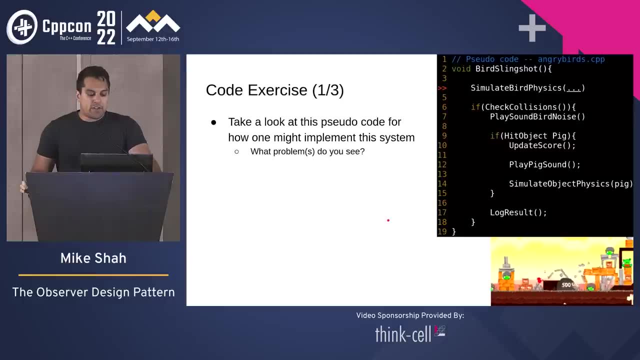 of one gameplay element of shooting the bird on the slingshot, But many again of these subsystems or events are evoked. okay. So here's a little coding exercise. So here's some code, a pseudocode I guess, that I wrote, And this could be one way to implement this sort of action, right? 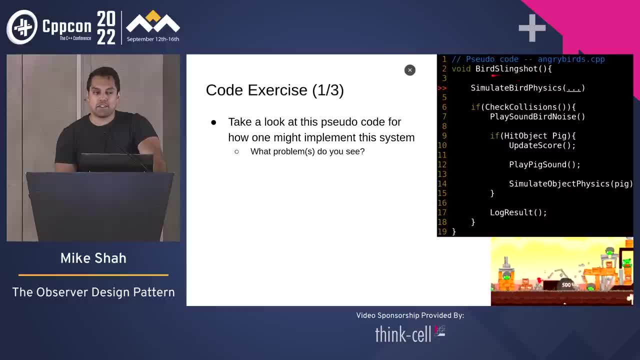 So you have this bird slingshot. So you have this bird slingshot function here And, you know, maybe you sort of simulate the bird physics and kind of send it out, And then you have, you know, check if there's a collision. 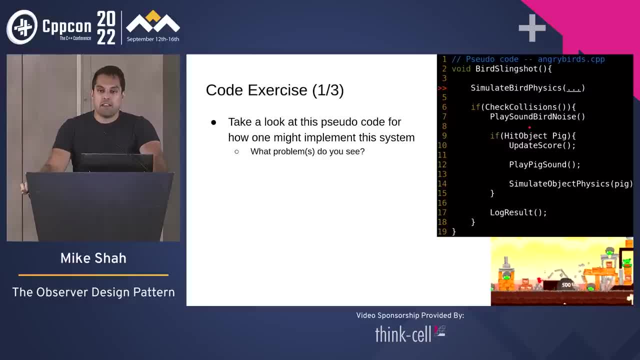 If there's a collision. you play some noise and do all these other sorts of things here. So I guess, what do folks think about this? Or I guess the way I can ask it is: what problems do you see with this type of code here? if you wrote this, What do folks think about this? Good code. 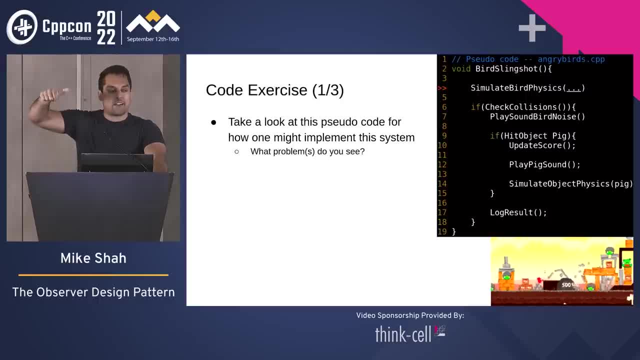 or bad code, Thumbs up for good, Thumbs up or down, Or maybe in the middle, If you don't care. It's like, yeah, sometimes you just got to get the code written. So let you kind of think about it And what I will say is, if you're, 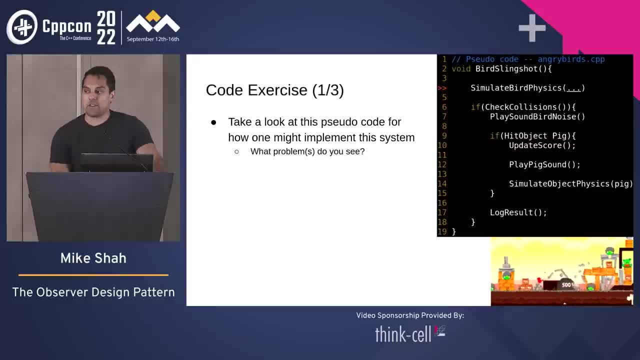 going to like. I want to sort of hide away from this code a little bit So you can take a picture, but I'm going to duck away Because this isn't the kind of code I would necessarily want to be responsible for, at least in a final product, And the problem that I'll tell you that I'm going to. 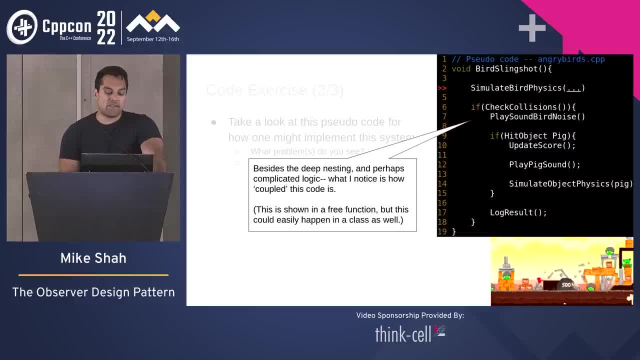 see here- and I'm guilty of writing code like this, you know, at different times, But you know there's some deep nesting here. The logic's kind of getting complicated. But really the problem that I'm seeing here and again this you know you have to kind of look at it a little bit. But 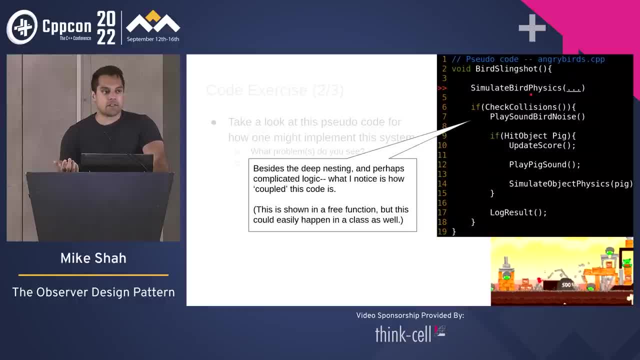 there's a lot of coupling going on here. There's different systems that have different sort of goals. right, We're slinging the bird around with the physics system and doing collisions, But we're also, you know, keeping track of our sound system. 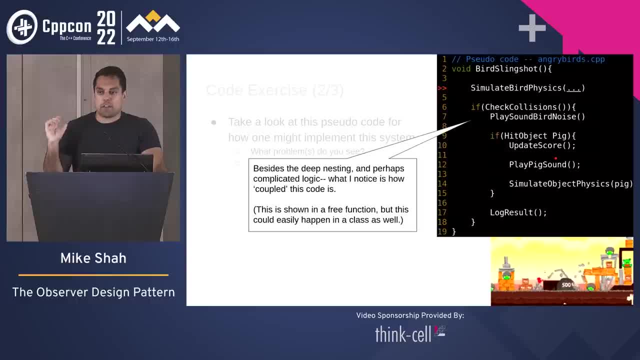 And, you know, updating our score. So there's a lot of different things you could imagine if one programmer had to work on this project. They have to understand sound, physics, animation, you know, whatever else is being thrown into this function, Or maybe this collection of objects, Okay. 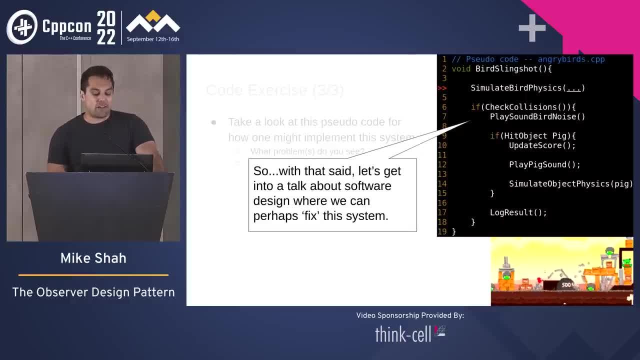 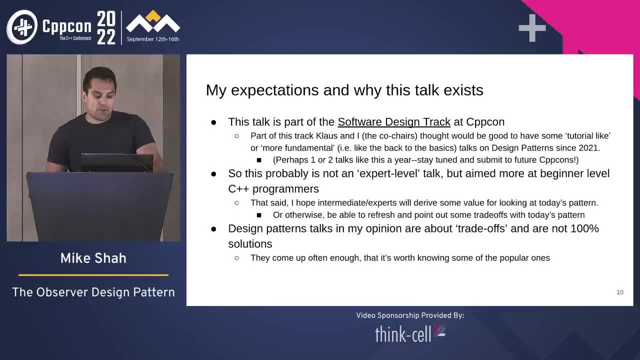 So, with that said, again, this is going to be a talk about software design And perhaps we can fix or clean up this system in some way to write some better code. So you know why this talk exists or is part of. 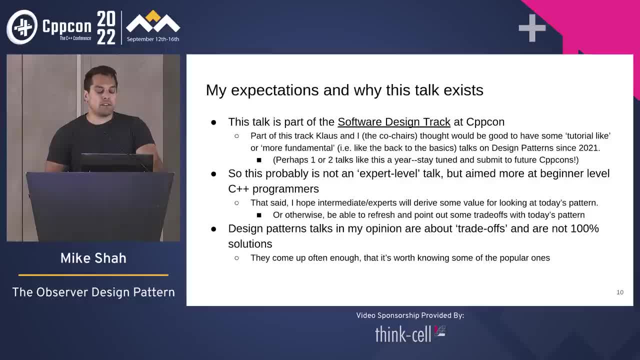 this is part of the software development track, as I mentioned, which Klaus and I came up with a year ago, And we wanted some talks that went over some what we think are fundamental design patterns and almost a more tutorial style to take part in this. So, again, it's probably not. 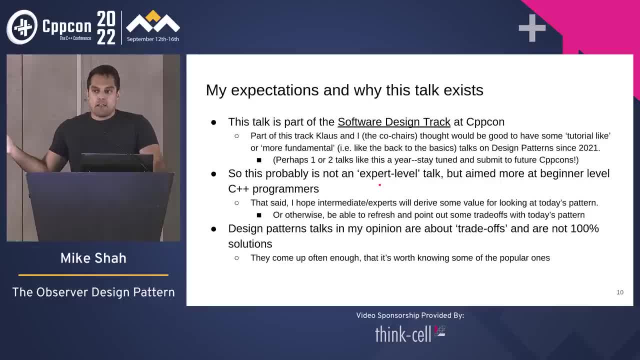 an expert level talk, but I hope it's beginner friendly. But also, you know, even if you are an expert, you can start to think about how to advance some of these systems once you have the foundations. talk Foundations of this. talk now. 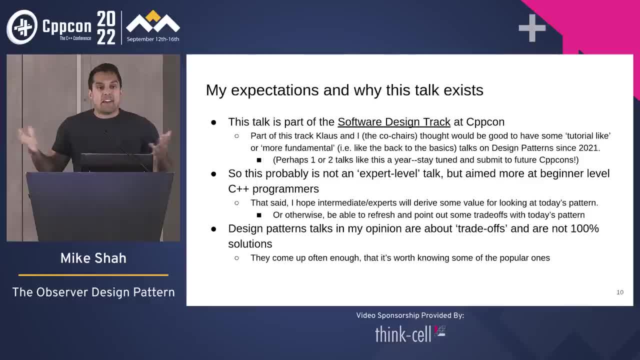 But with every design pattern and even what I'm going to show you today and software engineering in general, it's all about tradeoffs. So this isn't going to be a perfect pattern that we're going to look at today, but we're going to see if it can help us with that Angry Birds problem that we are working on. 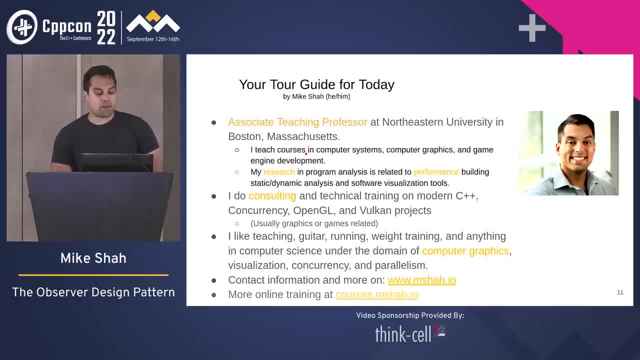 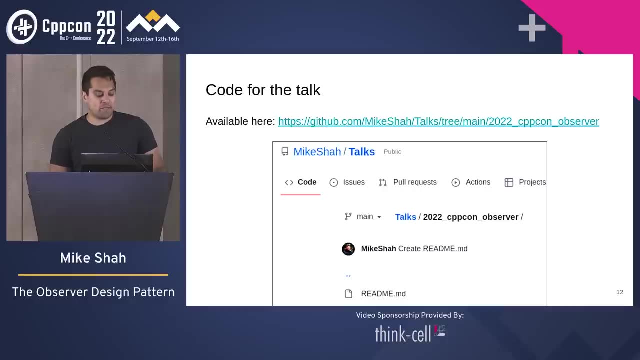 All right, So I'm your guide for today. You can take a look at this, but I'm primarily associate teaching professor- Here's my website- And then I do various consulting and C++ and graphics applications. The code for this talk will be available and there will be full examples that compile, So feel free to check those out after. 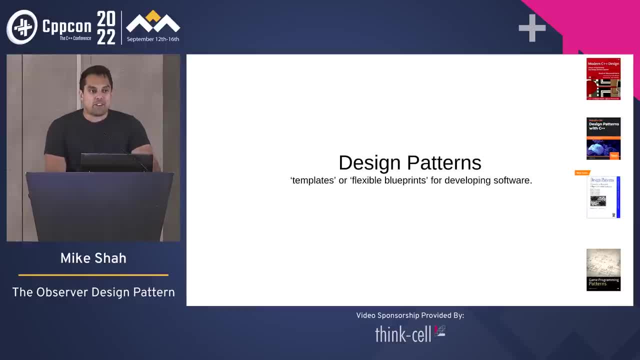 But, with that said, let's go ahead and get into design patterns. So, again, if you're at this talk, you probably understand a little bit about what they are, but they're templates, or, again, a better way to think about them is. 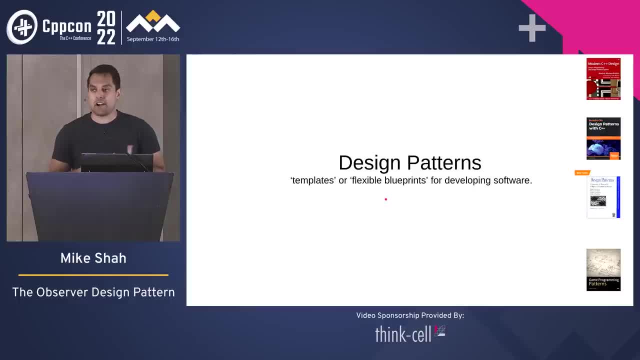 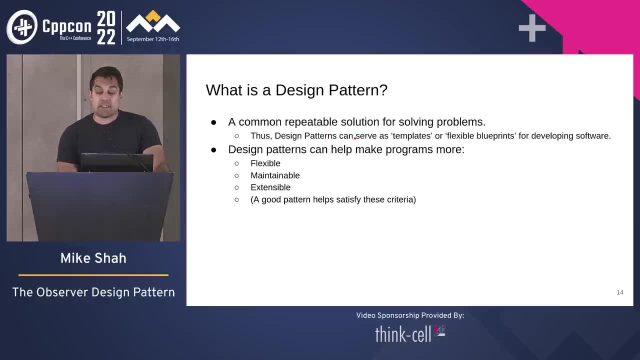 flexible blueprints for developing software. They give you a rough idea of how you might want to solve some problem that keeps reoccurring in software. OK, so typically we say they're repeatable solutions. So you'll see these often if you look through different code bases. 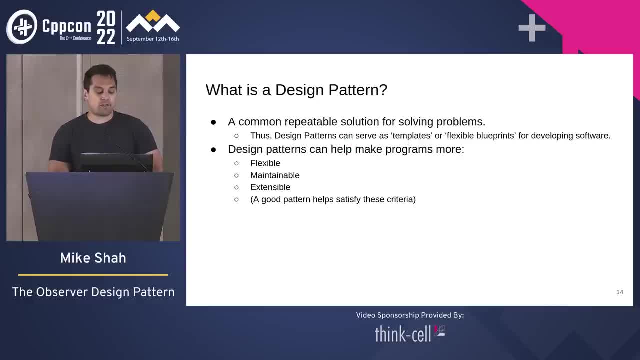 especially in specific domains, you might see some of these patterns show up more often than not. Now, in order for a design pattern to be useful, or what I think is again good code, it should have these three attributes, And we're going to look at these for some of the example code that I write today. It should be flexible, maintainable and extensible. 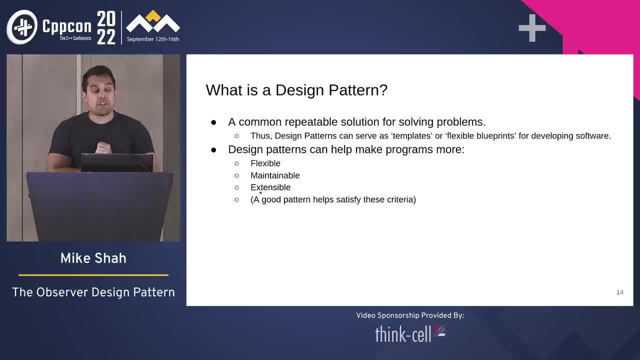 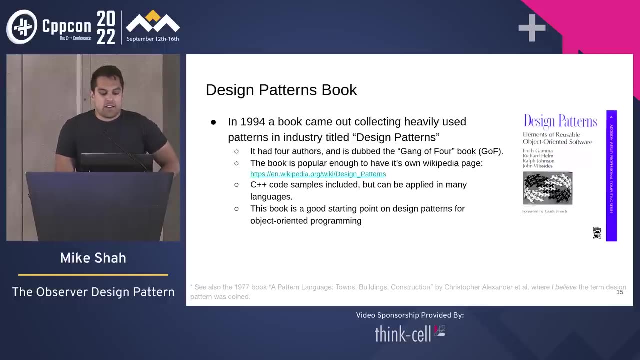 OK, Extensible, meaning if I added you to this team project you could probably add to it or build on the system. maintainable, Right, You could sort of have correct code, flexible. Maybe you could reuse pieces of it. That's the idea of a design pattern. Now, design patterns have been most popularized, I'd say, by this book in 1994.. 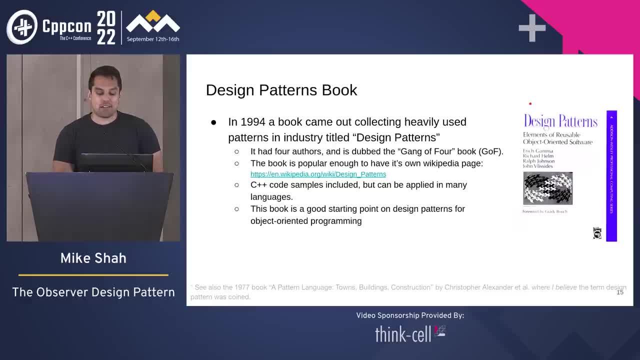 I think folks in the audience here might know this, but this is the Gang of Four, a design patterns book, And, as I was talking before this, wow, it's almost 30 years old but still highly relevant to how we develop software or at least study software. 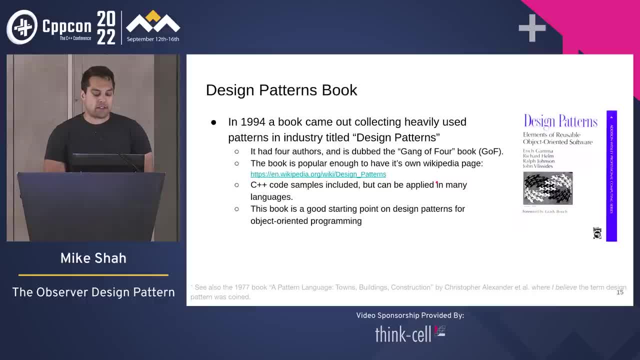 So you know it has its own wiki page so you can look at some of the other design patterns, But what this book really captures is, I'll say, about twenty three or so of the most popular patterns. Now there's hundreds of patterns. There's older books in this and so on that that you might look at. 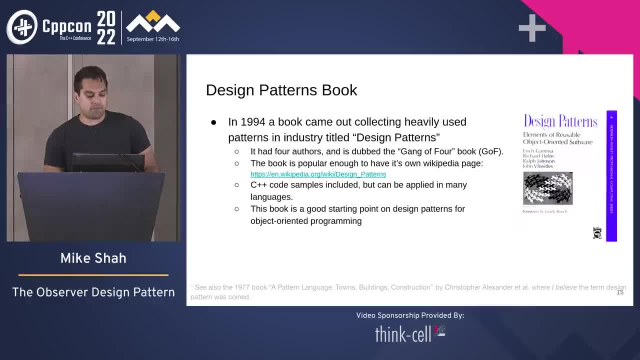 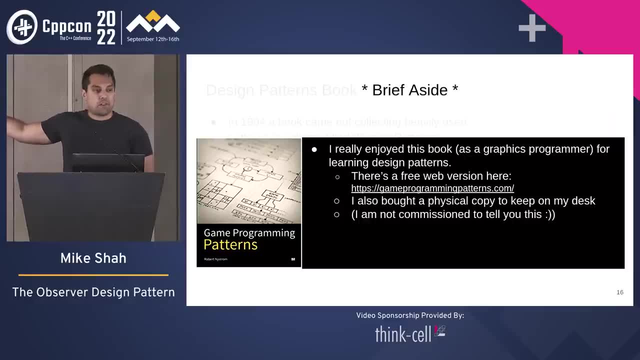 And there's lots of other wonderful software architecture books And there's lots of other things that are also coming out. So one of those that I do want to highlight and that'll be useful for this or for study later is this book called The Game Programming Patterns Book, written by Bob Nystrom. 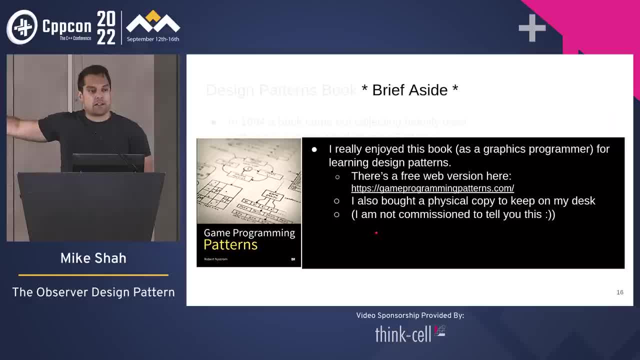 And it's a freely available book. So I'd highly recommend reading their section on The Observer or just, you know, any of the book. I read the book and then I was like you know, it was free online. It's like I have to buy this book And, as I say, I'm not commissioned to tell you this. 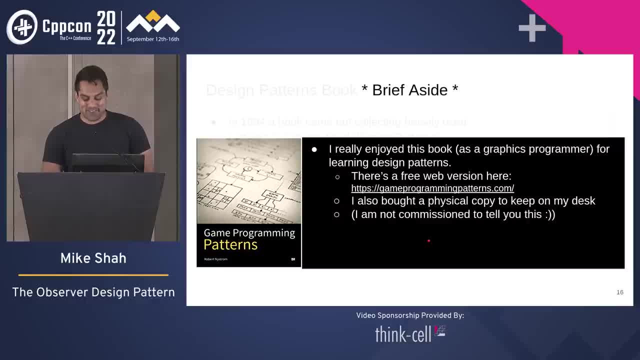 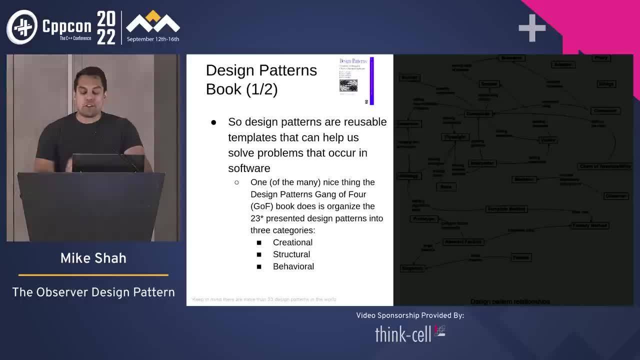 I just really like this book, So I support your author here. So back to the design patterns again, these reusable templates. One of the things that I think is useful when understanding design patterns or any software in general where you're trying to look at it, is to try to fit it into some category. 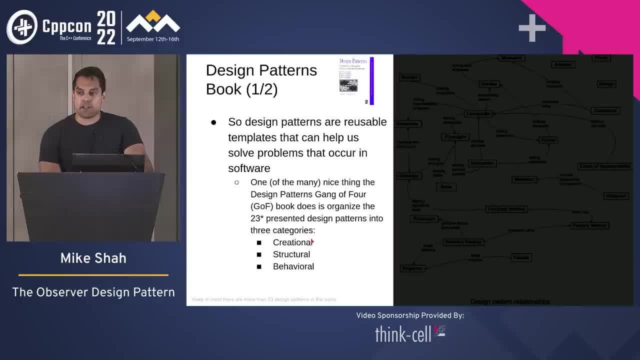 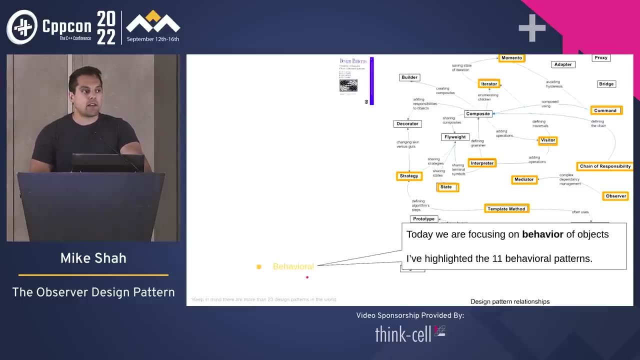 And I think that's one of the useful things that this book does is it breaks our design patterns into creational, structural and behavioral categories. So creational, How you sort of create objects. structural, what your program looks like. and behavioral, which is what we're going to look at today, is going to focus on how objects or your code communicates with each other. 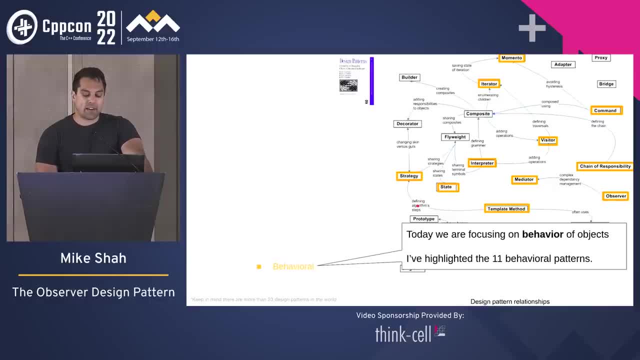 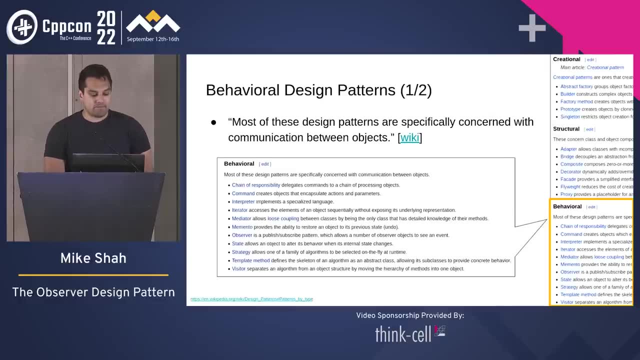 OK, so here's the behavioral patterns that are highlighted. some of them might be familiar, some might not, But of course we're going to be looking at the observer today. OK, so the observer pattern again falls under this category of behavioral. 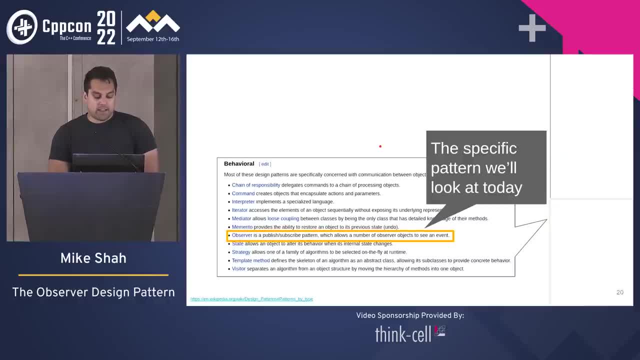 meaning that it's concerned with communication between objects and the idea of an observer in a sentence- And I'll show this again- is you have this sort of publish subscribe pattern which is going to allow some number of observers to see an event. All right, Let's try to uncover what that means. 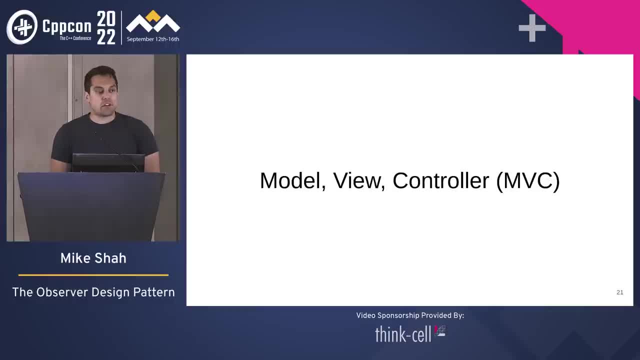 The other sort of terminology that I'd want folks to be familiar with, or where this pattern shows up. a lot is in these model view controller systems, or MVC. How many folks in the audience have heard MVC or maybe seen it built into an ID or something? 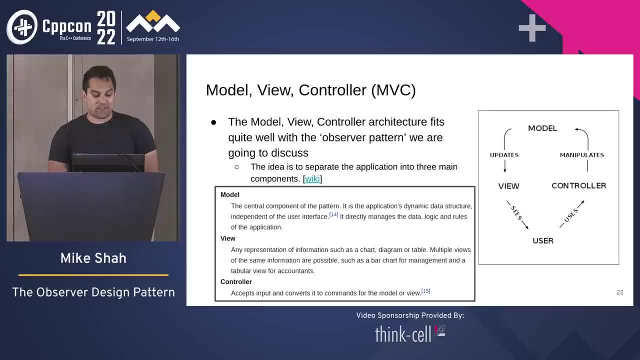 Yeah, about more than half the audience. I think you're so really quick. You know this idea, especially if you're building a graphical user application, whether it's a game or just you know some other desktop application. The idea is you have your user here and they have some controllers that could literally be some input device or maybe data being fed in your models. 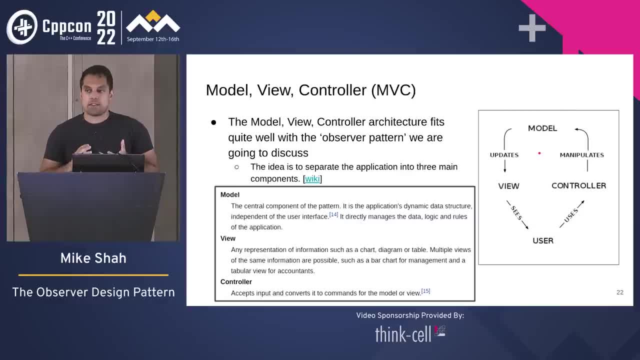 the system that sort of sets you apart: OK, OK, OK OK, has all the data structures. that takes in the actual data, the logic, the rules, processes, the inputs, and then we get the view, or update the view from that model. 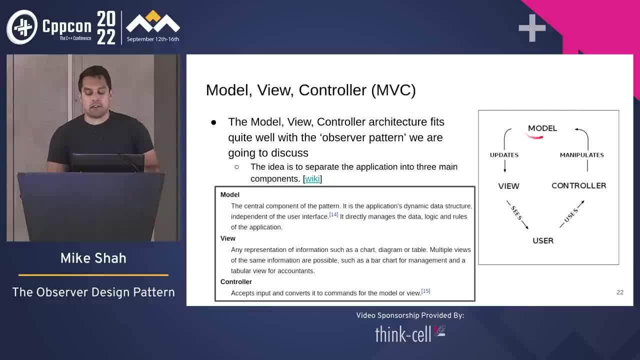 Okay, so in the case of the game, right, you may have all of your logic here, how the game plays and so on, and then the view is what you actually see on the screen, and the controller is how the user is interacting with it. All right, 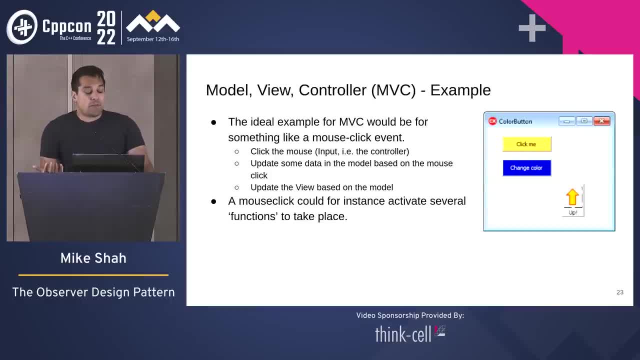 and here's just another example of it. Again, the ideal example or a simple example of MVC is: you know, you have some really simple application like this with some buttons that you can click on. That would be a good example of sort of. 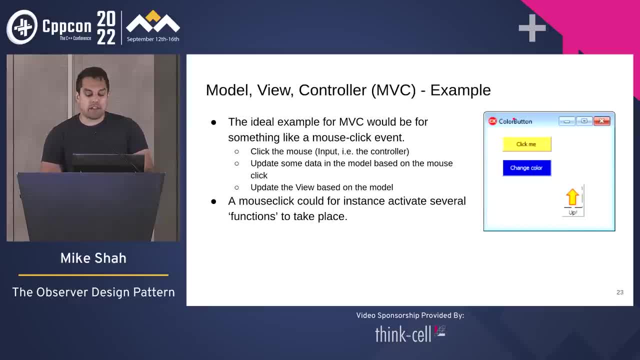 model view of controller. right. Your view is the graphical user interface. your controller, your actions are sort of clicking and then whatever business logic or whatever you want to call it behind the scenes is what happens when you click. whatever state is being changed. Now, in this particular case, even. 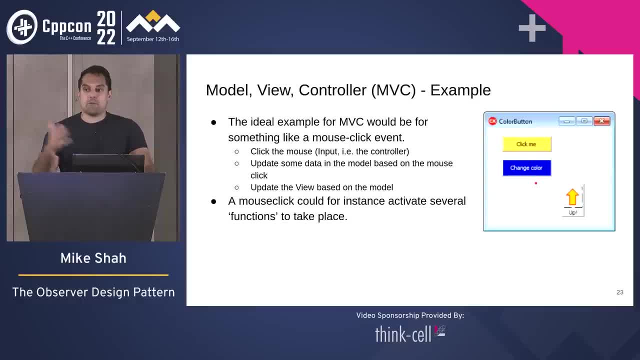 the simple one. you might click the mouse button and then some function takes place and then several actions occur. Okay, just like our Angry Birds example, where you click your mouse, drag the bird back and fire away. All right. so again, where does the observer? 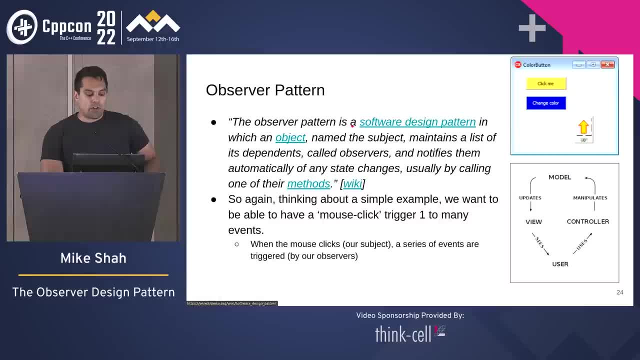 pattern fall into this. Well, the idea, or, from the the wiki, the observer pattern is the software design pattern in which an object, which we'll call a subject, maintains a list of its dependents, which are called observers, and it notifies them automatically of any state changes, usually by calling one. 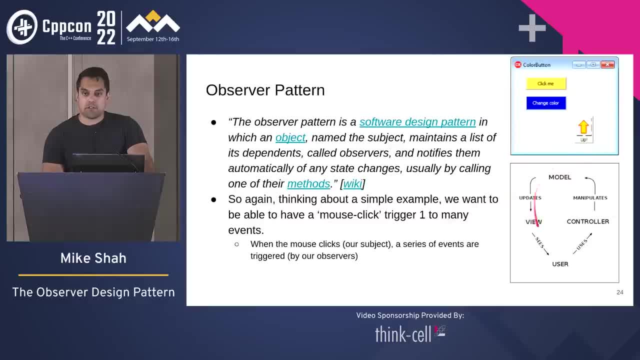 of their methods. So again you can kind of see how that fits into this model view controller mode, where you, you know, do something, some action that's affecting your actual data structure or logic, and then that change is sort of propagated outwards. okay, So again here would be the mouse click example where you have 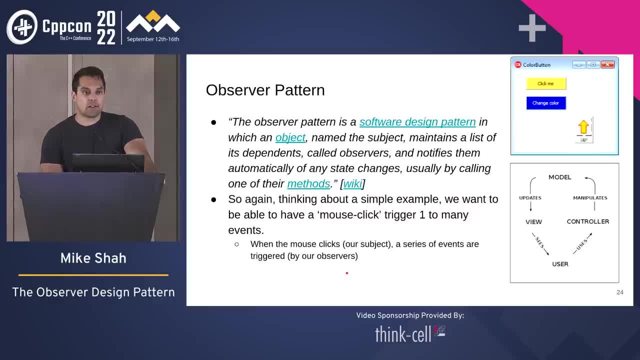 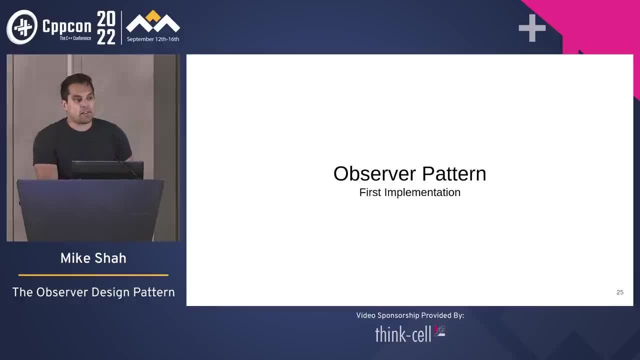 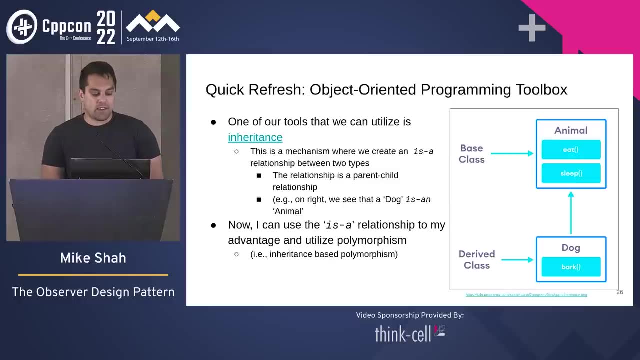 some subject that's clicked on and then a series of events are triggered. Okay, so, with that in mind, I think one way to approach learning this pattern is just to go with a very simple implementation. So let's go ahead and see what this looks like: A quick, object-oriented programming toolbox here. 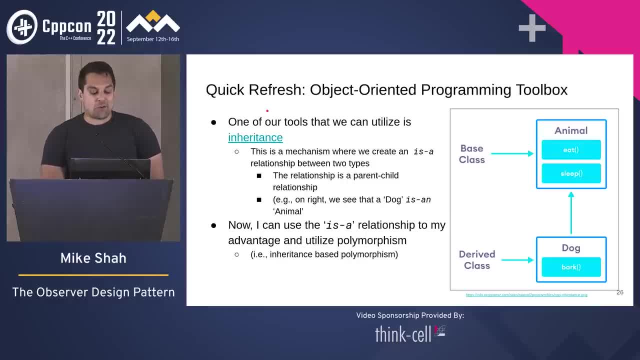 again, I think this audience will be familiar, but usually two of our tools are inheritance, which is one way to create a sort of is a relationship between two objects, right? So a dog is an animal. We're going to be making a dog. So this is an animal, and we're going to be making a dog. So here's an animal. we're going to be making an animal, we're going to be. 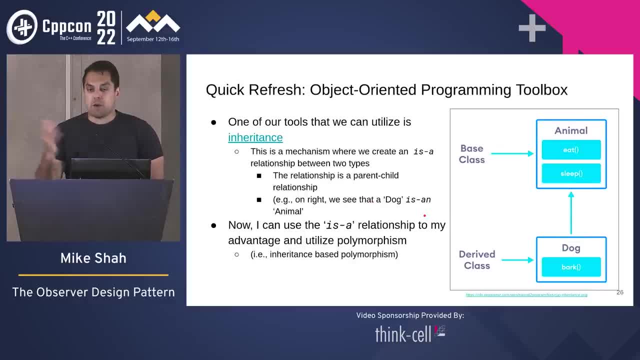 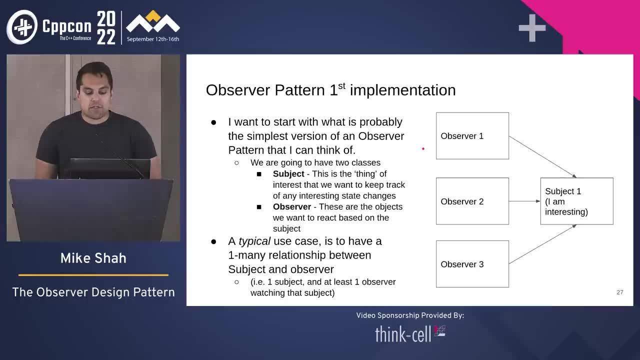 making use of this, And then, of course, you can have composition. it has a relationship, but we're gonna be using inheritance today, All right, so, with our observer pattern, the first implementation that we have, here's again what it looks like in sort of a picture. 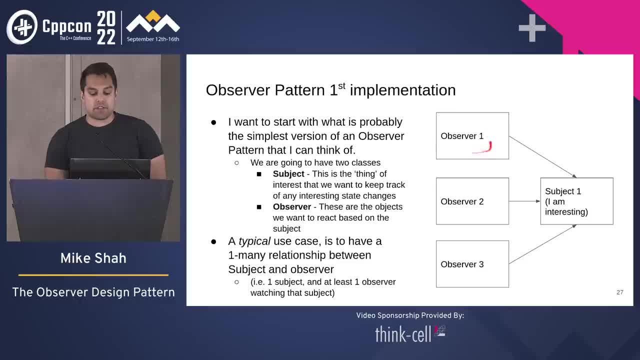 if I draw your attention to the right. So we've got our multiple observers here who are kind of keeping track of some subject, something that's interesting. Okay, so that's the idea here, And these are our sort of stakeholders in this system. 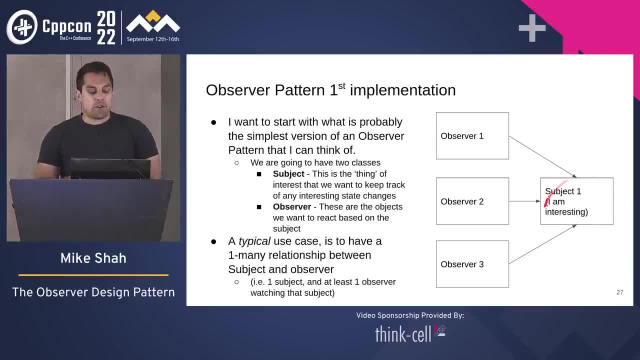 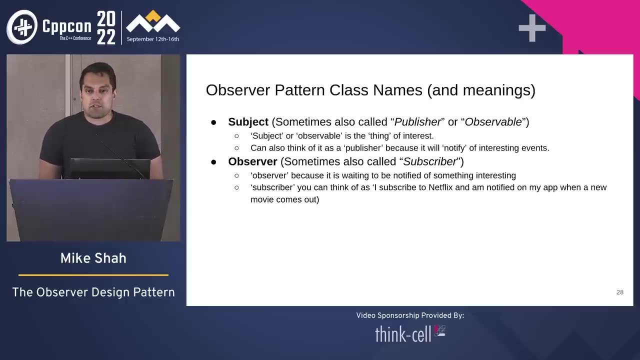 Your observers, which you could have many, and then your subject, which you usually have one. Okay, and that's typically the use case for this, where you have a one to many relationship. Something else that's also worth pointing out, because when I've seen observer taught, 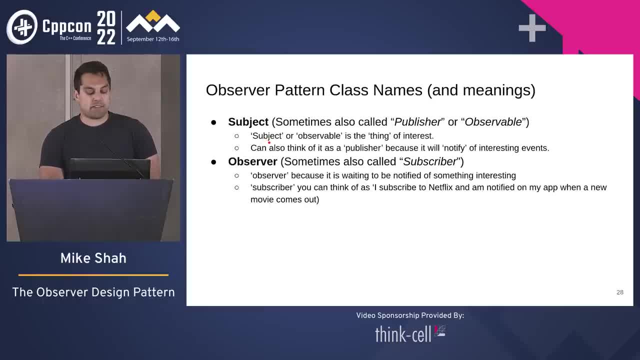 folks use different names for it And I try to be consistent in my code, but you'll hear the subject again. that's the thing of interest, Something that sometimes that's also called the publisher, or the thing that's observable, And then you have your observer. 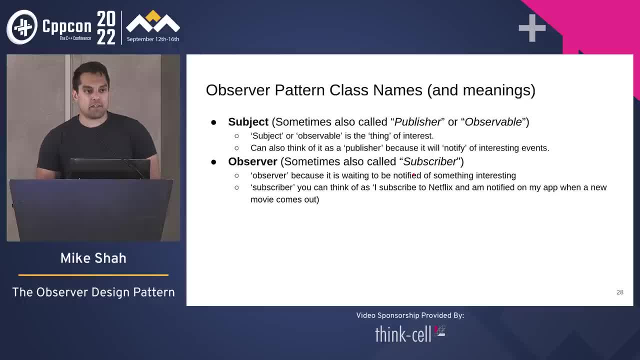 which is your subscriber. okay, And I also just like to think about this: like I subscribe to Netflix or I subscribe to Disney Plus, and there's lots of us who subscribe to those services, They can kind of just remember it that way. 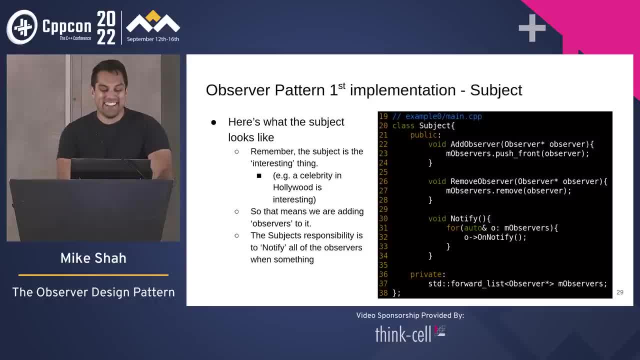 Again, I'm not commissioned for anything, All right, but let's take a look at our implementation. So here's our implementation here where we have a subject here, okay. So here would be an example of what you could have for a subject here. just a concrete class here, okay. 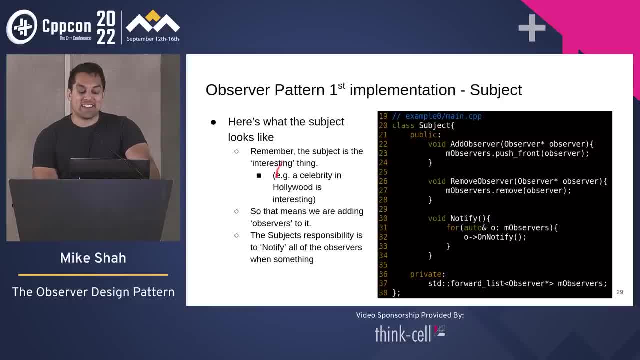 And remember this is the thing that we're interested in. So, again, if you want to remember the analogy, you could think of it like a Hollywood celebrity or something, something that's interesting and you might want to observe. So the idea, looking at this code. 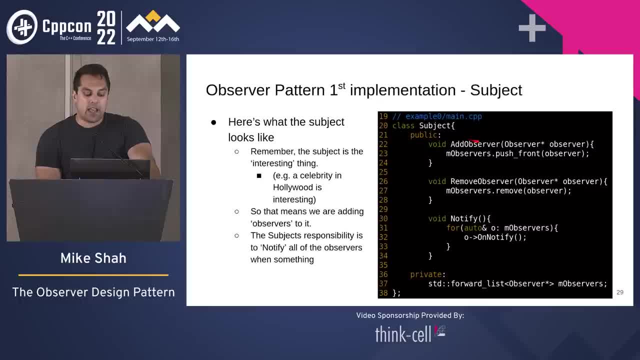 if I walk you through this again, we have this thing called subject and we have a few member functions here For adding observers. So I can add an observer to the subject that I'll be watching it. I can remove an observer as well. 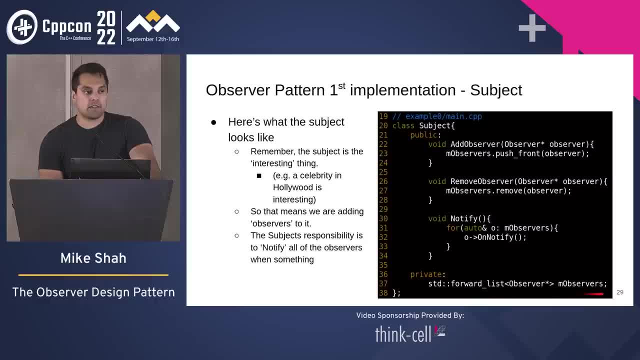 And those things, those observers, are all being kept track of in a list. okay, That's how we get this many to one relationship. okay, All these observers interested in this subject, And then the subject, once it's doing something interesting. 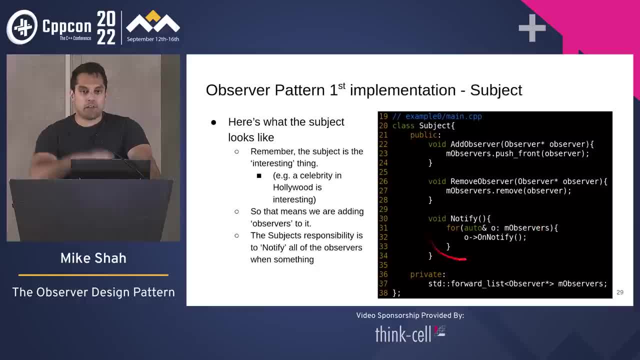 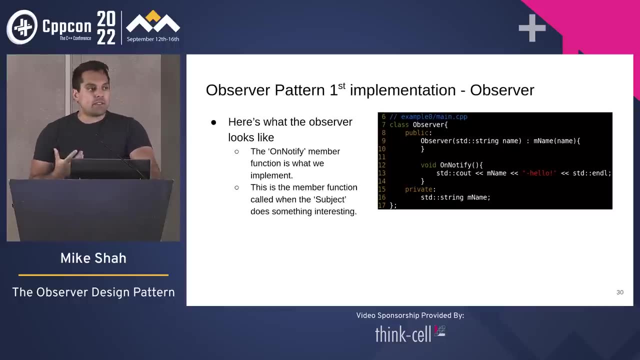 is gonna notify all of its observers. okay, So simply loop through all the observers. Maybe we call this notify all or something, but that's the idea in a traditional model, Our observer- what's this gonna do? Well, this is the thing again. 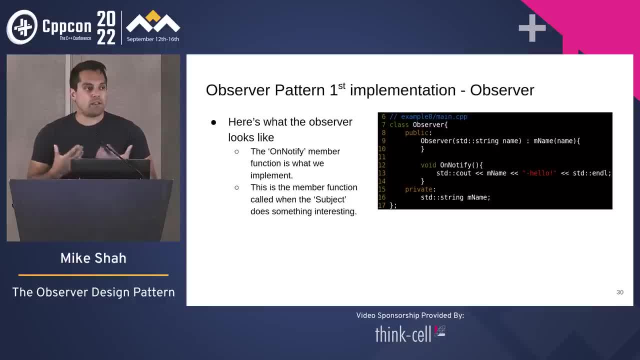 that's watching the subject. So it's kind of waiting and waiting and waiting till something interesting happens, okay, Till it's actually notified of some action. So let me go ahead and just take one step back to the subject and see that within the subject. 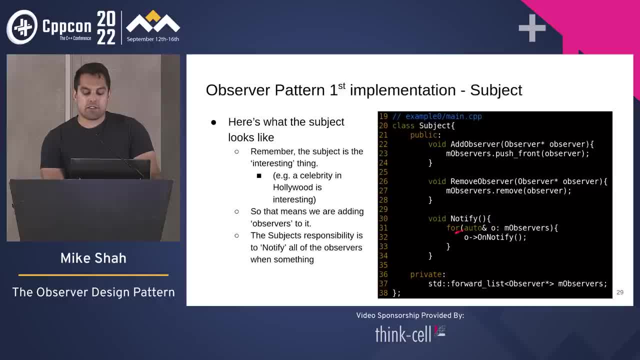 again the thing that's interesting. we're gonna say, okay, we're gonna see that within the subject- again the thing that's interesting. we're gonna say: okay for all of our observers. call this onNotify member function. 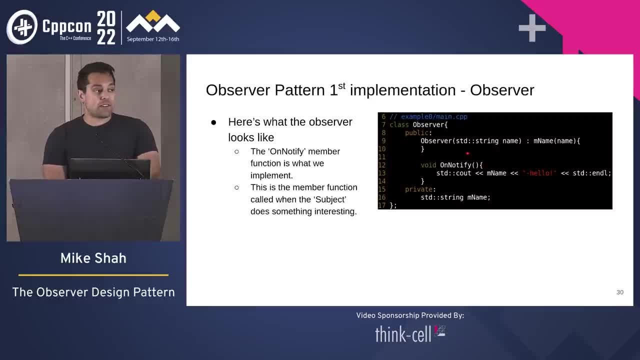 Okay. so back to our observer. you'll see that the really only interesting thing that it's doing, or the only work, is onNotify here. okay, So that's the action that's gonna be performed. And again, you can imagine this in our Angry Birds example. 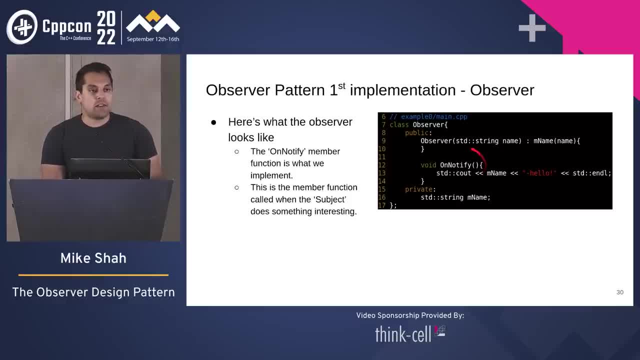 which I'll keep referring to and we'll build off of. This is where you would increase the score if you're in the scoring system, or do a collision if you're in the collision system, and so on. Okay, this is where the interesting work happens. 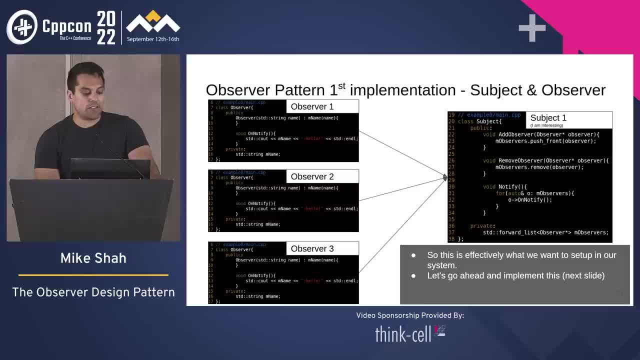 All right. so here's just another way to visualize it again with this many to one relationship. Again, we can have these observers here, they're these concrete classes and they're all looking at this subject, okay, And they're stored in some list data structure here. 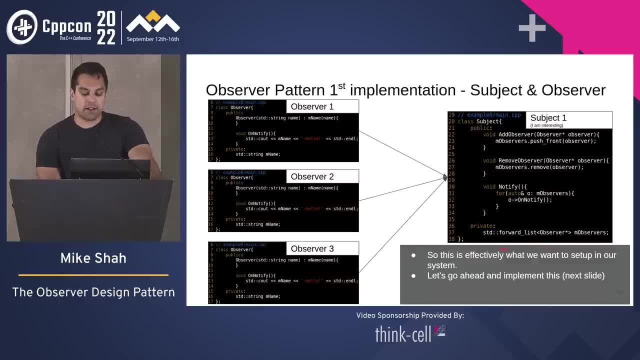 Again, you can use different types of data structures here. I'll talk about the trade-offs later, but that's the idea. So before I go ahead and run this, let me pause for questions. Let's see if folks are okay with this. much so far. 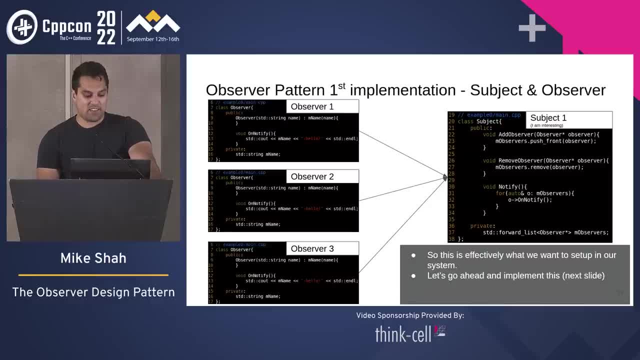 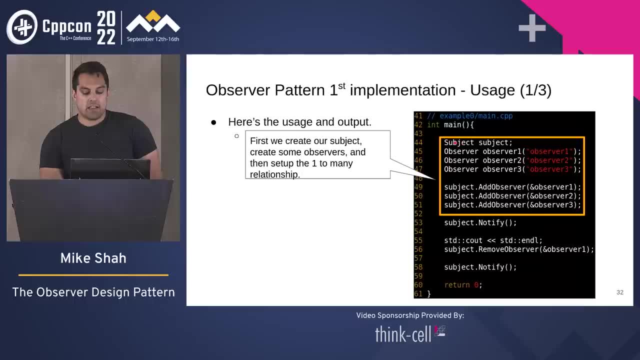 So far, so good. Awesome, All right. so the actual usage for this code. let's say we have our subject here and then we're gonna have the three observers that we create. I'm giving them names here again, just so we can kind of have some interesting output. 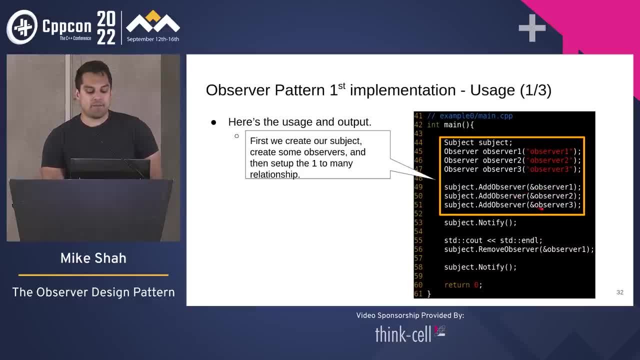 And then for our subject, we add all of these individual observers. okay, And then when we want to do something interesting, or something interesting happens again, you could imagine in your code the user. you know, maybe you have some LogicCaresas. 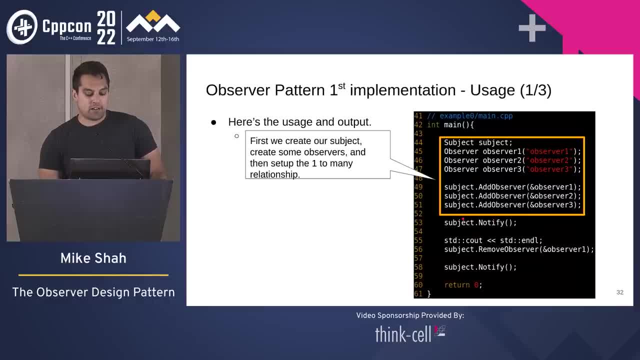 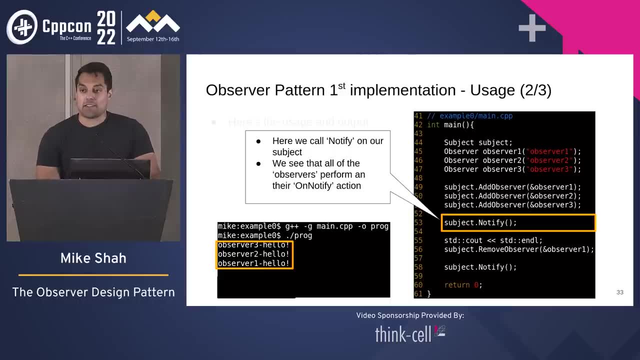 if mouse clicked, then you know, notify the subject or call subjectNotify, And then again notifies, iterating through all the observers and calling that onNotify function which, in this case, our observers are just printing out. hello, okay, That was the interesting work that they needed to do. 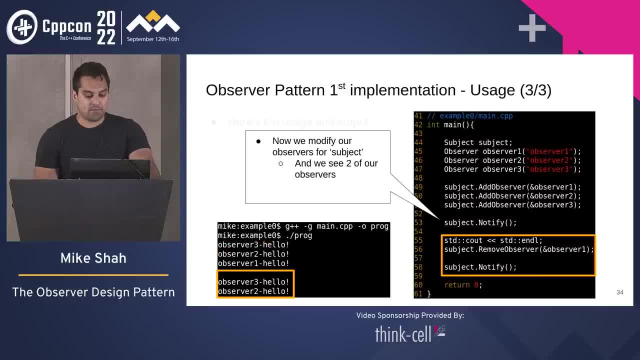 or the system that was invoked, All right, and of course we can unsubscribe to some service. So in this case, of course we can unsubscribe to some service. So in this case, In this case, when I continue forward with this program, I call subjectremoveObserver. 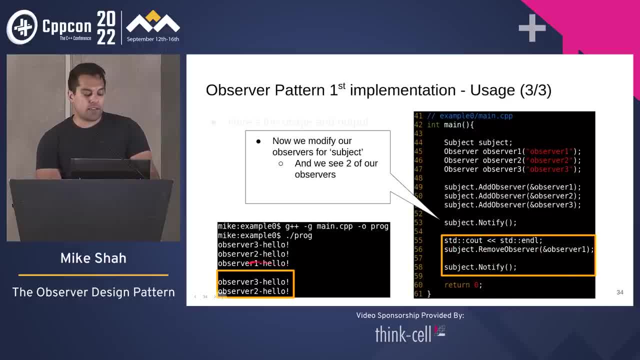 I get rid of this one and then now when I call notify, you'll notice on the output on the bottom left here I've lost observer one. okay, and they can be cleaned up or whatever, but they're gone. They're no longer subscribed to whatever service. 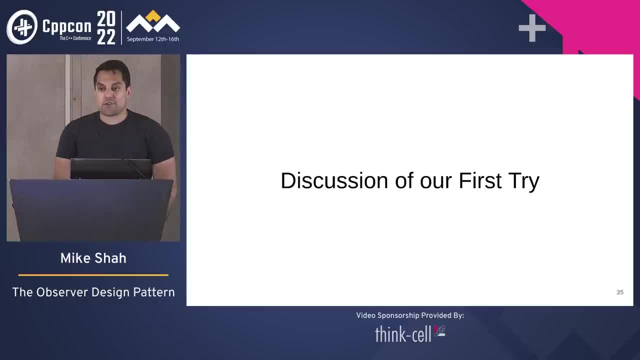 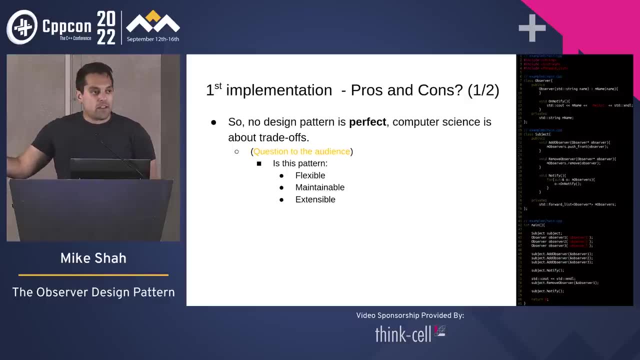 All right. So let's kind of discuss this. first try here on our observer pattern, and again I said no pattern's perfect, but this is sort of again a one-to-many, I think, sort of pattern. but what do folks in the audience think about this? 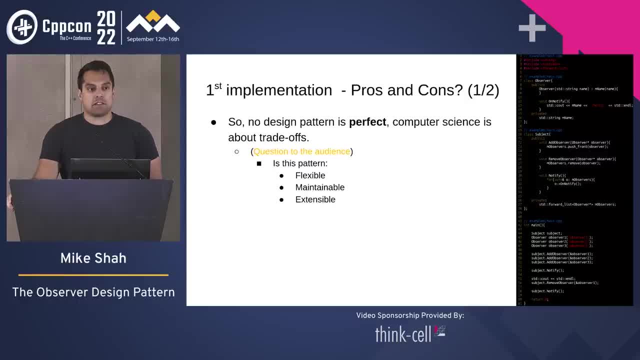 Was this flexible, maintainable, extensible? What do folks think? Any thoughts? Dangling pointers? potentially Okay. So yeah, we do have to think about that and I will clean that up, don't worry. but yeah, like okay. 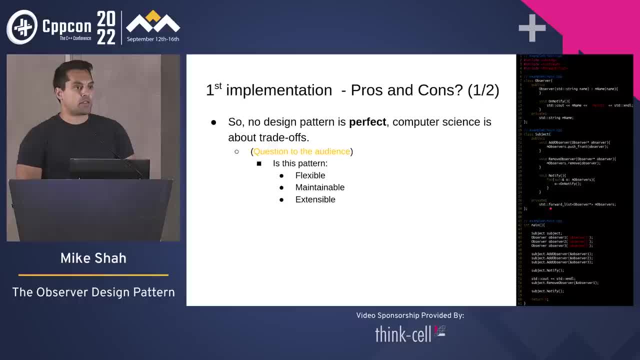 Let's be careful with removeObserver and some of these functions. Let's assume we did it correct, but it is a danger. Was there another thought? Yeah, We're going to have to think carefully about this too, and that's where I will actually. 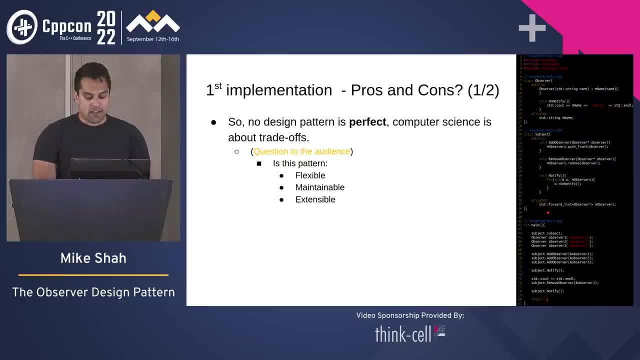 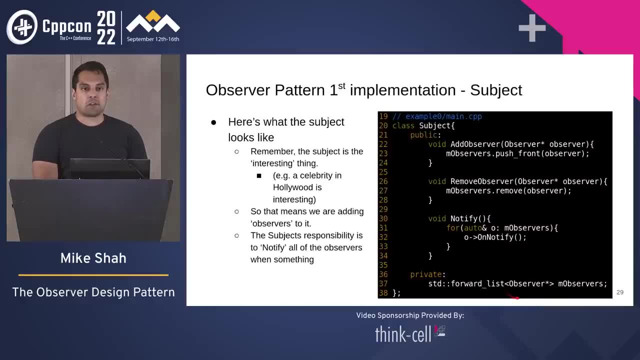 wrap up, depending on what our actual data structure is. so if I wind back a little bit just to keep everybody in the loop here, we have this raw pointer here and we're going to fix this right. We're going to have a modern C++ conference here later on, but we do have to think about 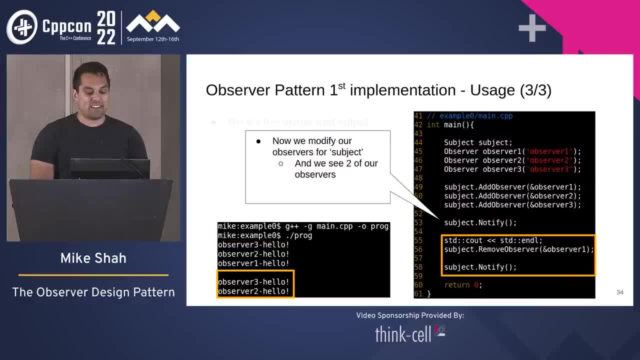 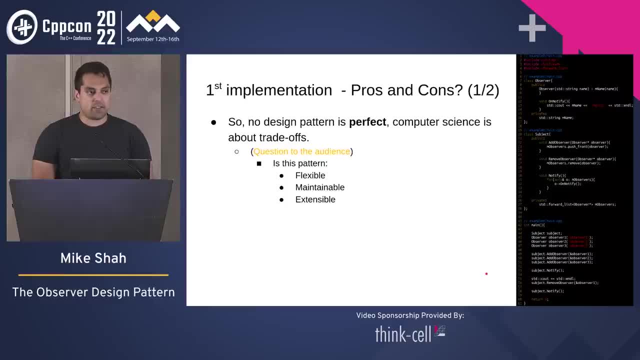 ownership, certainly okay. So I mean we could probably come up with some abstractions to kind of fix this. but yeah, just in thinking about this, you know, what I have so far for our criteria is: is this flexible? 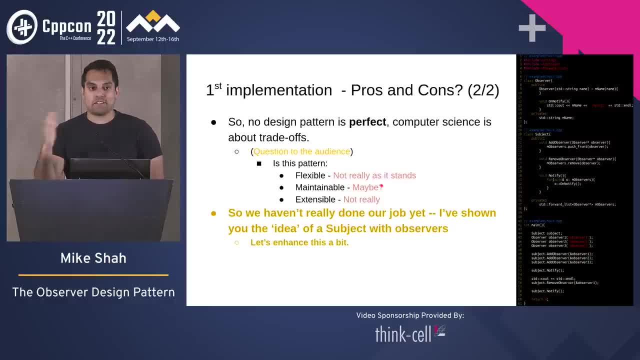 Well, not really as it stands right. We're creating a lot of concrete classes to kind of have these observers in our subject. Is it maintainable, Maybe right? Some folks have kind of come up with some issues about maybe ownership and some of these. 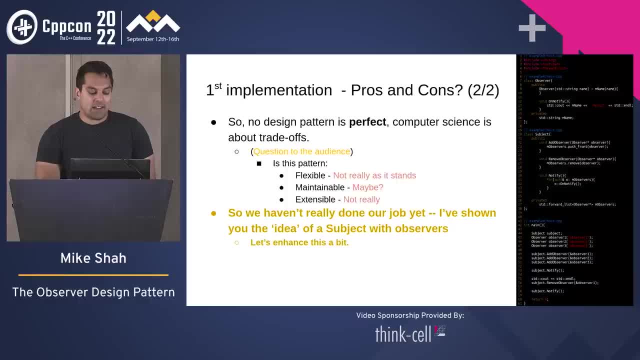 things. We're still writing individual code. Is it extensible? Not really, right. I gave us some of our tools for extending things meaning inheritance or you know some way to build off these data structures. so we don't really have that yet, but you. 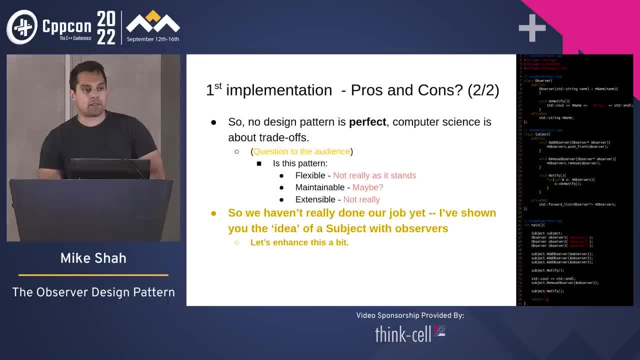 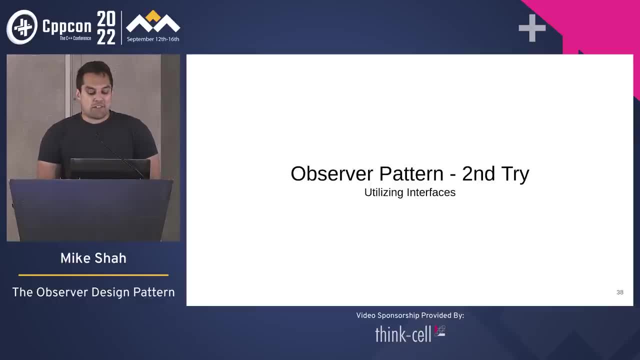 know, I think this is probably the most basic version of an observer that we can get. okay, So let's enhance this a little bit, All right, So let's try this in round two here and actually utilize an interface right, Utilize some of our object-oriented tools. 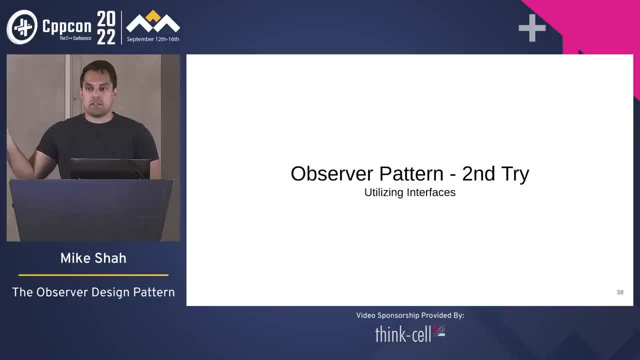 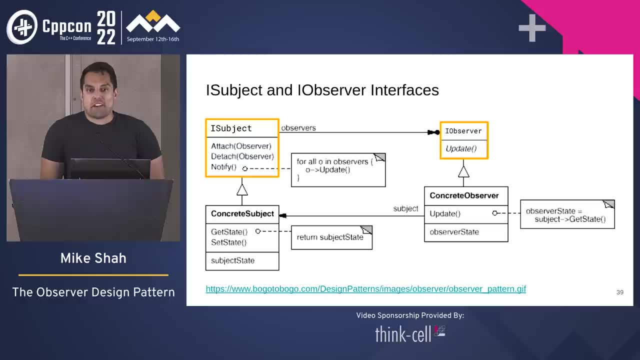 Now what I will say is: you don't have to use inheritance. You could do this using composition or other things, but inheritance is kind of a nice way to show this off. Of course, I've got to give you a classic UML diagram so I can understand this. 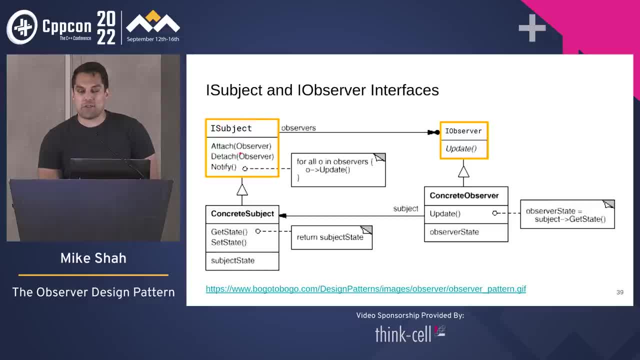 I've kind of highlighted the important part, or what we're going to do with our observer pattern here. That's it. So we're going to have this interface here. so our classes that start with I are usually abstract classes or interfaces- ISubject and IObserver- and then we can actually derive. 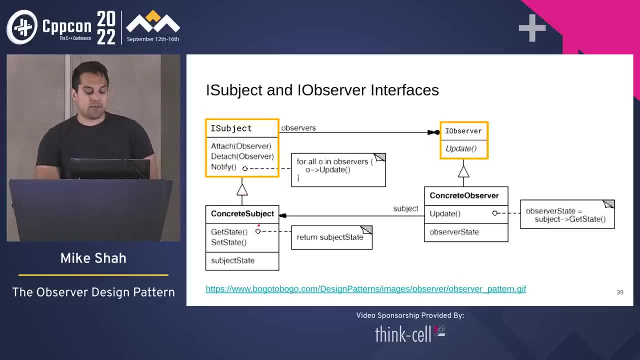 some concrete classes from those, okay. So we'll have an actual concrete subject and actual concrete observers, or maybe multiple of them. okay, But then we can kind of build some more interesting. you know, have a subject that can have different types of observers seeing what's going on. 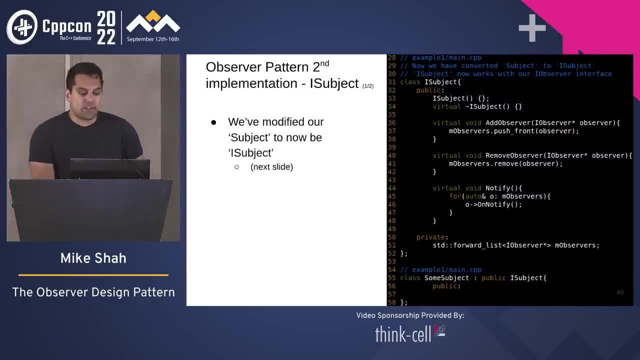 All right, All right. So here's some of the modifications that have been made, and I've kind of extended this out a little bit. So I've modified our subject to be an interface in this case. okay, So the main takeaway- and I'll kind of walk you through this code is right. we have. 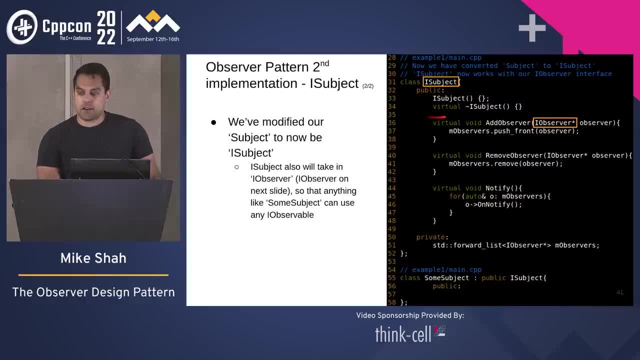 our class ISubject, which is going to serve as an interface. so again you'll start seeing virtual showing up here and when we're adding observers, we're doing this, we're adding, we're adding an interface to our observer here. okay, 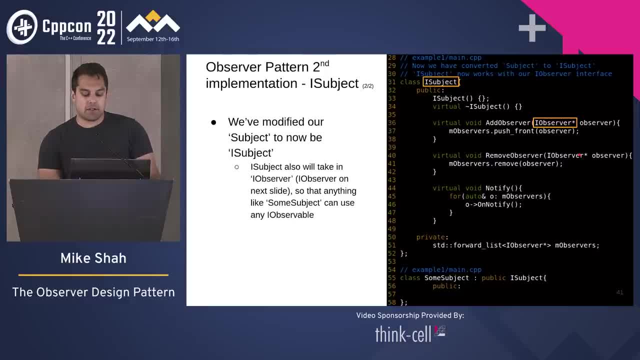 So you'll see. wherever we had a concrete class, it's been replaced with this interface. okay, Same here down in our forward list. here we're getting a forward list of anything that can be an interface to an observer. all right, All right. 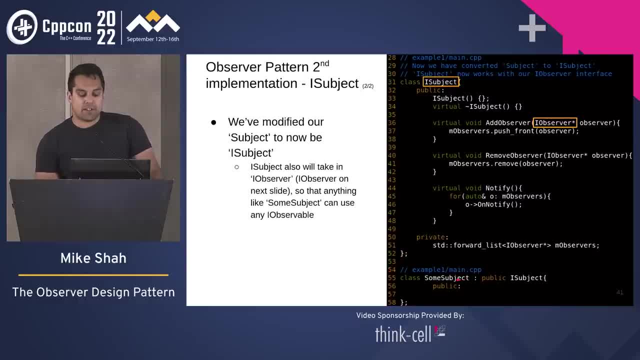 And then at the very bottom here you'll see we have a subject- and I just call it some subject, right? Anything that's interesting that you might want to check out, That's going to be inheriting from a subject here, this interface. okay. 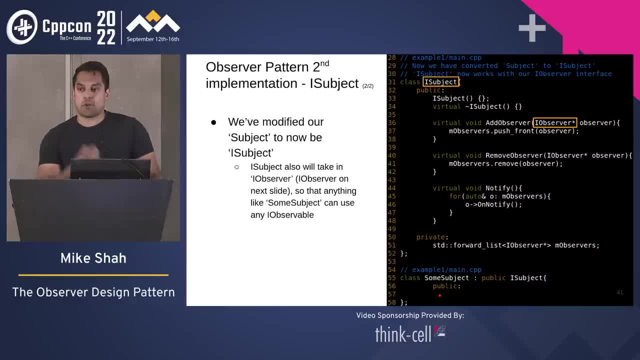 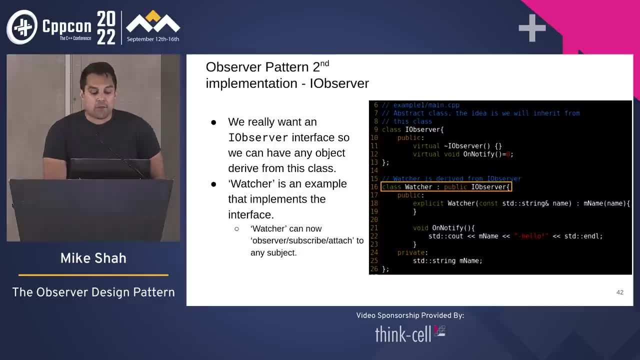 So this thing here can have subscribers subscribe to it or observers observe it- okay, depending on what terminology you want to use. All right, So for our observer again, we want to have this interface here so that we can have sort of different types of observers subscribing to some subject. okay, 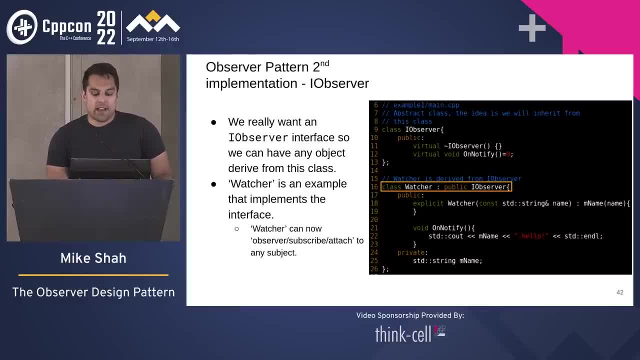 Different things watching or different systems watching. So in this example I have our interface to observer, but I've made this a pretty much an abstract class here. Again, I wish we had interfaces, but again pure virtual function here on notify that. 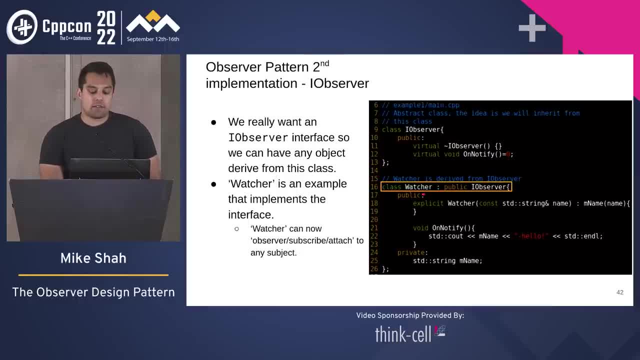 we have to implement. And then, as far as making use of this, I have watcher here which is deriving from our interface. okay, So watcher is going to be our observer, okay, As it's named, And then, on, notify is where we're going to put any of the interesting work that we want. 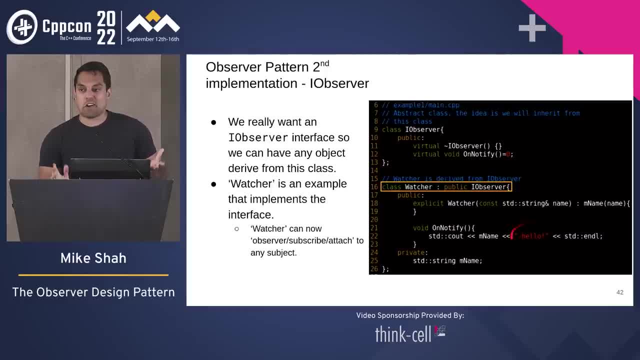 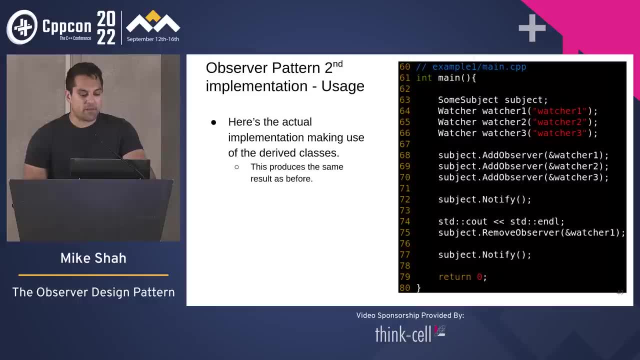 a watcher to do. In this case it's going to print: you know its name and then hello in this case, All right. So let's go ahead and move forward from here And we'll see our second implementation here for the usage. okay. 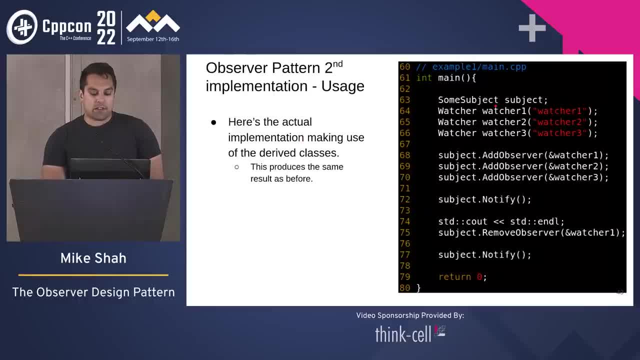 So here's the actual implementation. If you actually look at this code, pretty much nothing's changed, other than I've changed some of the names here to actually use our deriving. So I have some subject- which was the thing that we're interested in, watcher- which is: 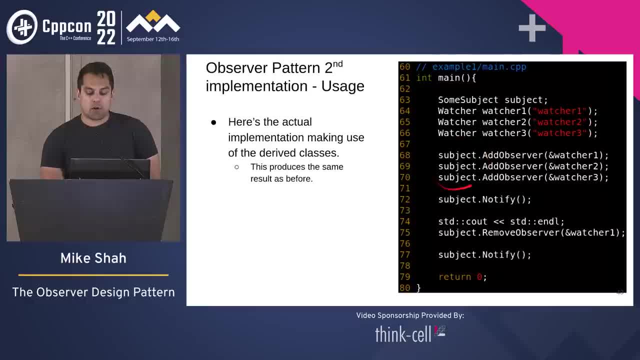 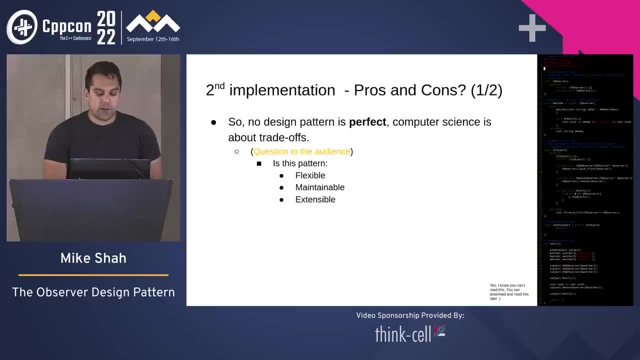 one of our observer types here, and then I'm performing this code here. Okay, So it's going to do the exact same thing as before, All right. So thinking about this- and again, I don't expect you to write the code or to read this- 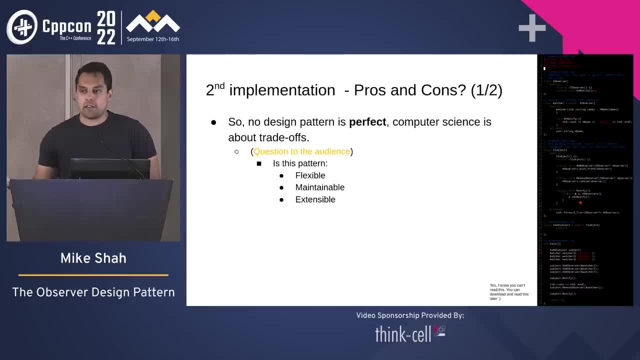 code on the right, but you know it's grown a little bit longer. We've added some interfaces in our code. What do folks think about this one? Are we getting more flexible, maintainable and extensible in this manner? 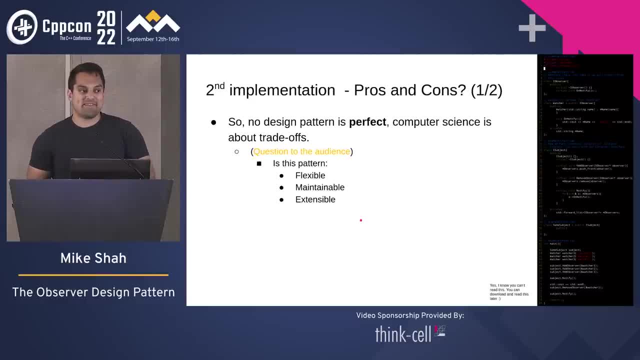 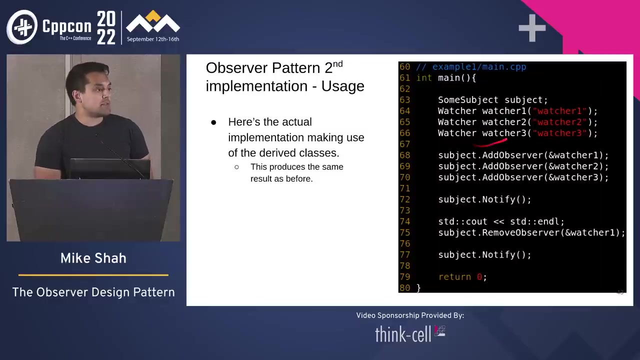 What are folks' thoughts? The question was: if I'm an observer, so in this case this watcher here you're saying, then I have to. I do have to create in this model. I have to model a class or this object here. 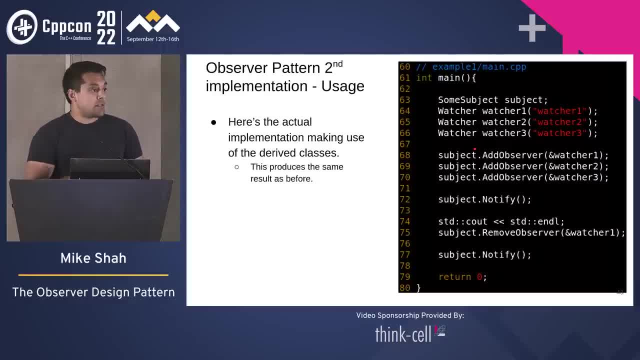 Now, what I will mention at the end is: these don't have to be objects, right. These could be functions or some sort of event that you want to fire off, All right, And we have another. The terminology I usually see is maybe like a listener or listener event, for example. 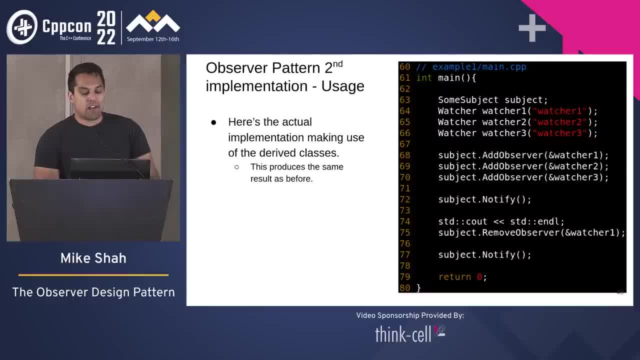 That would be another way to model it. I'm going to do it all with objects, but I could just have this subject take in a std function or something. Well, what I mean is like right now, if your example is: 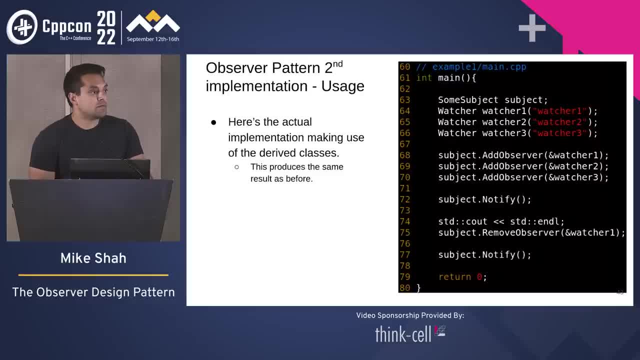 Okay If you have one subject, but what if you were interested in two different subjects? Got it Okay? Yeah, So the question was: let's say, I have two subjects here and I want this watcher to be watching two subjects. So, as it's modeled right now- since it's just a pointer- I could have both of them subscribe. 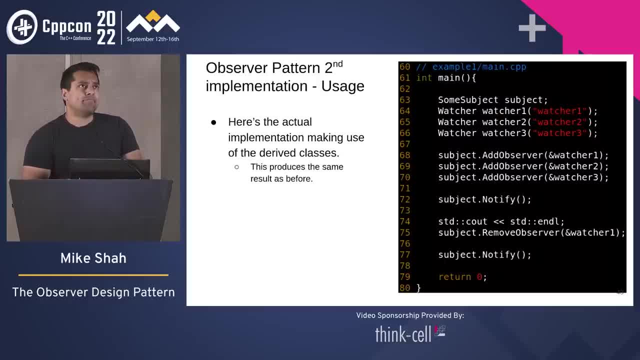 to that. I'm trying to think of what the analogy would be. It'd sort of be like again if you had two Netflix accounts For yourself and a friend, And then you have a buddy who really likes watching, that have both accounts on your profile. 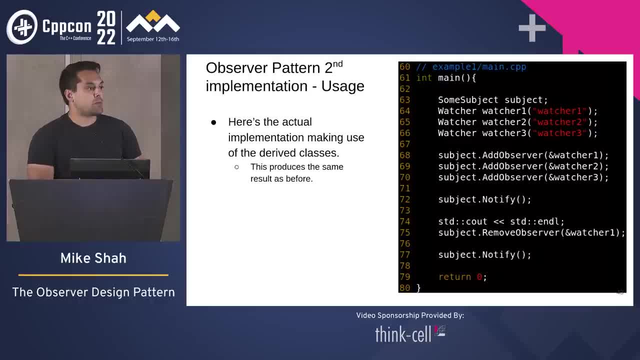 Right, So the same thing's allowed here. You could be subscribed to multiple things. Now, whether we want that or not depends on, again, how strict we want our observer to be. As someone mentioned, we do have to think about ownership. 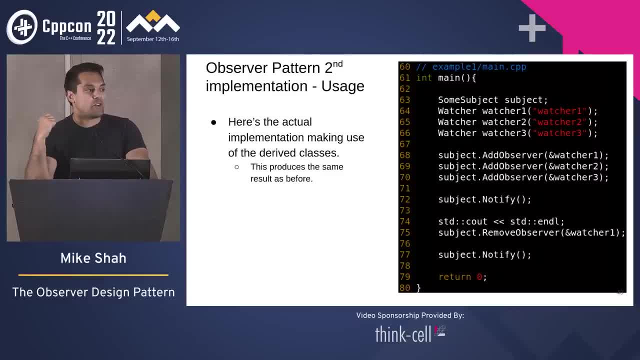 So maybe we'd want to move that pointer, Maybe not. I'm going to show you a smart pointer later. All right, Yeah, Yeah. The question is: yeah, notify doesn't carry any state right now. Yeah, That's correct. 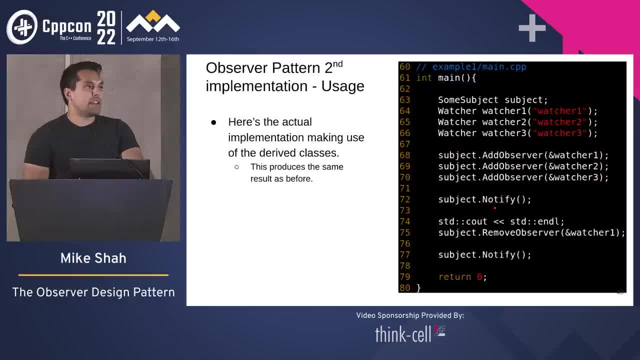 Yeah For this example. But we could pass state or have state in some sort of subsystem here. Yeah, Yep. Another question: Yep, Yeah, Yeah. So the follow-up comment was: if we had just a std function or something that we were. 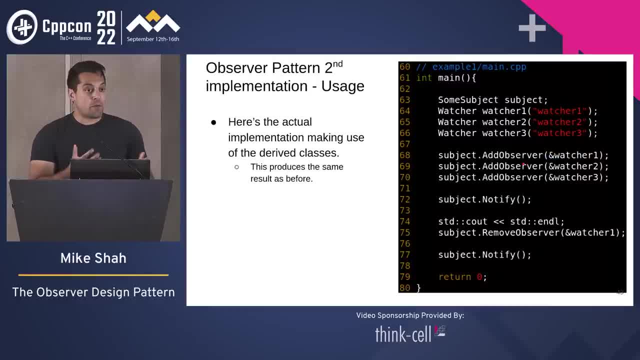 taking in here, I guess maybe to summarize it, I mean we get some flexibility. So I mean we can kind of think about this in the Angry Birds example, Right, So if we have a- I don't know- a scoring system or something that we don't really need to, 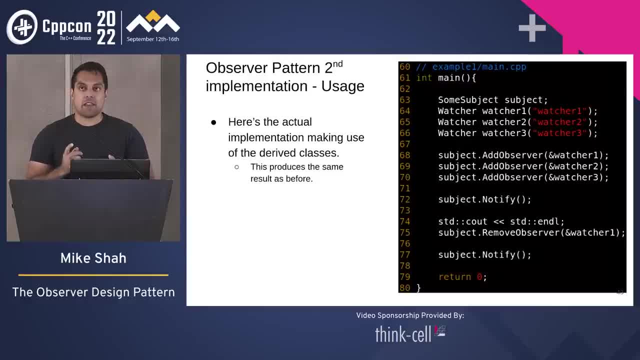 create another object for, maybe, Or a logger, where we just want to print out events to some log or something. We probably don't need to create a whole object for that, Right, Just call some function that writes out text, Right, So we can model this in flexible ways. 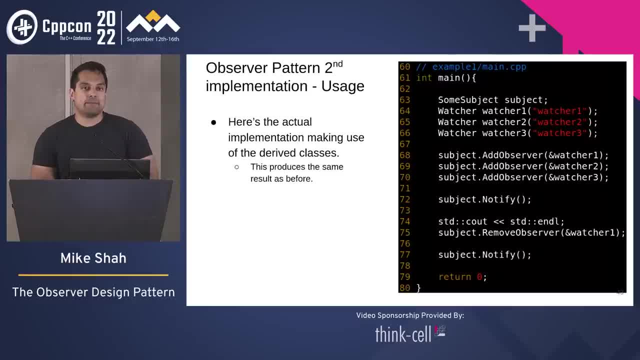 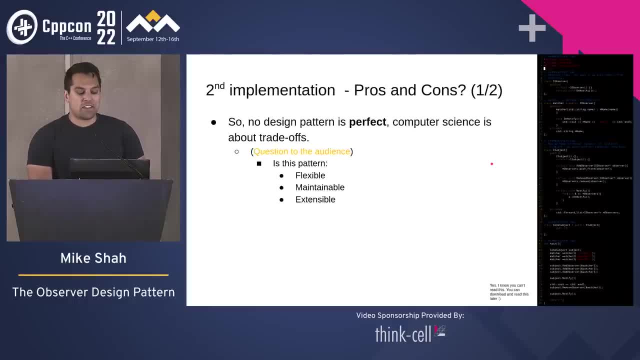 There's a lot of different types of observers that we could add to this subject, Right, So I think so. I think what I'm getting from this- Based off of the questions, since we're getting some more trade offs or sort of implementation details that we could add to this observer- is, I think we are doing better on this flexibility. 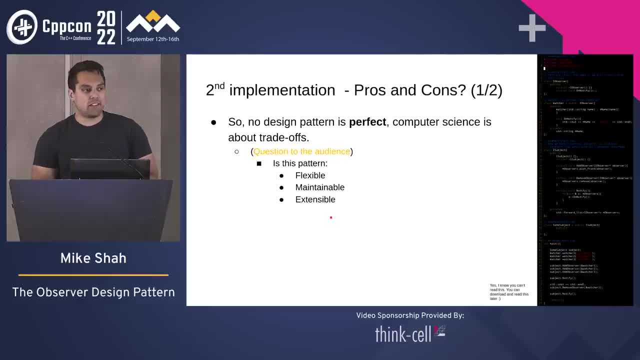 maintainability and extensibility. At least we're thinking about these things. now Let me show you what I I want the answer to be, I guess, Flexible. well, I think we do need some more power here. I don't think we're quite there. 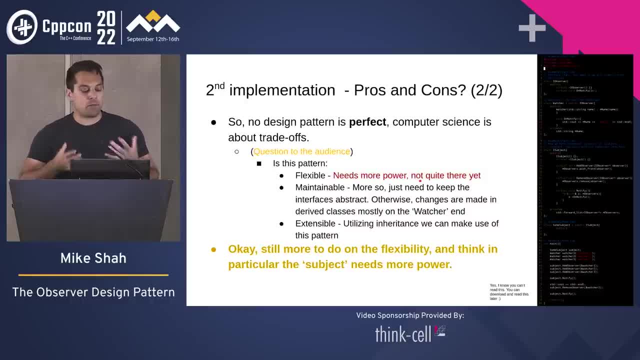 yet, And folks are even mentioning things like: yeah, what if you just wanted a function that might be more lightweight, instead of having these objects and ownership to worry about? I agree, I think that would be another progression here. Is this maintainable? More so, I would argue. 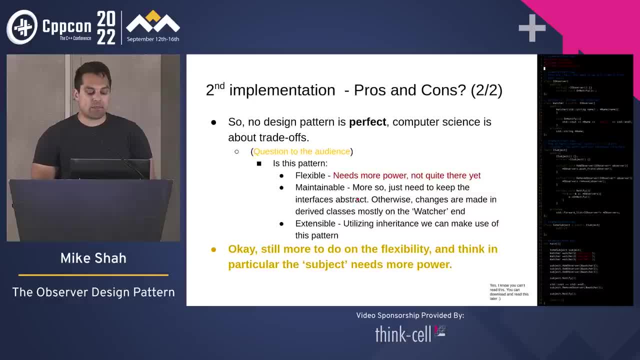 Once you have your interfaces sort of in place, then you know the actual changes that are occurring are in concrete classes, right? Your users are implementing some specifications, some blueprint that they're following. I think that's a good thing. There's other things you 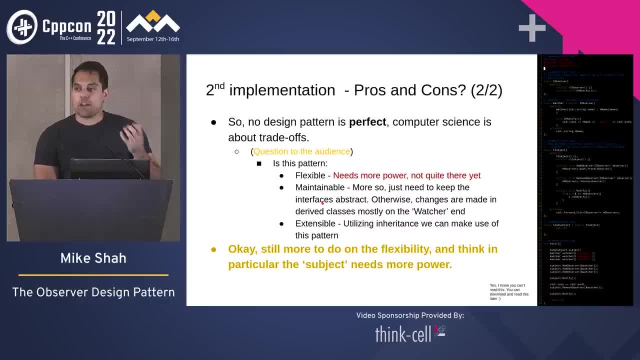 could add to this, to make it more maintainable, Various idioms and so on, And then I would say this is extensible. We're inheriting from some base class to extend, have different observers. I'm fairly confident of that, that we have at least extended this. 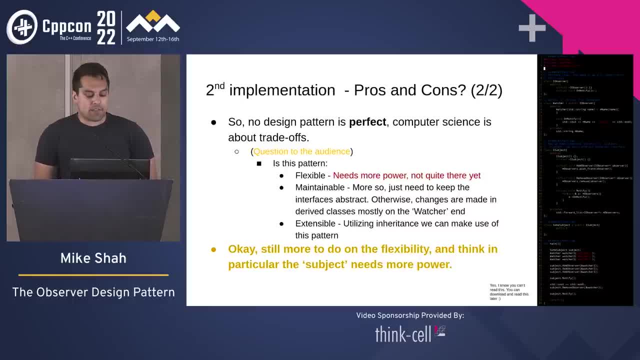 But I don't think I'm quite happy with this. I don't know if other folks are quite happy with this. We want to add a little bit more power yet again, Or at least maybe improve the efficiency on this pattern. All right, So let's do a third round. Third round of our observer pattern. This: 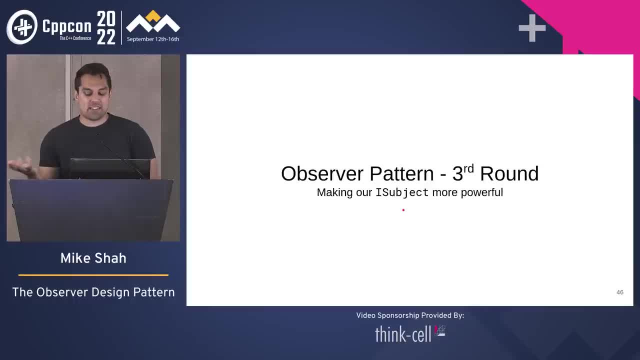 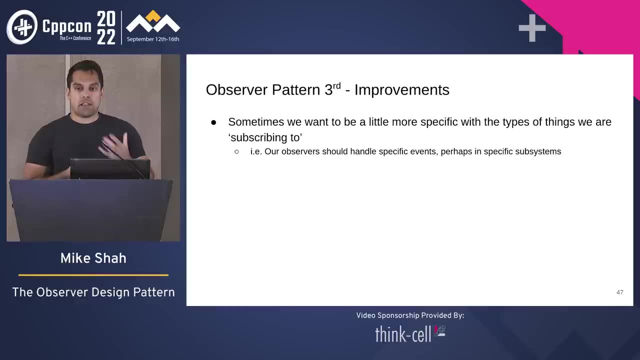 time we're going to make the subject more powerful and, I think, get to something that looks more like an observer That we might have, And in this case we want to be a little bit more specific with the types of things that we're subscribing to. So someone mentioned that there wasn't really any state or 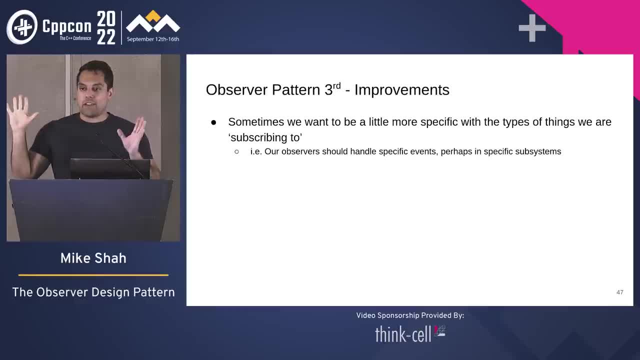 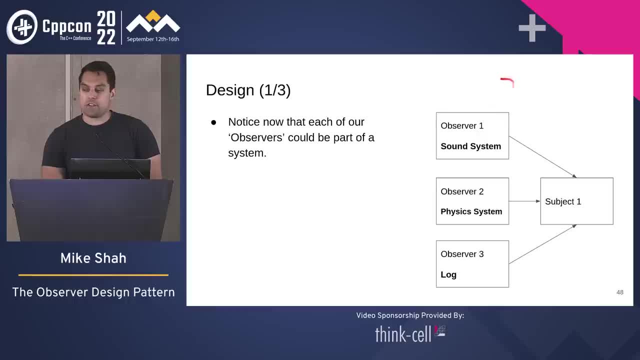 attention to the right. we have this sort of same picture at a high level if you just look at the boxes Right. Multiple observers, One to many relationship here, One subject to many observers, But this time I want my observers to be part of specific systems. 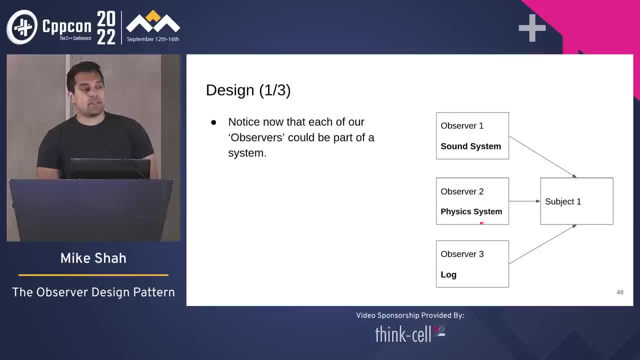 Maybe one is part of the sound system, One is part of the physics systems, One a loger, Animation, collision, Whatever other. you know the systems we mentioned to start. So kind of moving this forward here. we want something that looks a little bit more like this: 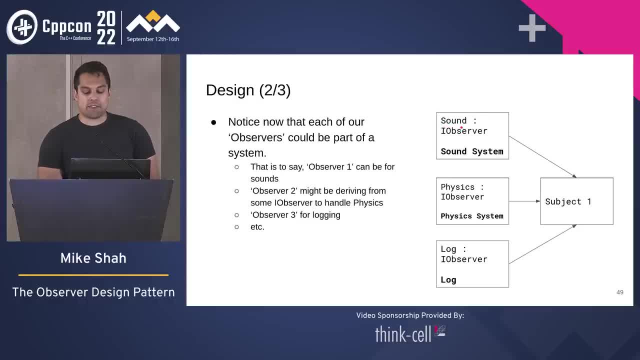 right where we have our sound class, some concrete class that we can make That's derived from an eye, observer, this interface, same thing for physics, same thing for log. Okay, so we're actually going to derive some new classes here that could do something interesting Now. 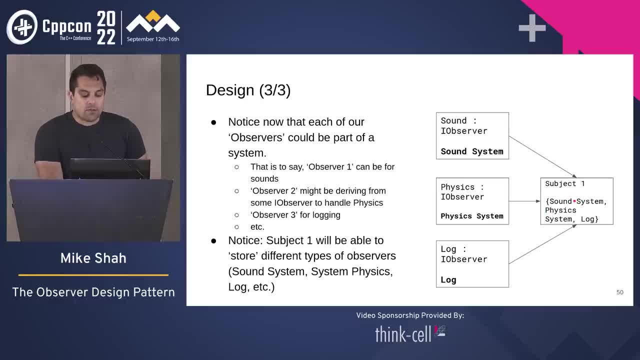 for our subject here. I want our subject to be able to store or maybe handle these different observers in different ways. Or maybe, if I have a bunch of sounds that need to be played but I don't need to do anything with physics, maybe there's some way I can just look at. 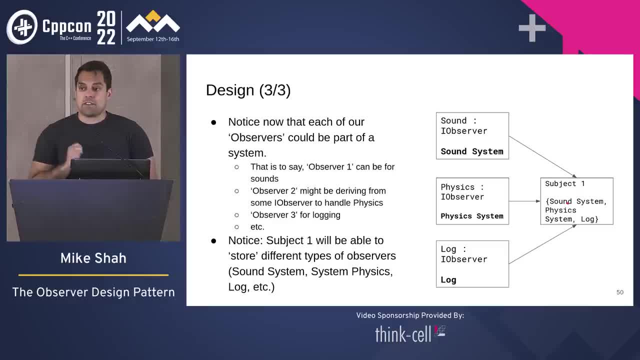 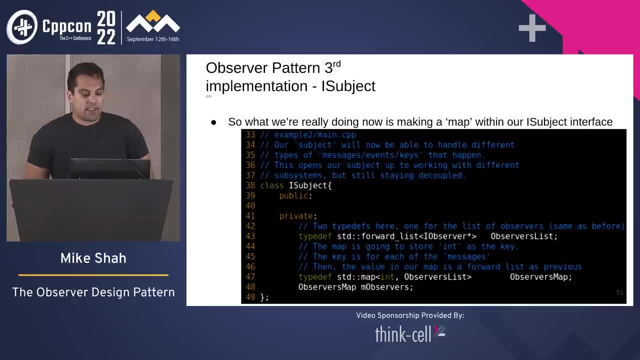 notifying the sound system that interesting things happened. Okay, Alright, so let's advance this design a little bit, And here's where we'll start with our actual interface. here And again, there can be multiple ways to do this, But what I've got for 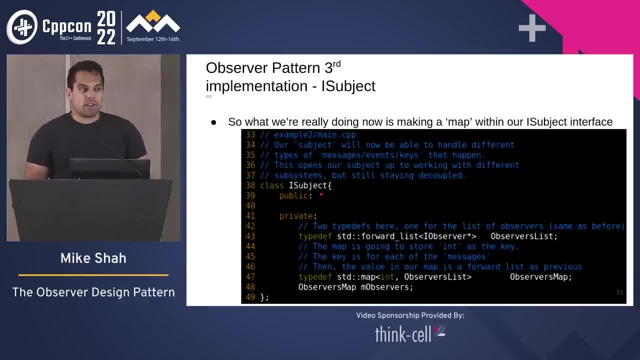 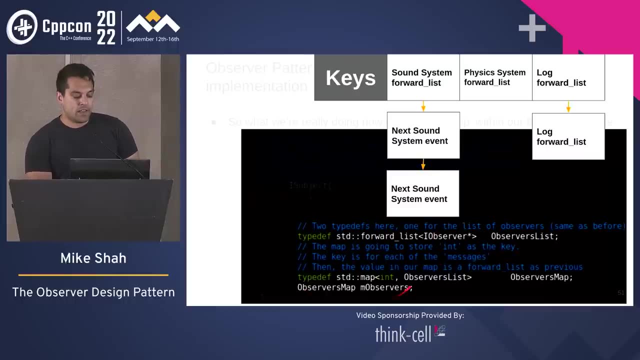 our interface here is: I really want a map that can handle the different types of events for a particular subject. Okay, And again we'll have something that looks like this. I'll kind of highlight it at the bottom: Here's the code here. So the real important thing is just this last line. 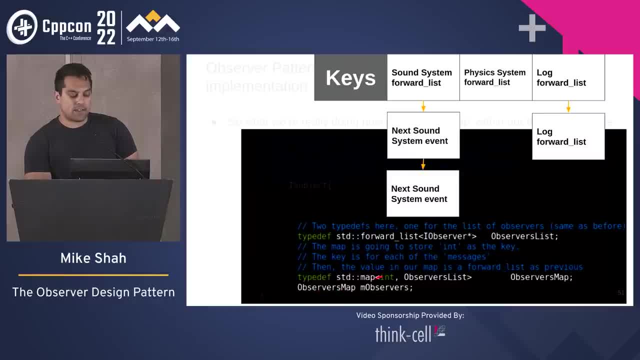 here that says we have this observer's map. Okay, so basically that's going to consist of some key, which, for now, is going to be an integer and a list. Okay, and here's what the actual visual data structure looks like. All right, 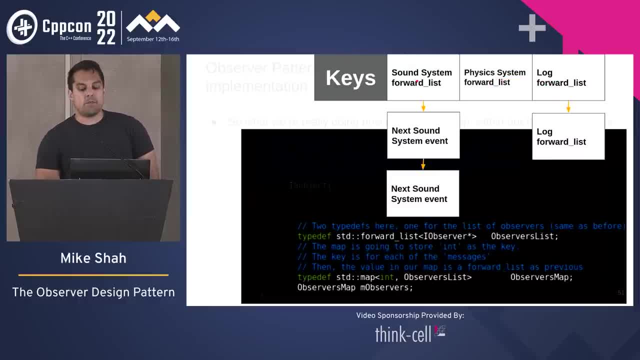 we have these different keys, So messages that are part of the sound system, messages part of the physics system, messages part of the logs. Okay, so that's what it looks like And then maybe within you know each of these keys. this is our forward list. Now we could have you know. 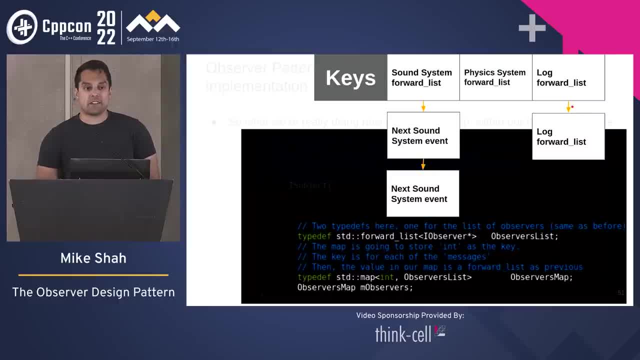 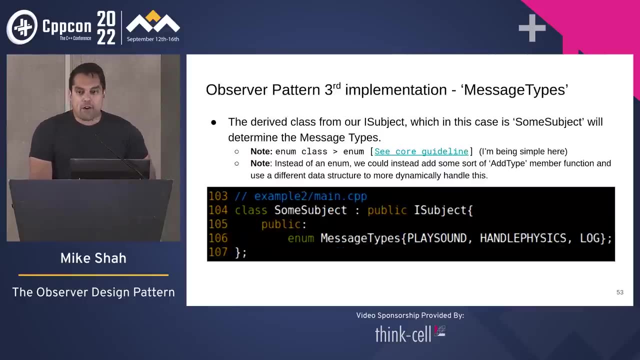 three sounds here, one physics thing and two messages logged. Okay, so that's the idea or the interface for subject. All right, So now how to sort of work with this. different subsystems here, the different message types, Okay, so how do I organize this so I know something's part of? 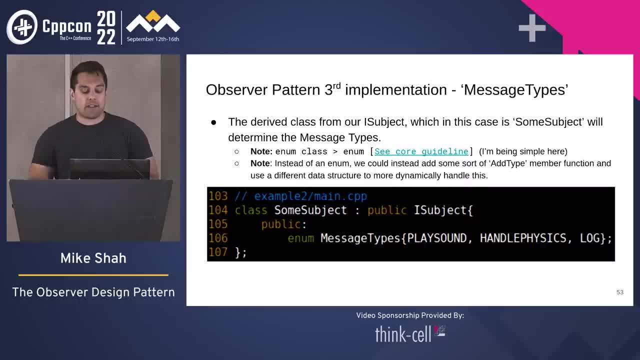 physics, part of sound, part of the log system, or as many else that we have. Well, here's one way to do it And again, I'm going to do things as cheap as possible And I'll C++-ify it in a moment here with some newer things. 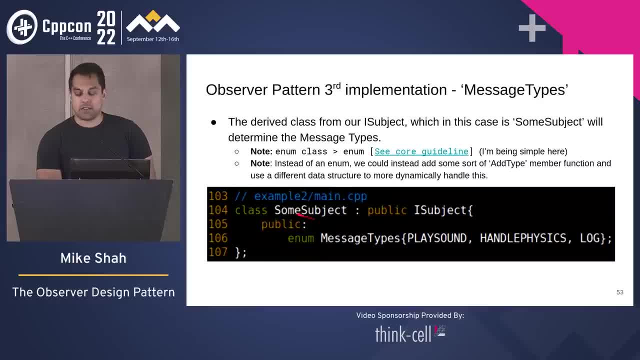 But just taking a look at the code here, right, here's our concrete class for some subject. Again, it's interface for the subject, But here's the different types of messages that it can handle. Okay, so I just kind of embedded these here, this enum, here. 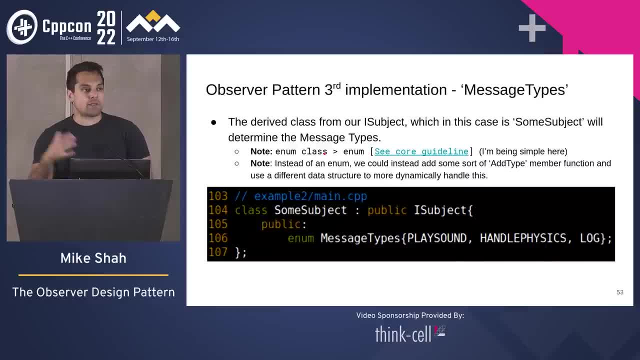 Now I am going to improve this. Don't worry, We'll have an enum class and we can have some type safety for our users. But again, the idea is that we just want to be able to identify. okay, this is you know. 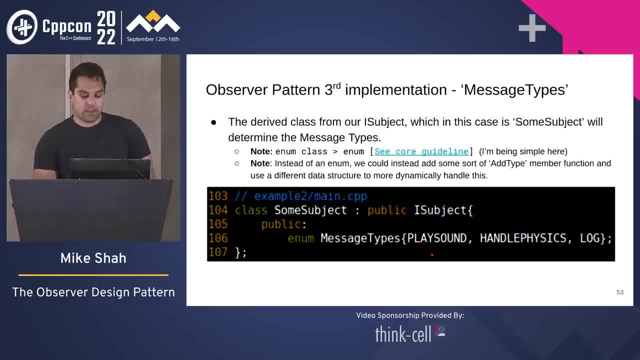 some observer. that's part of the sound system here And of course you could also make this more flexible over time if you wanted some subject to be able to listen to, not just these message types, And then maybe you add a function for add type or remove type or the things that are allowed in this particular system. 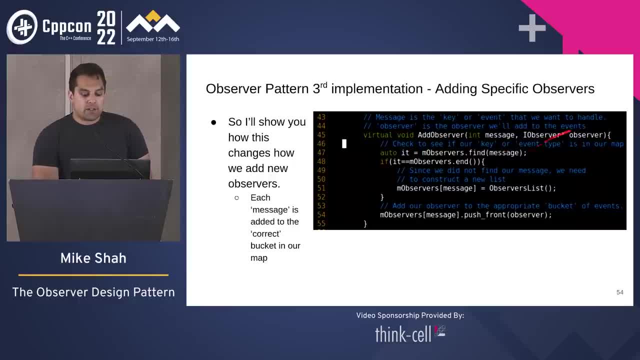 All right. so now we want to be able to add specific observers, So this is what it looks like in the code. We'll have- and this is part of our interface for our subject: an add observer, member function, the type of message that is, and then, of course, the observer, whatever that type is. 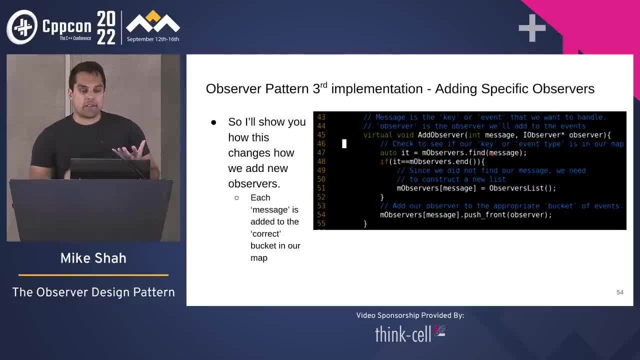 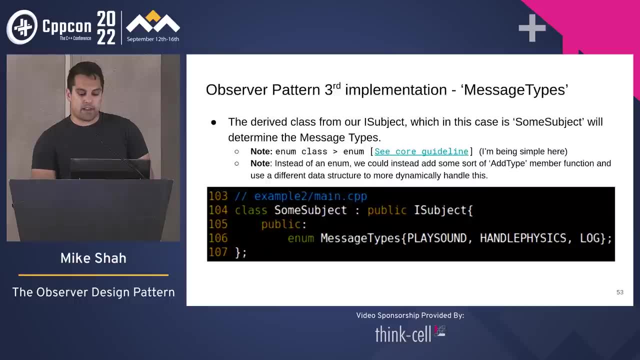 I won't make you read through this, but basically this is just what's creating that hash map for us, or that map data structure, right, that map of lists. Okay, so if I go back here, that's creating this. here We have our keys free to the systems and then the forward list. now 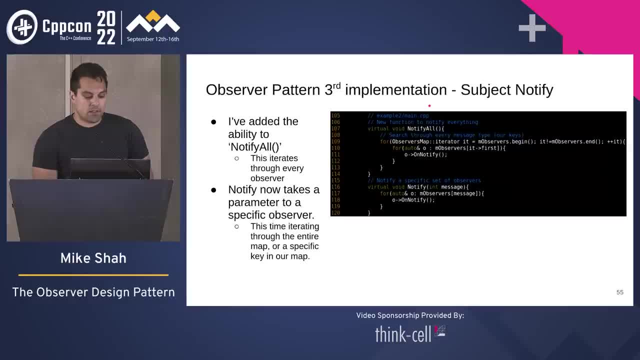 Okay, so that's the idea, All right, and then now, also as part of our subject, our interface for our subjects, we need a little bit more power. So we're going to have two ways to notify if something interesting happened. 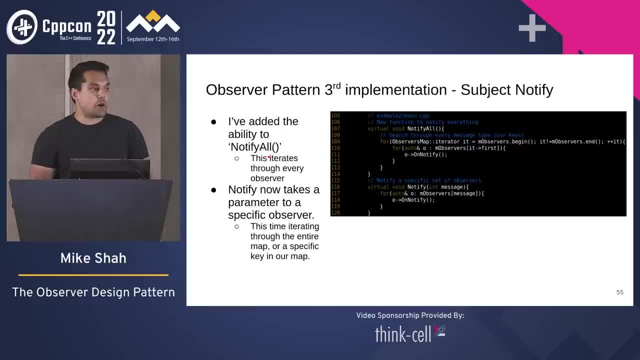 The first, which is at the top of the code and explained here, is notify all, And that again does the same thing that we've seen so far in this talk: It just sends out. it says, hey, you know, something interesting happened, so all of my observers call that on notify. 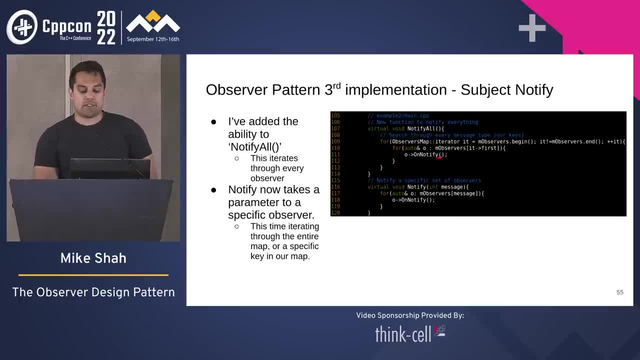 Member function. you know, however they implement it. Okay, so just for everybody. And then, of course, you can have notify this time, taking in a specific type of message here, and then just notify those observers that are part of, you know, a specific system. 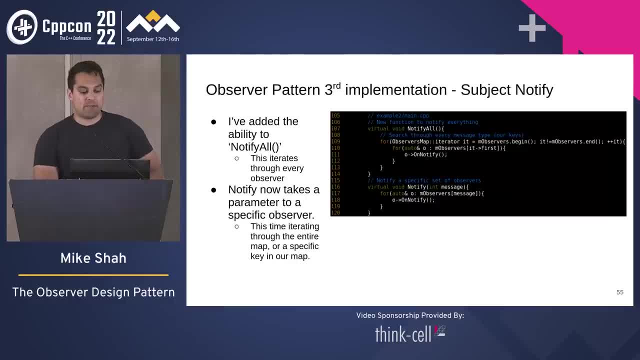 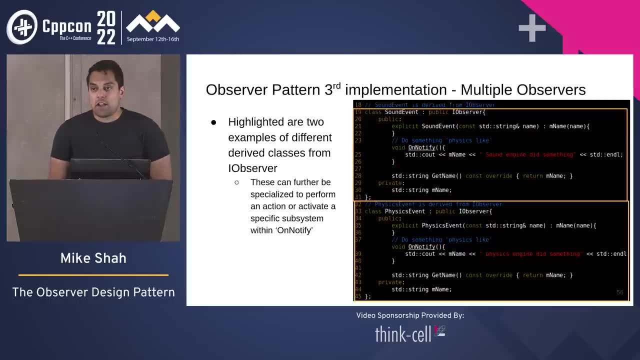 Sound system, physics system, log system or whatever it might be. Okay, All right, so that's taking care of the subject. Now, how about the observers? How do we create these different systems, or how would you sort of set this up so we can again sort of break our code into different units? 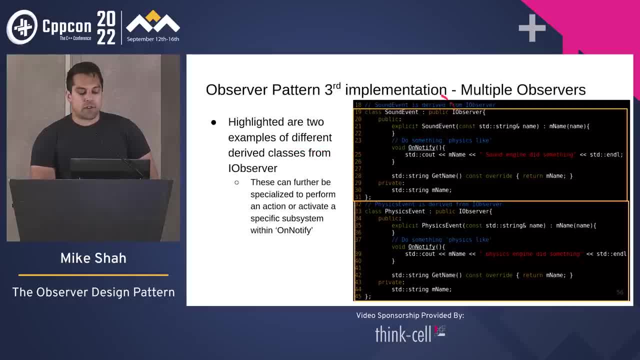 We'll highlight our two examples that I have here of just creating two concrete classes from our observer interface here. So I'll draw your attention to the top here, where we have our sound event, and to the bottom here where I have some physics event. 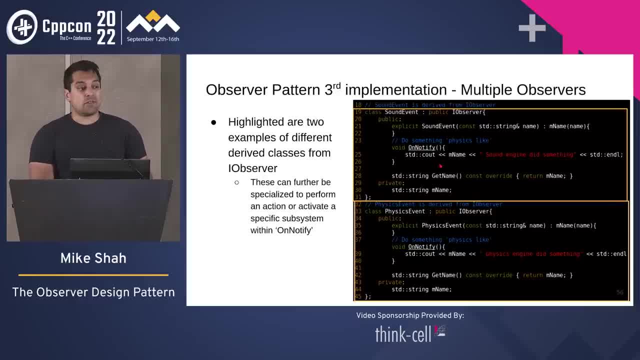 Okay, And now this is where, in our on notify, we could actually do something much more interesting, Right, All right, So for sound, okay, I'm just printing out: sound engine did something For physics. physics engine did something. 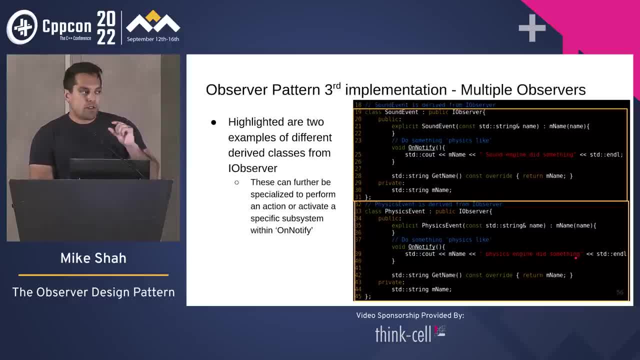 But you could actually play a sound or whatever. But again, remember the important thing: from the bad code we started with right. what we're trying to improve is my sound event here doesn't know anything about the physics system. My physics system doesn't have to have- or shouldn't- again I'm going to argue- any of the sound code in here. 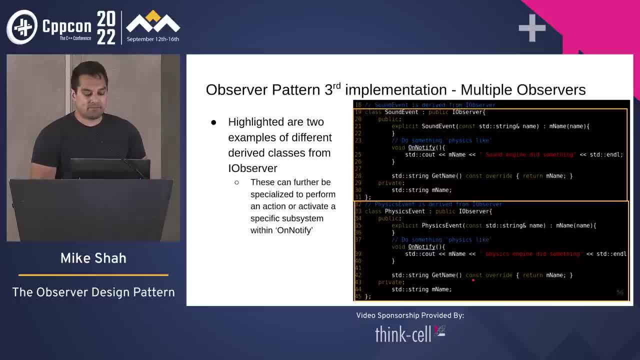 Okay, So we're effectively decoupling these things now. So I'm going to go ahead and show you how to do that. So I'm going to go ahead and show you how to do that. So I'm going to go ahead and show you how to do that. 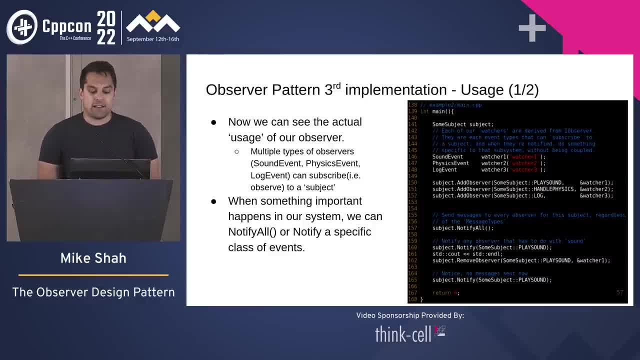 All right, So looking at the actual usage of these things, so how do we create our subjects? We'll just kind of walk you through here Again. the top looks pretty similar. Some subject hasn't really changed, But lines 146 to 148, I'm creating three different types of events. those new observer types that I have here: sound event, physics, event log event. 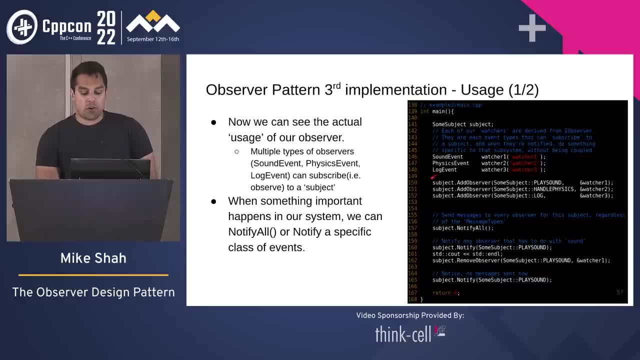 They've got the same names and so on. But what's interesting or more interesting is that I've got two types of events. But what's interesting or more interesting here- at lines 150 to 152, is now I'm able to add observers to specific systems. 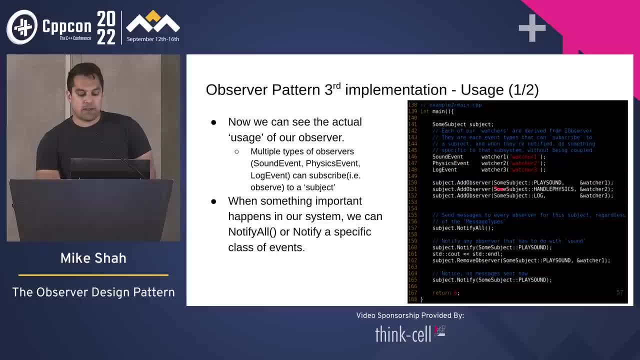 So again, sound event here, which is watcher1.. And I'm saying, okay, some subject. that's where that enum belonged. that's part of the sound system. So play sound or sound system or music, whatever you want to call that. that's what watcher1 is going to be part of. 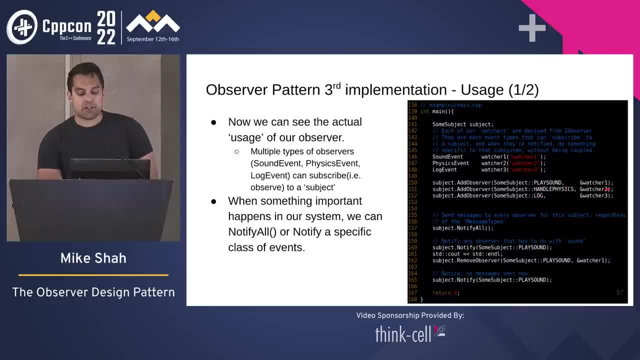 Okay, And then repeat the same thing for handling the physics for watcher2, because watcher2 is a physics event And so on. so on, All right, And then actually, as far as running this line 157, I just notify everything. 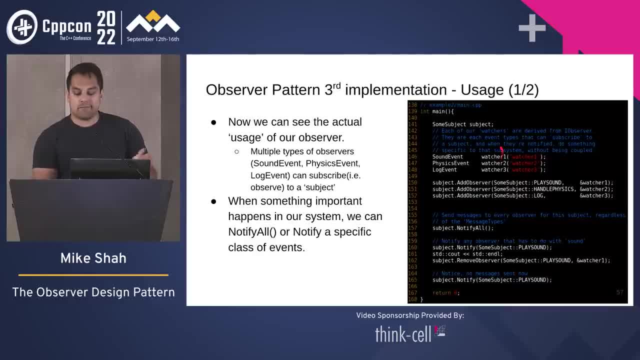 So again, nothing's changed. I want to actually just call on notify for each of these watchers And then later on, at line 160, I'm actually going to notify a specific type of observer. I'm going to say, hey, anyone who's part of the sound system here, you call your on notify function. 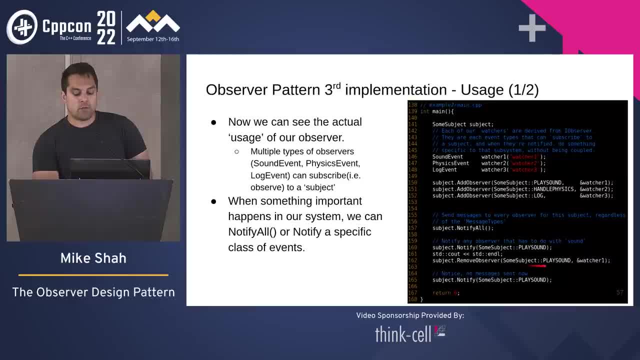 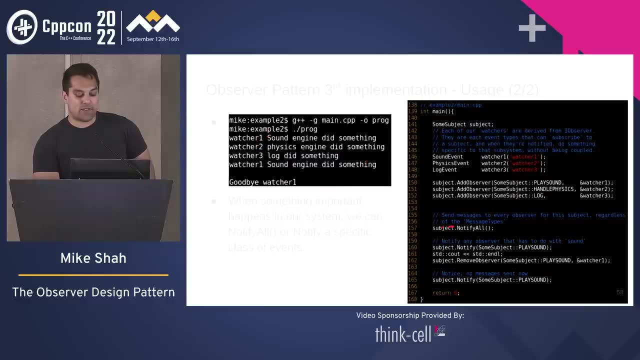 Okay, And then I'm going to remove watcher one which is part of our sound system, And then I'll notify again, and then you won't see anything. Okay, So I'll actually just show you what it looks like here. So this first chunk here. that's where, at line 157,, I called subject: 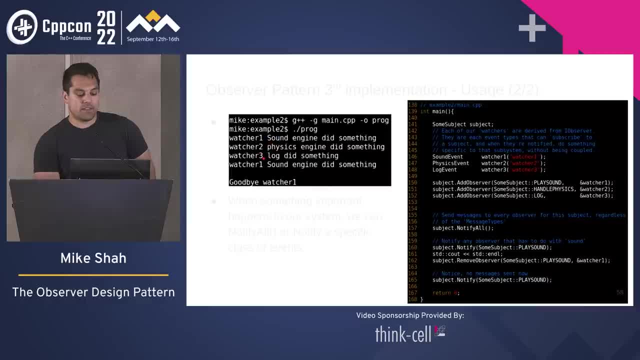 notify all. So I got watcher one, two and three, And then I came down here and said: notify just. you know, play that sound here. So I got watcher one. you know, sound engine did something And then I removed the observer And that's where it says: you know, goodbye, watcher one. 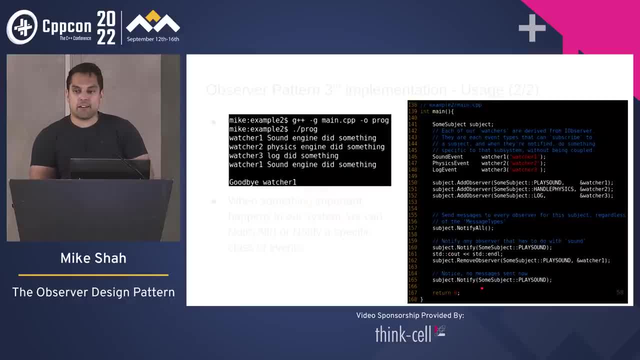 I call notify. Well, nothing happened there. There's no nothing observing, nothing interesting. no observers for this subject here that are part of the sound system. All right, Let me pause here for a moment, or actually, let me pause here and let's discuss. 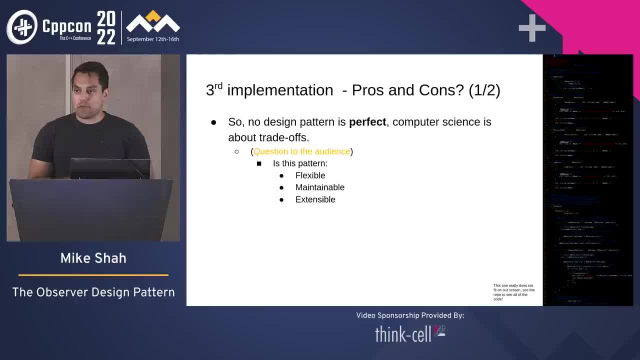 What do folks think about this at this point? Are we getting more flexible? Have we maintained our maintenance? Is it still extensible? What do folks think? Yay or nay, Hopefully, all right, More maintainable, Yeah, Oh, less maintainable Because. 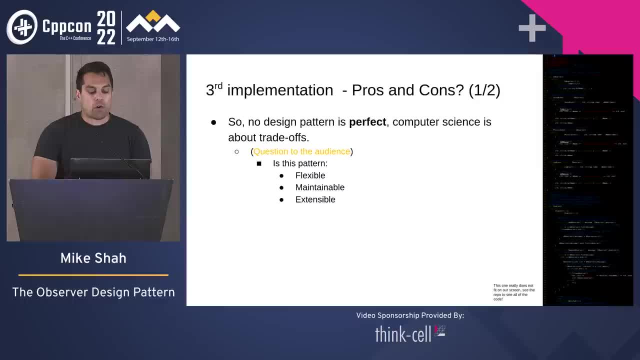 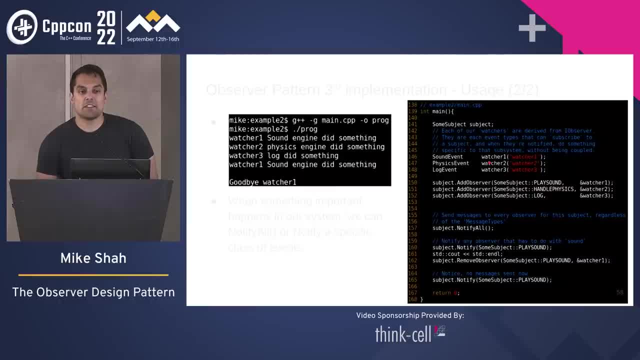 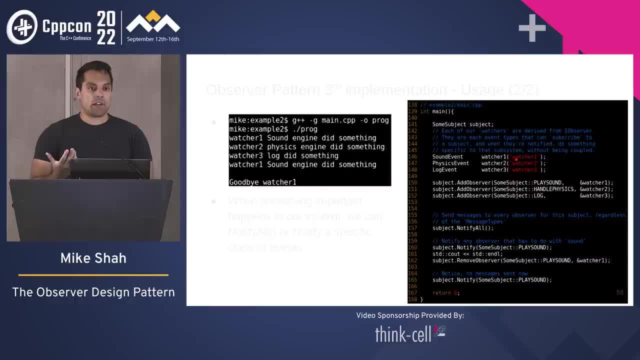 few things. One, yeah, having these heavyweight objects. if we're just doing something in our system, we could replace these with functions, with functions to the communication, if we wanna know where these were coming from or who sort of belongs to us in our system. 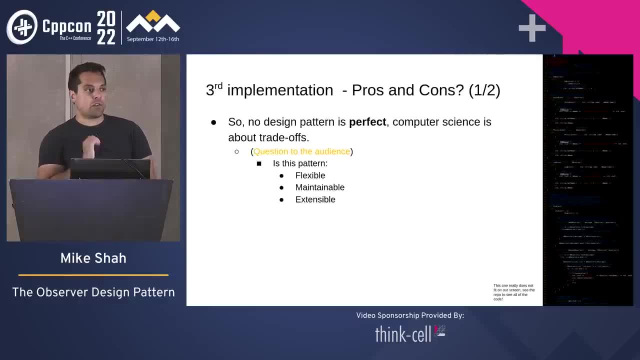 We could have that information to make it sort of more maintainable or log it. Yeah, I think it's a similar vein, like it seems like it would be easy to accidentally view, like Watcher 1,, the physics method instead of the sound. 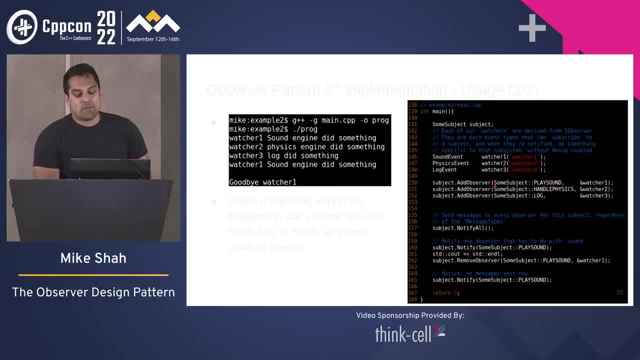 Yeah, okay, yeah, yeah, Yeah. so we're saying: yeah, here's Watcher. 1. We wanna add observer? and then well, what if I mess this up and I say some subject and this is colon, colon physics or something right? 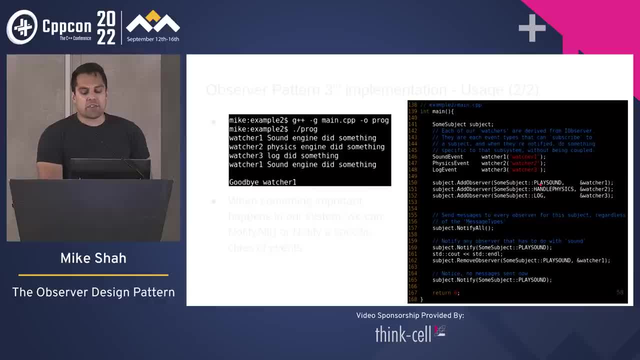 There's no sort of safety in that regard And I agree with that right And I was thinking a little bit about that. So thank you both for commenting, So we could restrict this right. We could have a little bit more either. type. 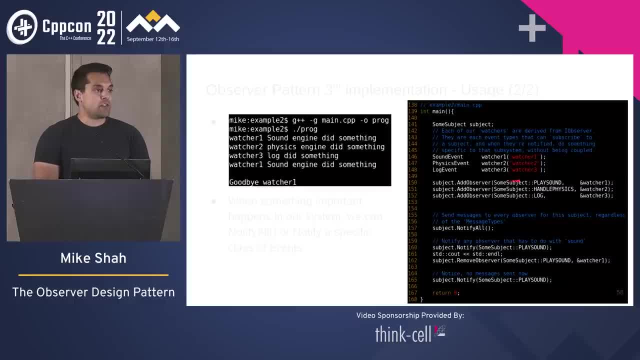 we could have type safety in different ways of: just well, right now we're using an enum, but we probably want an enum class, maybe a variant or something. to make sure we're passing the same thing For this one, I decided not to do anything. 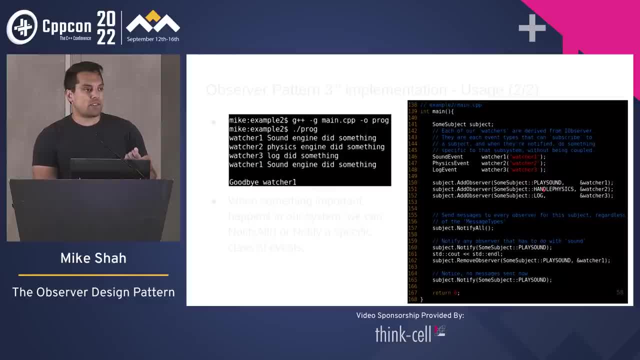 because maybe there is a use case where you want the physics system to also know about sounds, right, If you're modeling like sound waves or how they're bouncing off walls, I said, okay, I'm gonna allow myself to break the rules here. 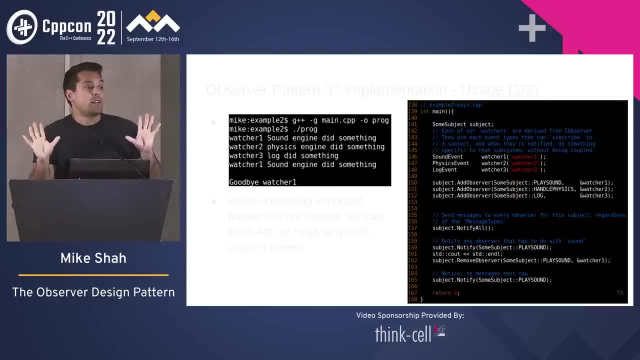 because I've seen that done in games, but maybe that's a bad thing. Maybe we want a different message for that type of thing as well. Yes, in the back, Yeah, and that's how it feels, like you can hear a lot of multiple things. 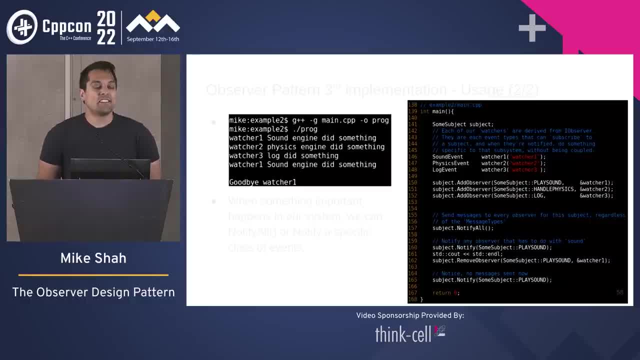 Can we get out of it? Yeah, Yeah, Yeah, Yeah, Yeah, Yeah, Yep, Yeah. so the comment was the subject: could notify about the type of event that they want? And maybe I can sort of more succinctly: this is like the C-sharp for folks who use C-sharp. 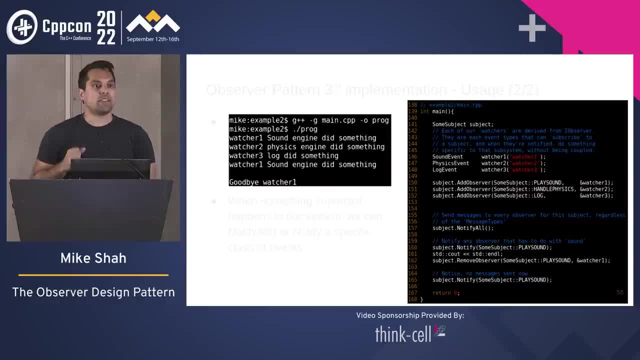 I think model or just like takes in an event. I think that's like built in, It's built into the language for folks. Okay, Yeah, I'm actually gonna show you something else crazy for this conference. I'll show you Java in a second. 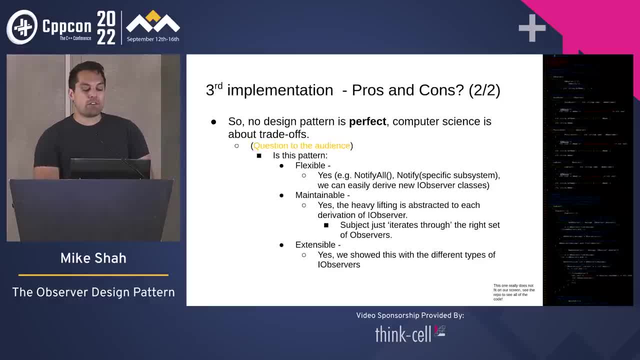 But where we're at here, at least, we're pushing more towards flexible. We have this system that can notify a bunch of things, or maybe notify some things. We are lacking type safety, which is a problem. right, Users can make errors, which I think is the valid concern. 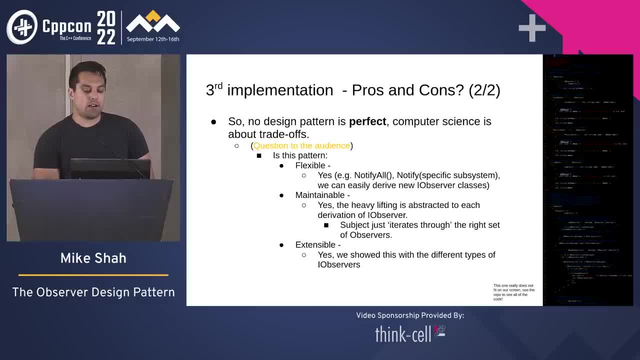 Here, right, If I pass in the wrong sort of system here. So I think we do wanna address that As far as maintainable. again, I think the heavy lifting has been abstracted out right. We're at least pushing it to the concrete classes. 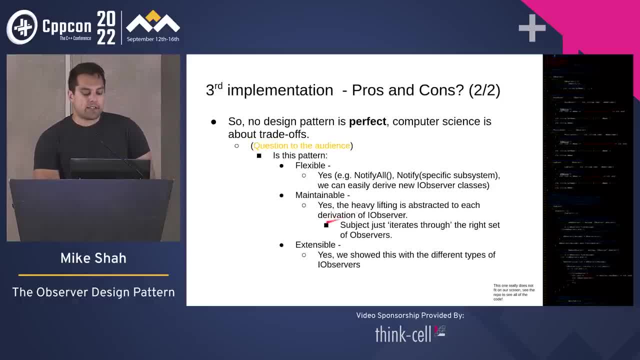 rather than just bundling everything together And extensibility. I don't think anything's really changed there. We have added sort of a complication with that little new, though that we might wanna think about like how to you know better decide what those new messages are? 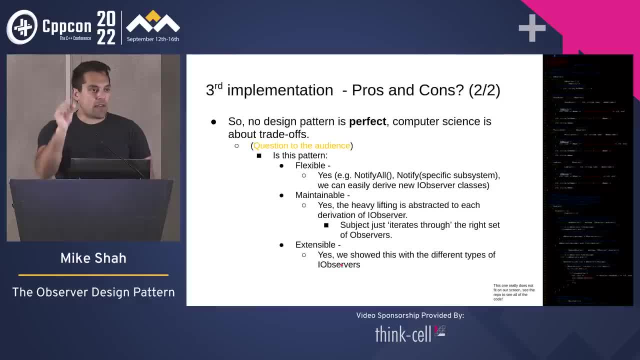 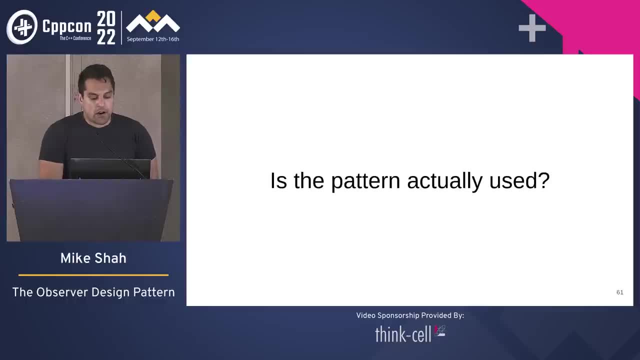 But overall pretty reasonable That we could have also different types of subjects that have their own lists for different reasons. okay, All right. So we're actually wanna. that's the last sort of big code dump as far as iterations, But you know I was thinking about this pattern. 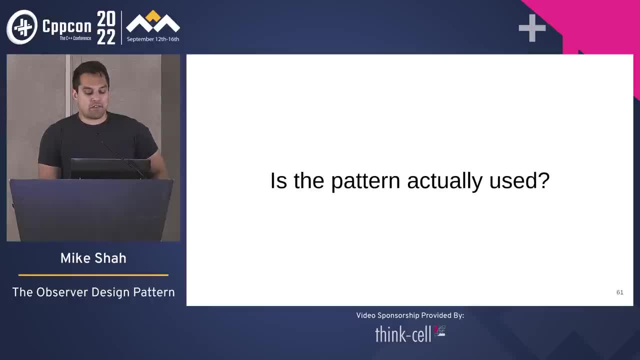 It's pretty pervasive. I mean, I think that's why we have an audience for it. You've heard of it, but is the pattern actually used? So I thought a good exercise, and especially since we've had some discussion about like. 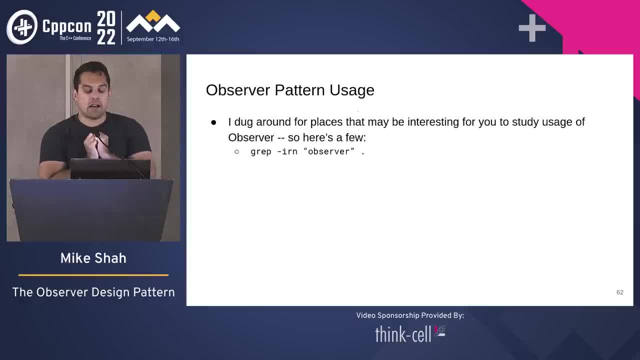 well, how would you tweak it this way? Or what if you passed in the event, with the actual like the subjects? the best thing to do would be to just look at some code. So I looked around just at some kinda graphics-y systems. 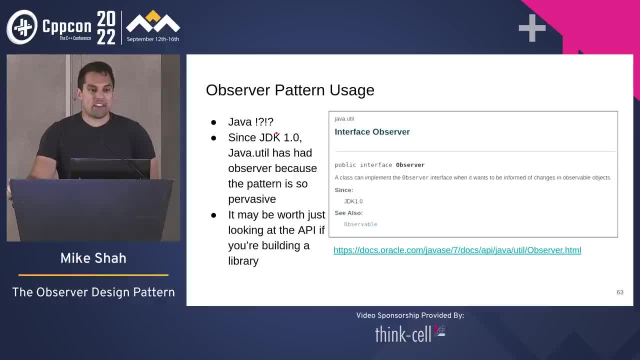 and also Java, which happened to be one of the first results. when I was sort of studying about observer. I found out observer has been so important In model view of controller and graphical user applications, these types of things, Java, since their JDK, one has had observers. 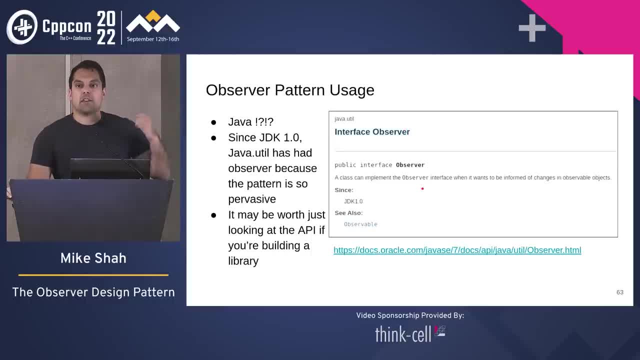 in their utility library, okay, And they have sort of a similar thing with notify, notify- all this sort of API. So this might be interesting for folks to look at if they're trying to figure out, well, how should I model things or what should it look like. 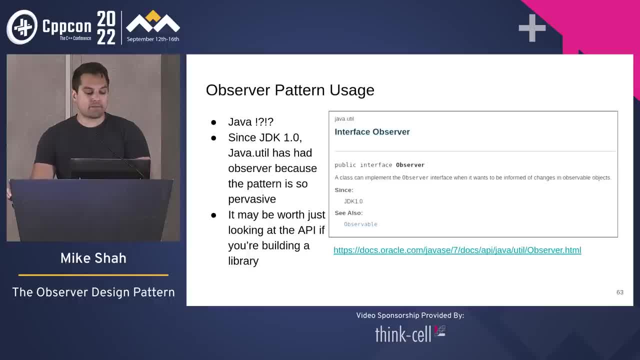 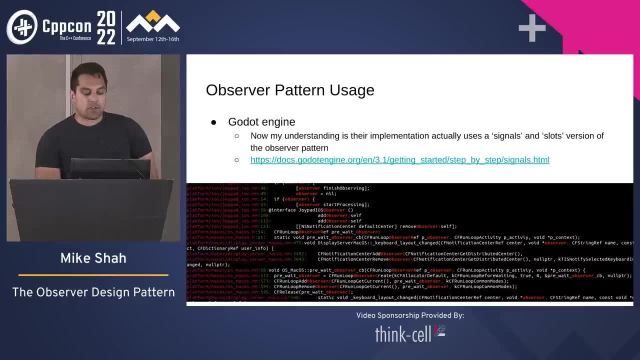 Again getting some of those finer details correct. Few other interesting source codes to look at the Godot engine. So this is completely open source Again. just wrapping around, for observer pattern They actually use something called like a signals and slots. 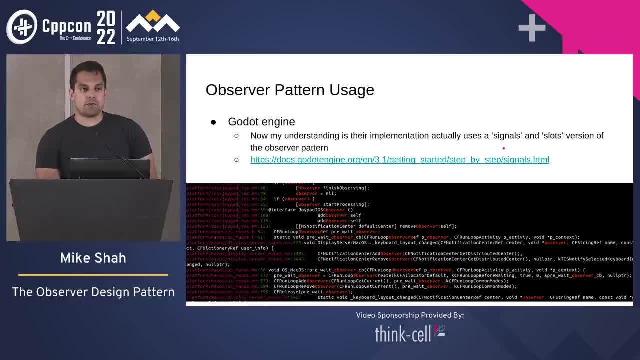 I think this is also pretty pervasive in Qt. Are folks familiar with the Qt or Qt library Write this sort of pattern? just another way to sort of have things- and by things I mean objects or functors- listening to their subjects. okay. 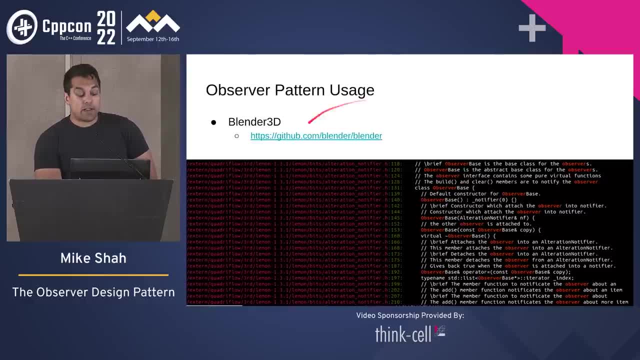 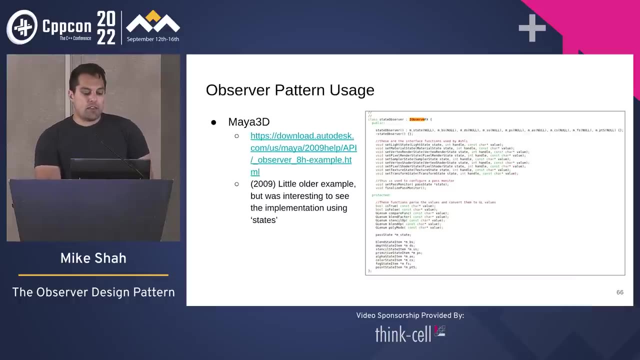 So an example there. Blender 3D, another big open source application, has lots of different observers or a base cases. I think there's just a little bit closer to what I've shown. Maya 3D, again another sort of interesting example. 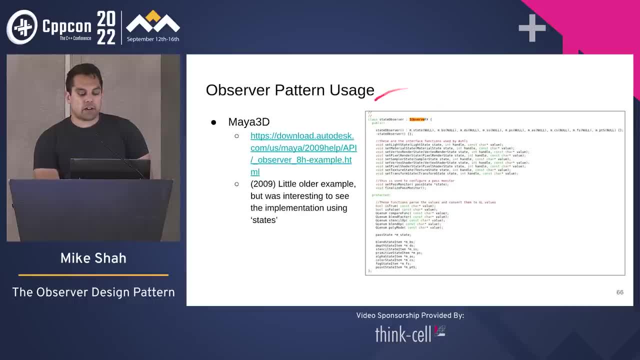 This one was kind of interesting because it had different states that it could observe, And I apologize, this is a small font, but you'll see that there's maybe seven or eight different states here. You'll actually see the constructor for for things that can happen. 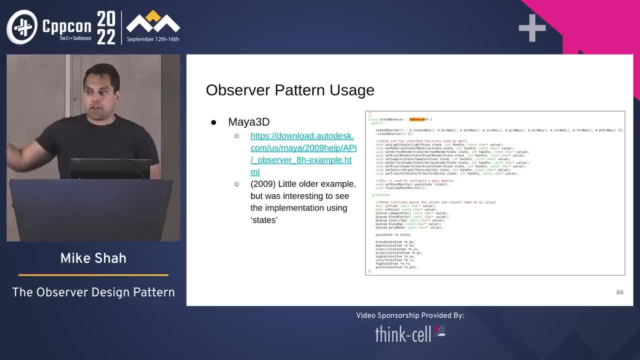 Okay. so again, you know they don't have some giant lists that you can extend indefinitely. They just said, hey, there's gonna be eight things here or whatever, and those are gonna be the different states that we keep track of and can change. okay. 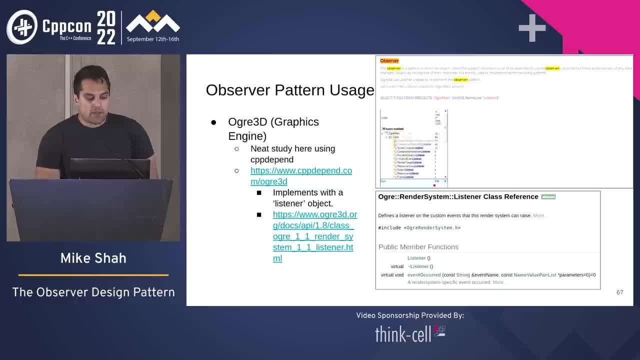 So again a little bit of a different model, And then finally Ogre 3D, which is another open source engine, And this one has per system, or of some of their systems, specifically their render system shown here- different types of listener classes. okay, 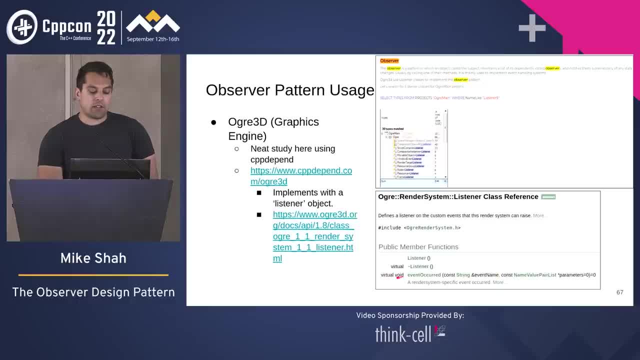 And just looking at this member function signature, here this event occurred. I think this is what folks are talking about. they'd like to have here. They'd like to know, you know, what the event name was and then maybe a list of things that are affected here. 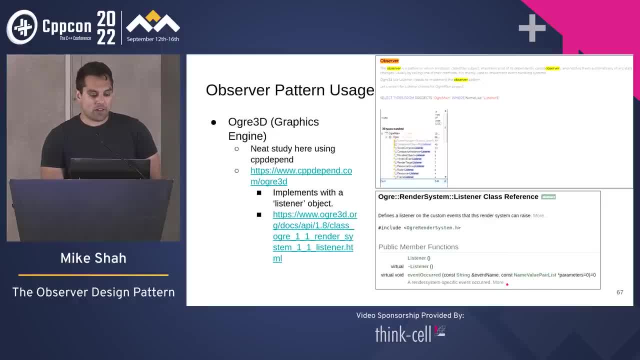 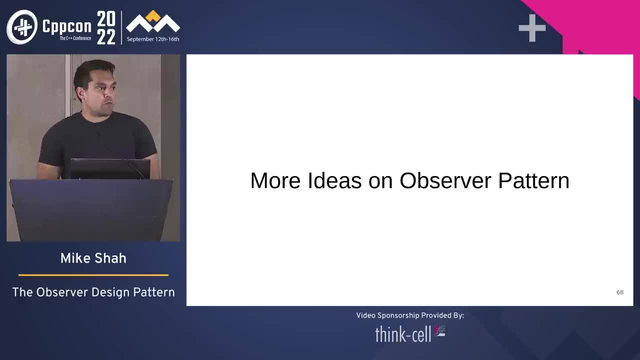 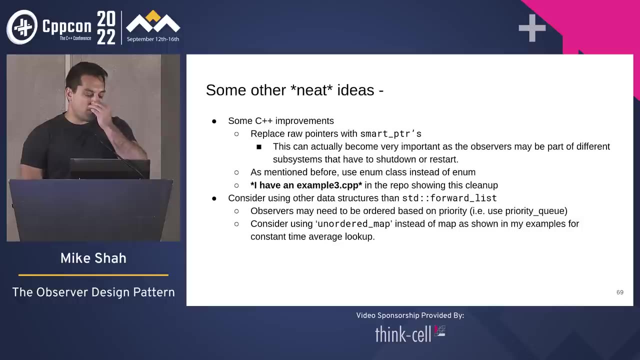 So that's sort of the idea here. All right, so a few more ideas on the observer pattern, since I think we've got one that works. it can be improved a little bit, but some other sort of neat ideas and places where we can improve things. 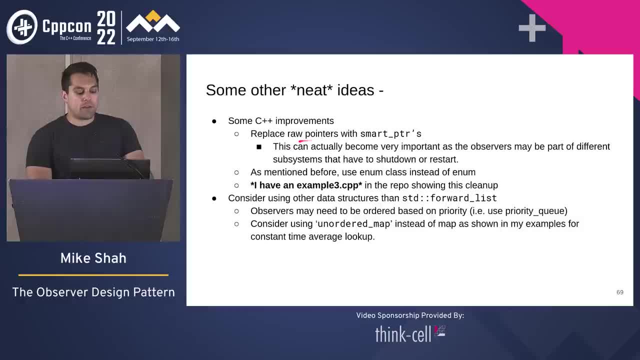 So folks might've mentioned, you know, raw pointers. We can replace these with smart pointers, right, And then we can at least maybe avoid some issues. Someone mentioned, you know we could have a dangling pointer, these types of things. 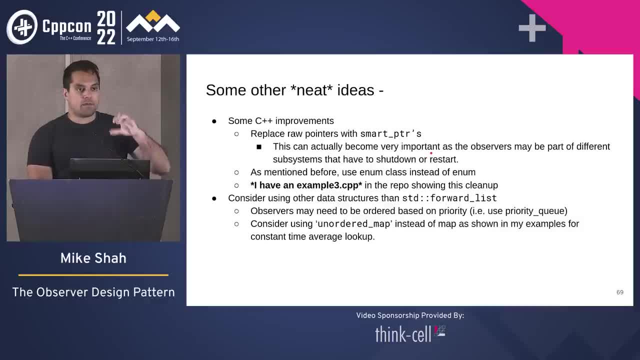 We do actually have to think carefully about ownership, though once we've subscribed to something, you know if we're gonna use something like a unique pointer, well then you've got to move ownership and then think about what the lifetimes are gonna be. 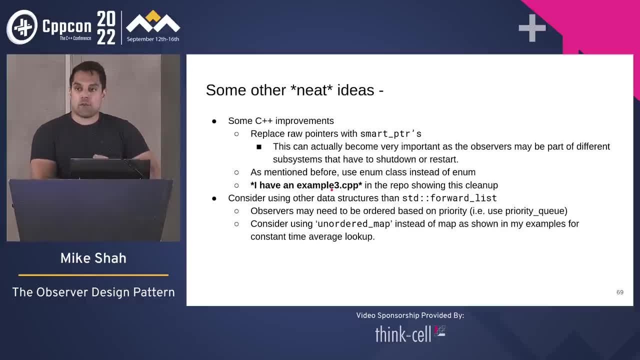 I'll show you an example, briefly, which is example three: CPP in the repo, where I use a shared pointer, which is probably, you know, the default to use smart pointer. but I'll talk about that again. There's some other things we might wanna think about too. 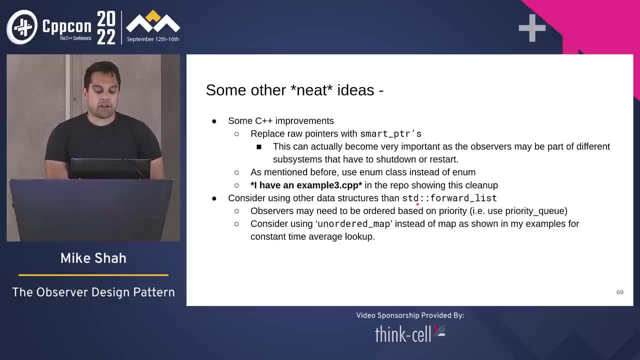 I've been using forward list pretty frequently here, but that's another thing we do wanna think about our control of, So you know as adding those watchers to some subscriber in a specific order, does that matter? Okay, so if it really matters, 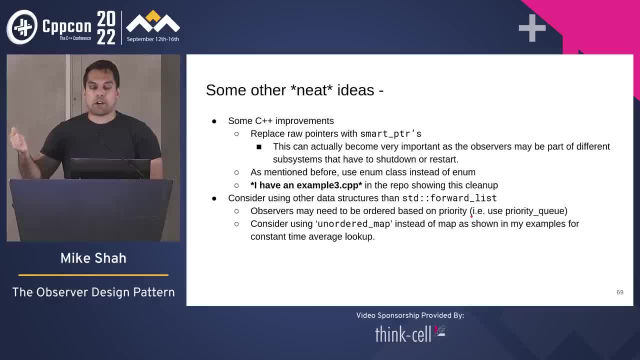 you might think about some other data structure, like a party queue, to make sure that all the physics events happen before the graphics events. Okay, if you have, you wanna move something or simulate the actual motion and then display something, right, So you might think about those kinds of things. 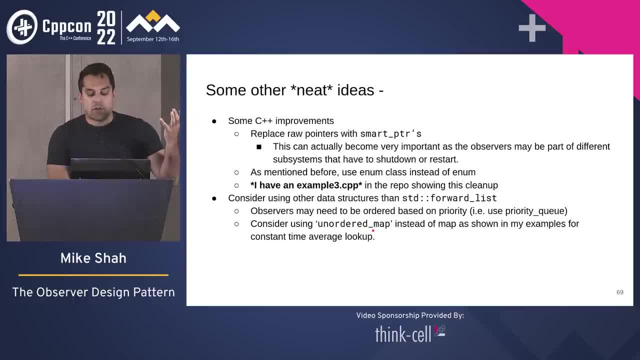 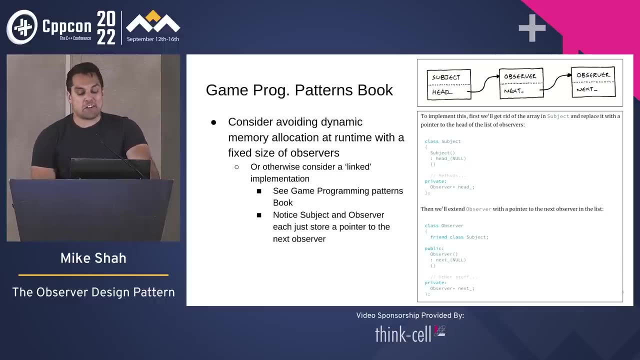 For most of this code. I was showing map to preserve order, but unordered map, if you don't care, is gonna give you better average case performance, constant time lookup, The game programming patterns book which I mentioned earlier and again. I'm gonna encourage everyone. 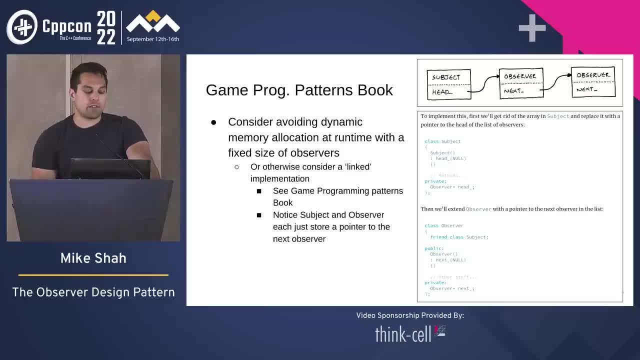 to at least read on. the website also shows some other interesting implementations of the observer. Again, we have to think about if we're creating lots of these objects. I was creating objects today which could be much more heavyweight than functions or other things. 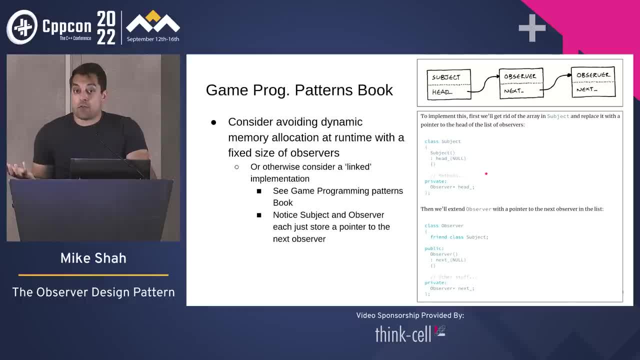 has another way that we can sort of just avoid doing dynamic memory allocation right, But essentially just having the next observer. So from our subject we have the head and then each of the observers point to the next observer rather than maintain that list in the subject. 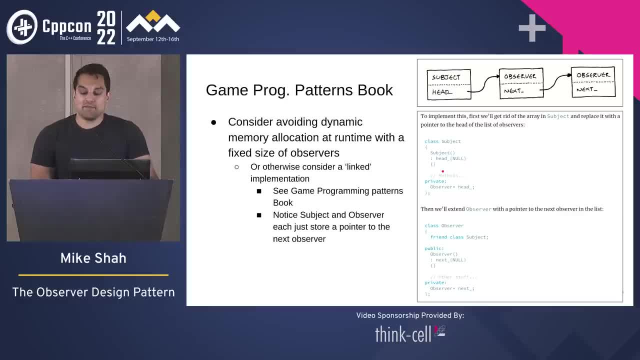 We have a question online. Can I Signal slot lifespan management are the trickiest challenges when implementing observable Cued signals, boost signals to address those. Is there a chance that C++ would provide a standardized solution out of the box for such commonly needed patterns as observable? 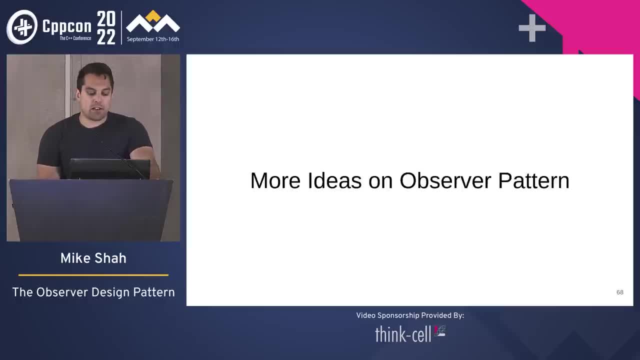 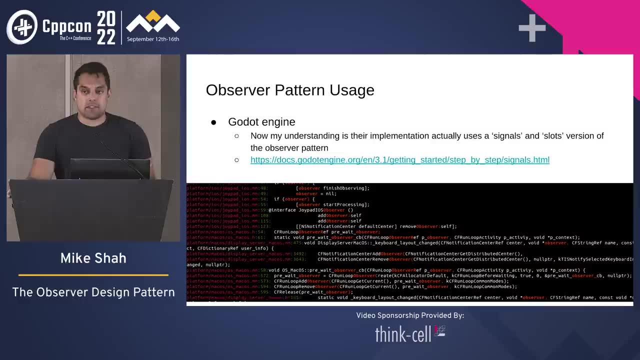 It's really good questions, The questions about you know. just rewinding back. Let me go back to which one did I have? signals and slots, This one from the Godot engine, and about standardizing some of these patterns because they're tricky to get right. 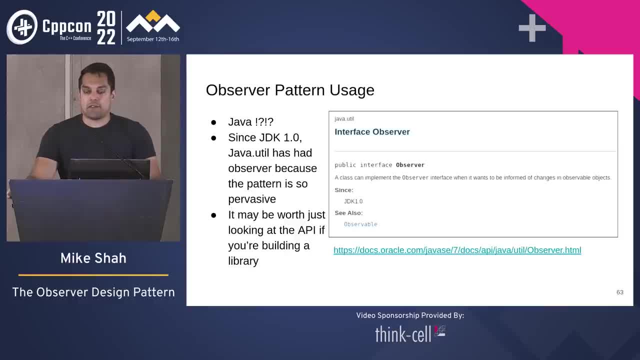 I mean, we saw the instance where in the Java utility library they have this. I don't have any insight, nor have I written any papers about proposing this, but I think this could be a good sort of proposal or something to think about. 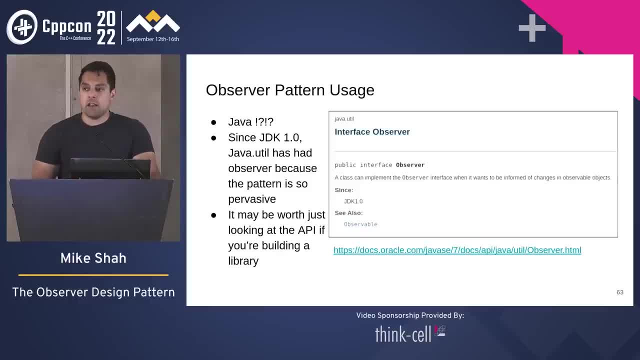 We are getting more sort of data structures in C++ 23,, different types of maps and sets. It would be interesting to see some of these patterns that we keep using and maybe implement them. Observers, I've implemented it. It appears pretty reasonable. 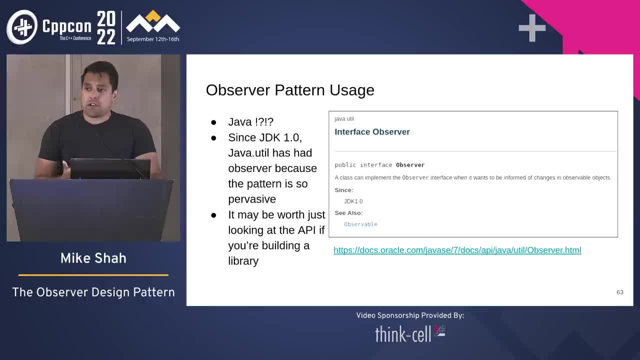 but getting some of these right is tricky. Now we do have to also think about things. There's been actually a few talks about Atomics, and there's a really good one I'm gonna reference from Tony Van Erd about building a lock-free implementation of a Zerber. 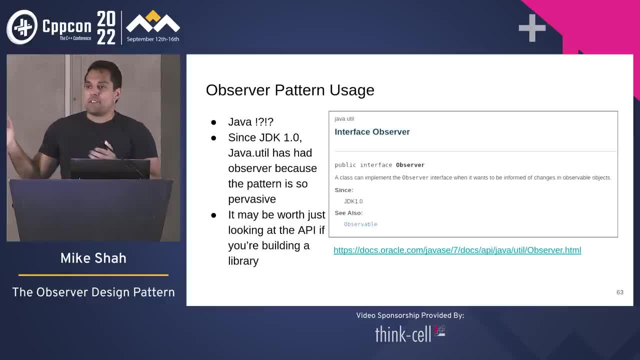 Again, that would be hard. That's hard for me to write, so I would love to just use Tony's and have that in the standard. I don't know if it belongs in the standard, but there should be some libraries here, So that's a great question. 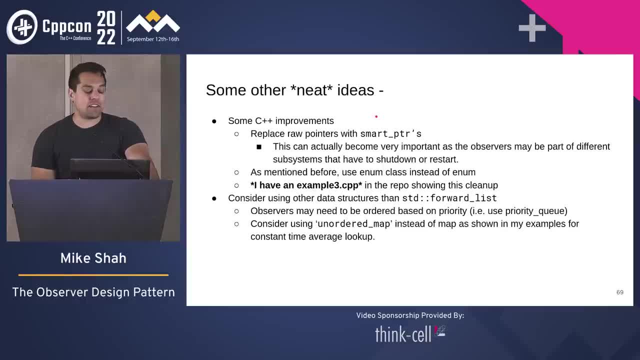 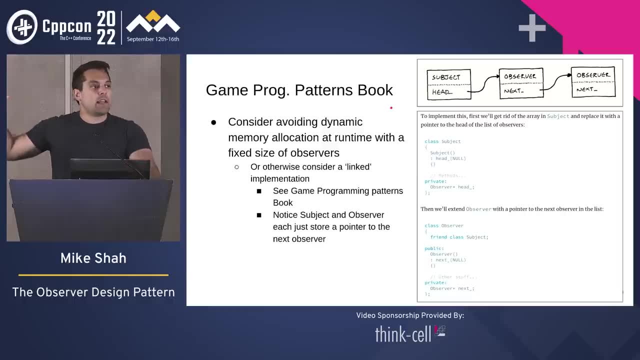 And this falls right into our sort of neat ideas or things that we need to be thinking about. Let me move here. So, again, this is one way to. again, if you're concerned about dynamic memory allocation or having lots of observers, you might go with this approach. 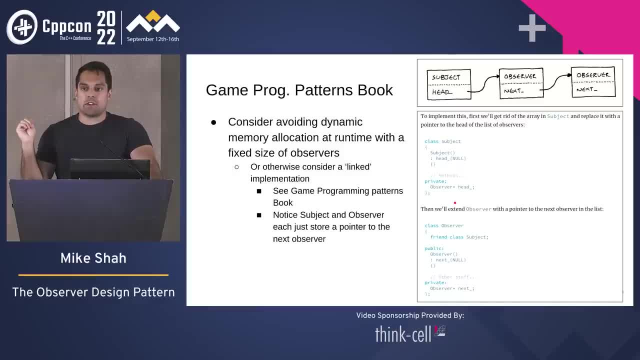 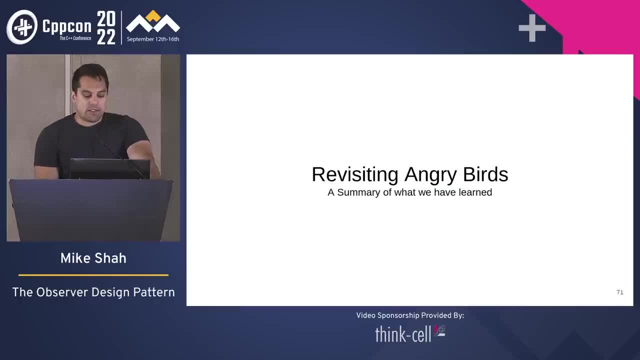 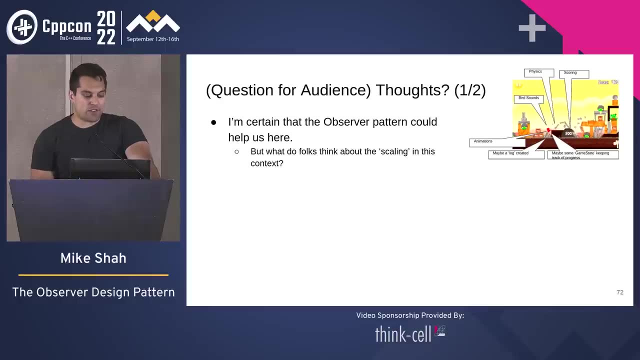 or you might just say, hey, a subject can only have 10 observers, right? That was sort of what Maya 3D was doing, okay, Okay, so let's revisit Angry Birds and kind of summarize here a little bit. You know, and this is for you folks to answer. 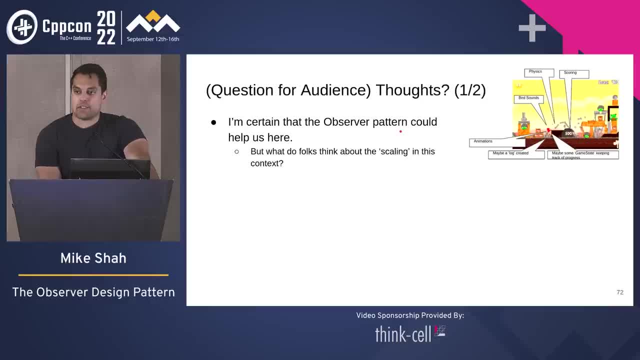 But I think the observer pattern here could help us right Where we have this bird, who's pretty interesting. it's doing a lot of things. this is our subject, and we can subscribe a bunch of or have a bunch of these sort of subsystems. 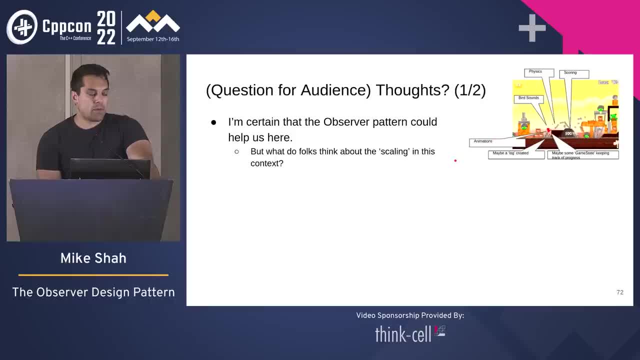 waiting to do something interesting. But my question here- as many questions, do you know- falls back to scaling. What do folks think about this? How does this, you know? how does this scale if I have? well, in this case I have, let's see. 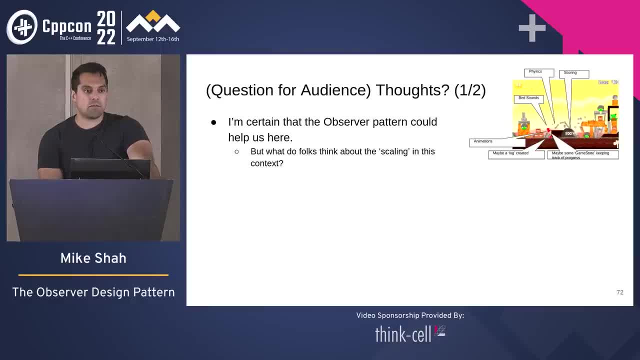 one, two, three, six observers for this one bird Is that? that seems reasonable, But what about when this bird crashes into the rock here, this stone? and that stone also has to have its list of, you know, observers and subsystems that get fired off. 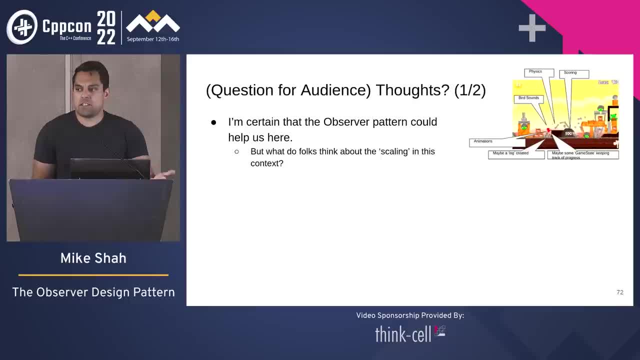 Does this seem like this could grow pretty large, Potentially right. Maybe this is fine. This is fine for Angry Birds, But remember, we're sort of iterating through these lists of observers per subject, So we do have to think about the performance. 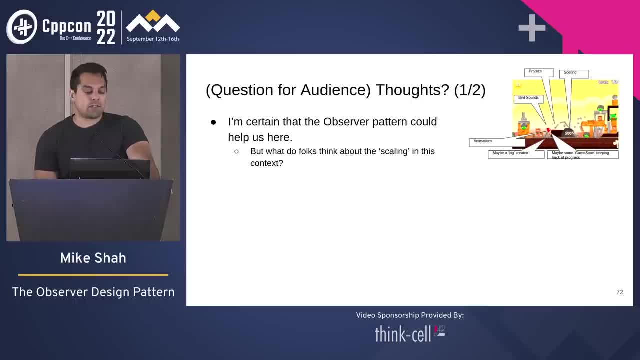 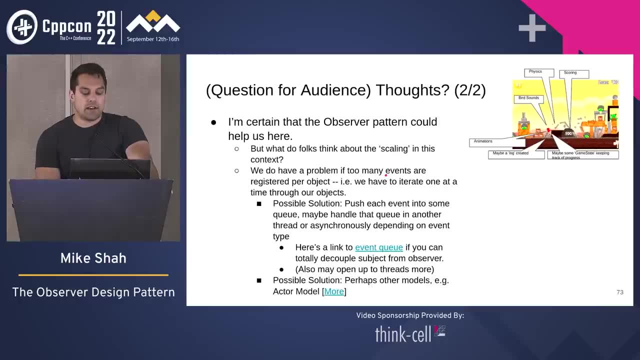 a little bit here. So my solution to this, or some things to think about: right, If you start having too many events right on, notify things that are happening per object. we might have to start thinking about pushing these into a queue, right. 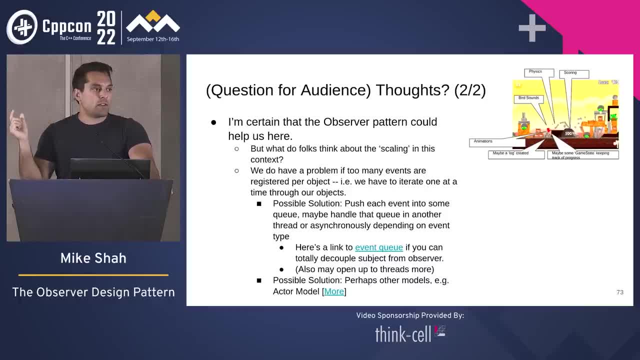 And then this is gonna be sort of a different pattern of just sort of having an event queue. Maybe those queues are for different, different subsystems, Maybe they're being taken care of in different threads. Again, we've got to sort of balance complexity. 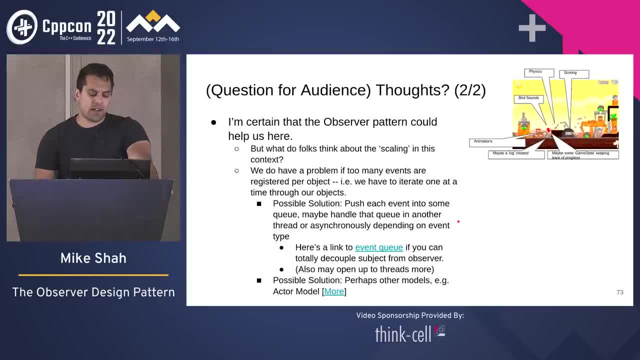 with the performance here, but that's something to think about. We might even think about different types of models if we're getting into concurrency like actors and these types of things as well, especially if we have lots of objects interacting with each other. 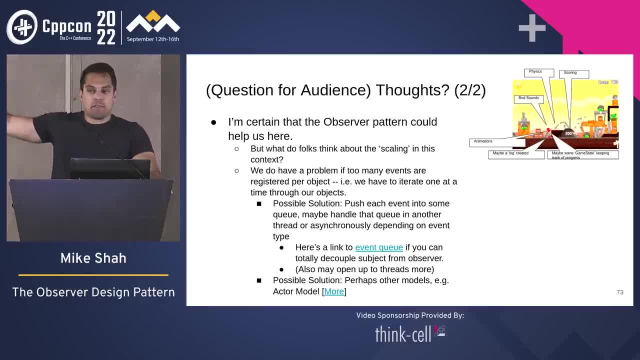 But for the most part I think, or I'm pretty convinced, at least for this scale of game, we could get away with this pattern, Okay, unless we're really- I don't know- destroying a lot of stuff or the physics system is going wild. 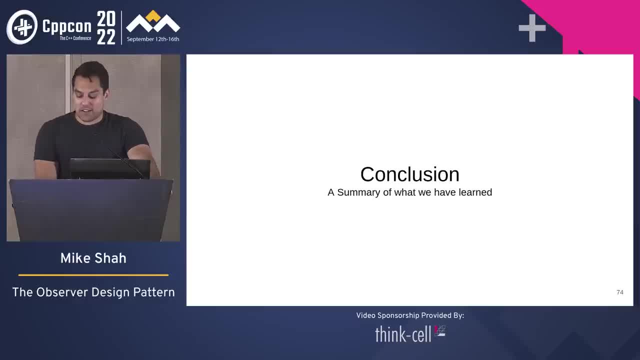 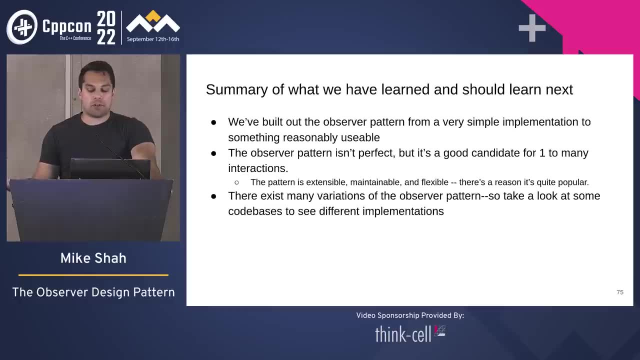 which it could All right. so kind of concluding and getting towards the end of this here and thinking about what we should learn next. you know, we've built up sort of a simple observer pattern, And the way I always like to look at these things is: 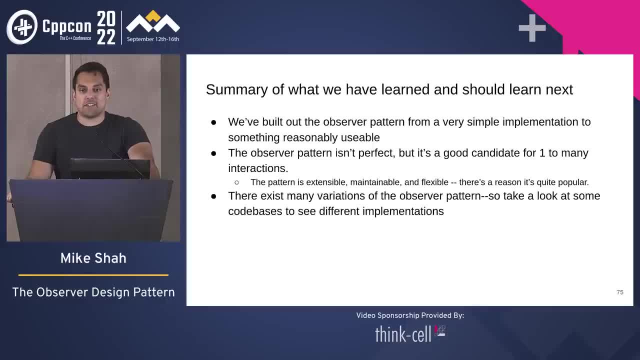 well, what did I wish I had you know when I was learning this? What's the simplest thing, right? Just start off with those concrete classes, and then we sort of built up, okay, And that's exactly what I did for my implementation. 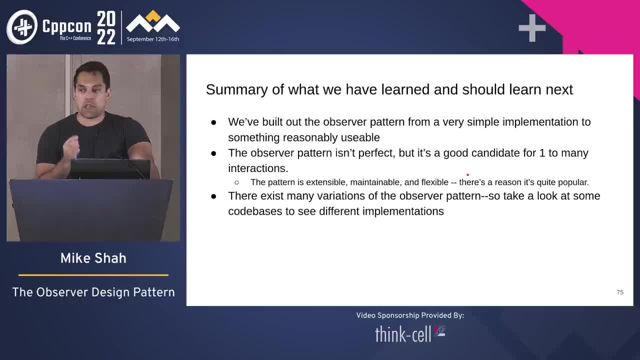 This isn't a perfect pattern. in a sense, It's usually a good candidate, though. when you have one to many interactions, it could at least be a starting point. if you're trying to solve that in your application, okay, That's why it's used so much in a you know. 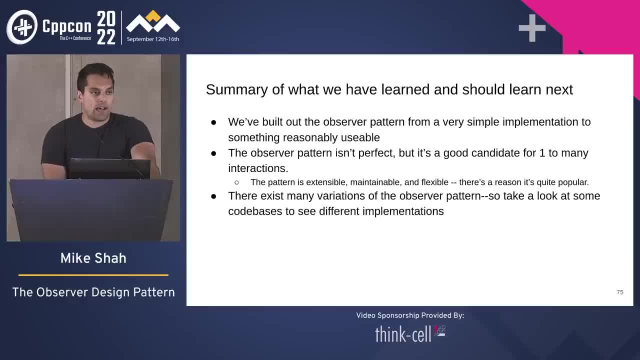 graphical user interfaces, model view controllers, et cetera, And I think, as many folks were suggesting, there are just many variations of the observer pattern where we're trying to have different requirements of what type of events so we want to allow. how safe is our system? 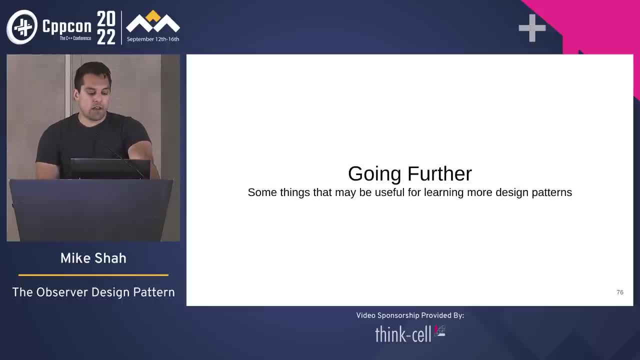 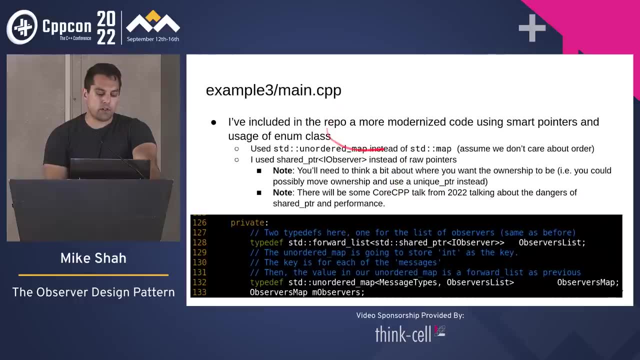 these types of things right Which we can enforce. So going further, you know, just adding a little bit of safety, modernizing our code a little bit. This is a snippet as part of the interface for the subject. You can see the whole thing in the code here in example three. 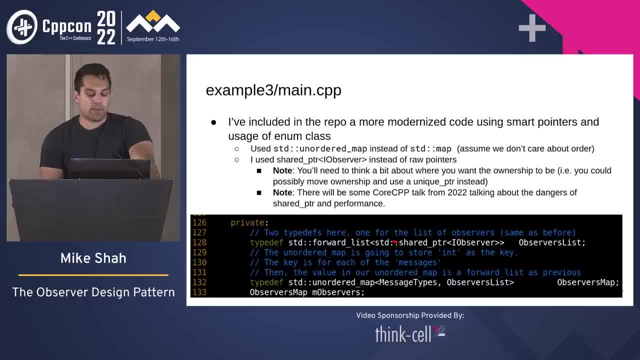 in the main CPP file. Now in this example, I am maintaining a list of shared pointers here because again, this could allow me to have a observer for multiple subjects if I want, which I won't get with unique pointers, and I don't really have to think as much about the ownership. 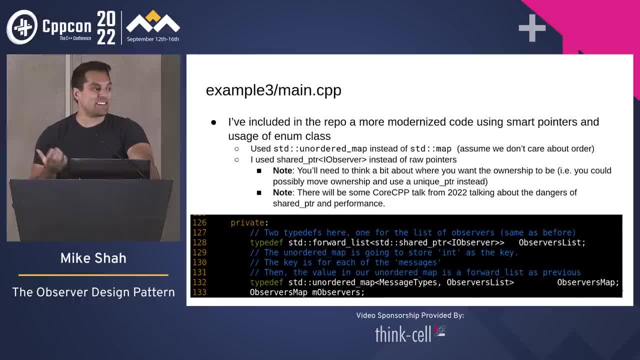 But again, you have to think about the ownership. Is it gonna be, you know, a unique pointer, But you know, in this case you have to be careful of shared pointer. Now there is gonna be a talk. I was just at core CPP. 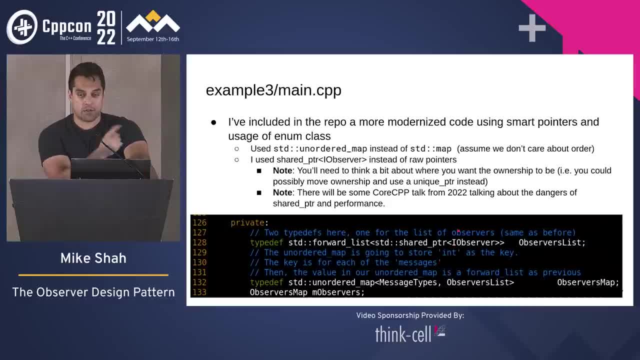 about the performance implications of shared pointer. I think there was one next door as well. There's been a couple about shared pointer and atomic performance As well, so you do have to think about that as well. Once you start sharing things, there's locks involved. okay with a shared pointer. 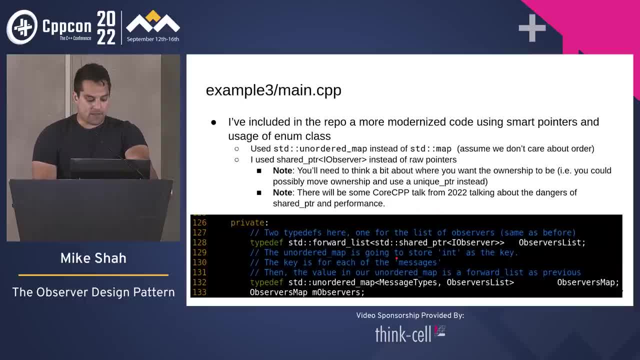 And then let's see the last thing. let's see, I believe I fixed it here. Oh, I guess I don't show you, but there is an enum class in here, I promise. Where are the messages? So we get at least some type safety. 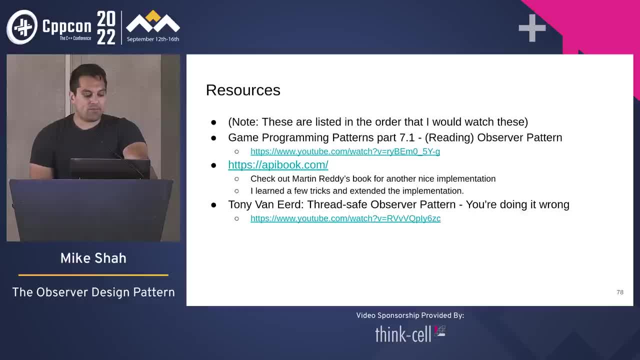 We're not just passing in integers, Some resources going further: game programming patterns book, the API book, which I'm gonna show you in a second. This is the AI book, which I think is an underrated book, by Martin Reddy. He did a lot of graphics work on Second Life. 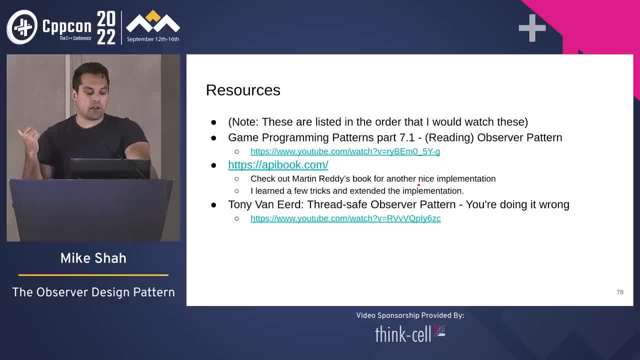 some Pixar work. He has a nice implementation of this and also talks about push-pull observers and some other models. And then this is the Tony Vannard talk on thread-safe observer pattern And to the online question. this is the type of stuff I would like to see. 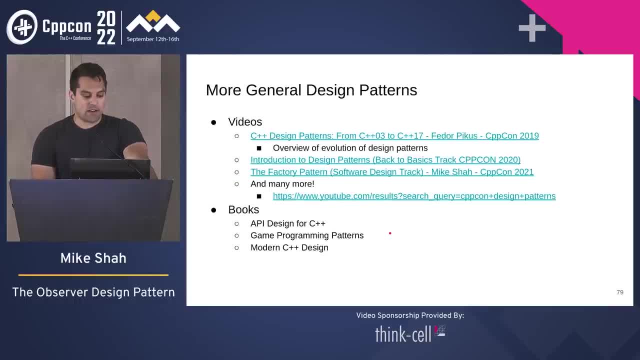 in a library somewhere, All right, So those are general design patterns from past CppCon, So feel free to check those out. Here were a few of the books again And, with that said, we have a few minutes for questions, but thank you for your time. 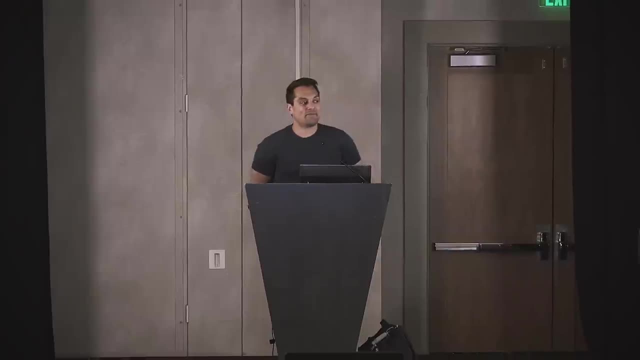 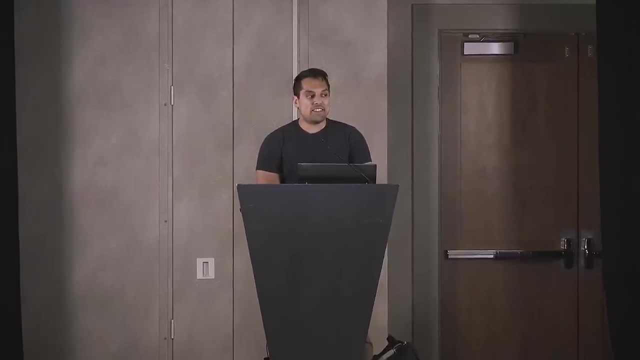 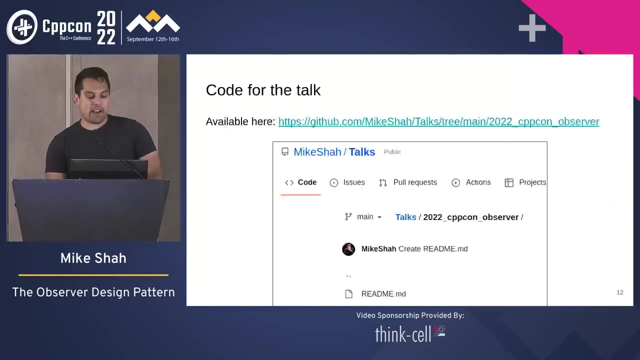 This has been wonderful. No questions Then it's: yeah, sure I did. yeah, Let me wind back to this. I'll get back to that here, Just so if you want to take a picture before this talk goes live. 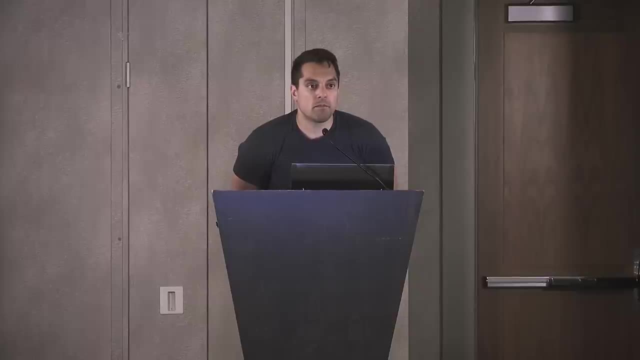 Yeah, question back. That's good. So the question was my disappointment. C++ doesn't have a interface like Java or D or these types of languages, So would it be cleaner to have a concept? I don't know enough about concepts to give a great answer. 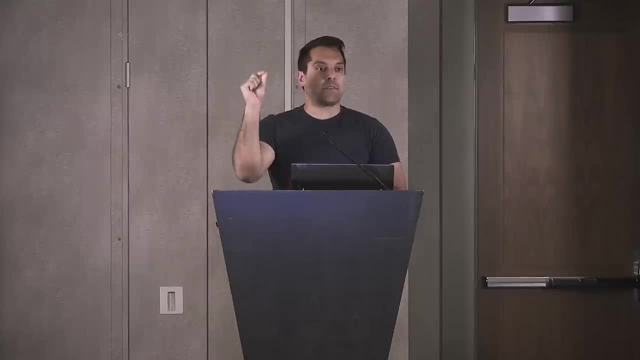 but it could be the right tool, right Because the idea is we're enforcing right Something that we're driving from has some functionality. So if that's the case, in general I'm a fan of what I understand of concepts. 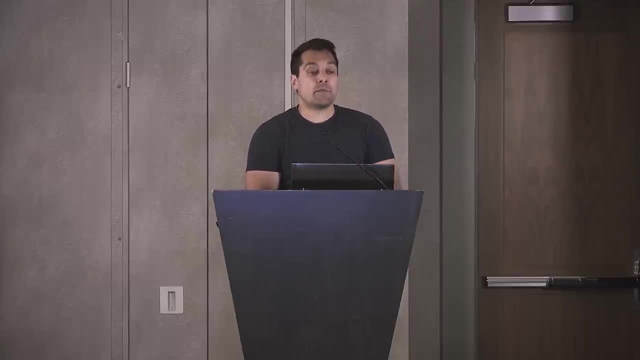 I think it's gonna make code very good and very safe. It has that potential. so absolutely, Yeah, Yeah. so the comment is: why not go a step forward and make this templated right So we could have- well, I guess we would sort of get- the extensibility. 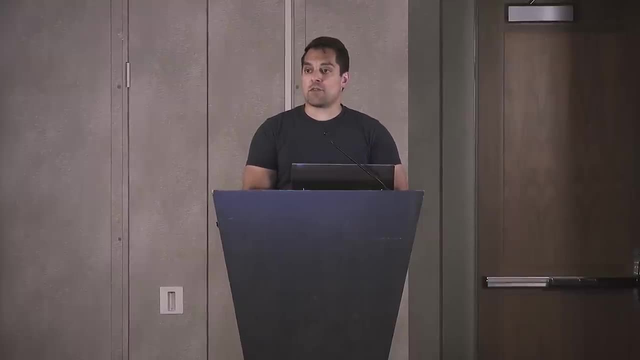 or I guess the code generation from templates, maybe the additional performance as well if we know what types of systems that we wanna generate, or subjects. I guess that can listen to specific observers. I think that that's a great next step, yeah. 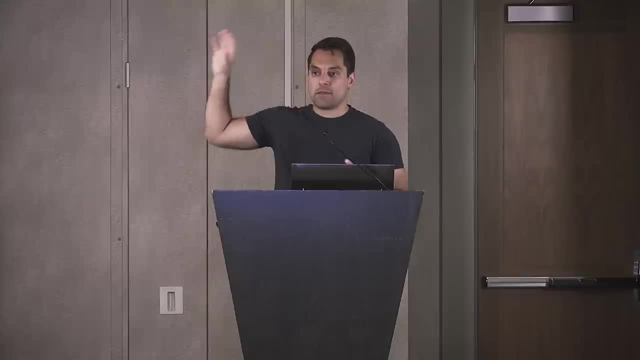 I don't have any argument. I think that would be right. if you're sort of following along, that would be a great next progression. you could try Right, and then you could have other types of- I think in a place to look at this. 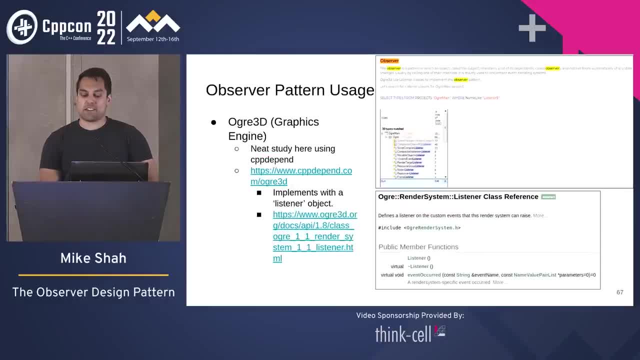 sorry to move us away would be the Ogre when I was looking through their different code base, because they had like render system and then like a specific type of listener for that thing, And then they had another class and a specific type of listener for that. 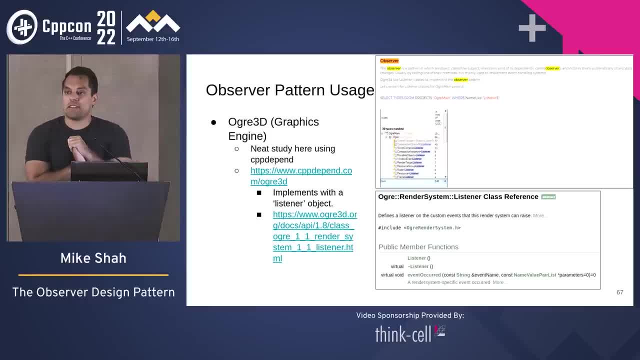 It's like: well, you could template that out or maybe look at the, in this case for graphics. they probably have a lot of concrete classes, but that would be a great place to look. yeah, Yes, So if you're using shared pointers for the observer. 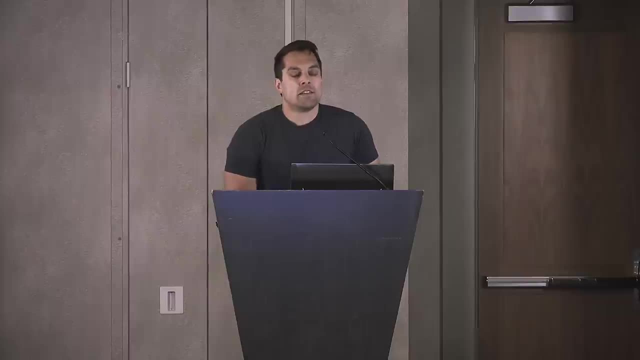 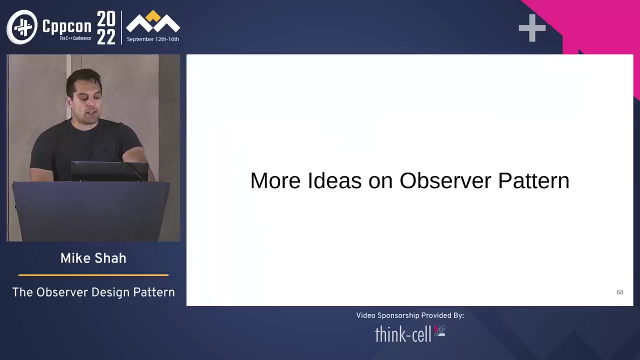 what's a good way to manage the lifetime of the observer? The question was, if I'm using a shared pointer for the observers, what's a good way to manage their lifetime? Well, I guess we get. and I guess, let me go to the 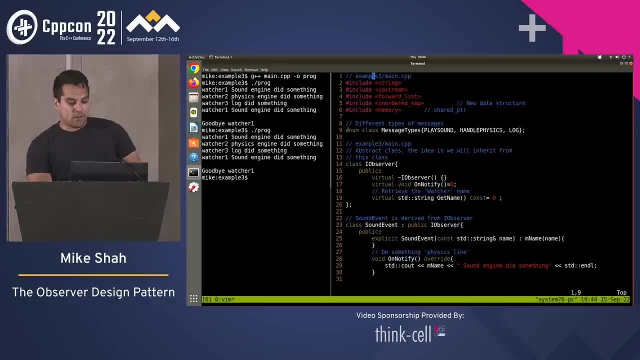 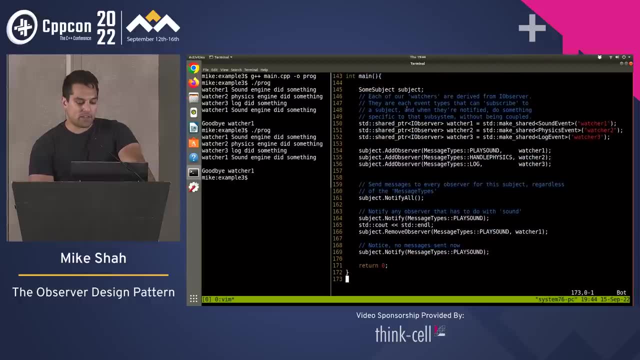 I have the code here. here, as promised, a new class. Oh, I made it global, though Don't look, Cause if we look at this with the shared pointers here, all right, I'm just declaring them in main, So they're pretty much just going to live forever, right? 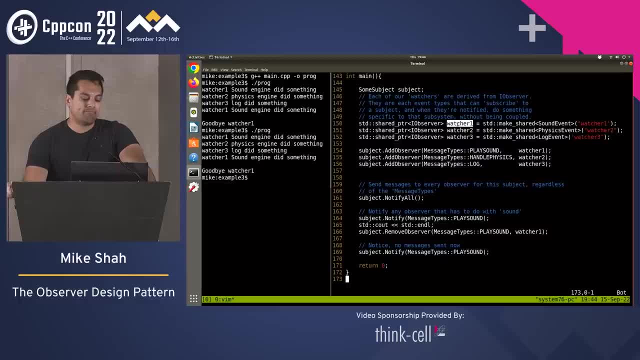 We'll have this reference to them: Make them weak pointers. Yeah, that would be one way to do it. Yeah, Yeah, Yeah, Yeah, Yeah, There will still be the cost of shared pointer right in that. we have to when we're like iterating through. 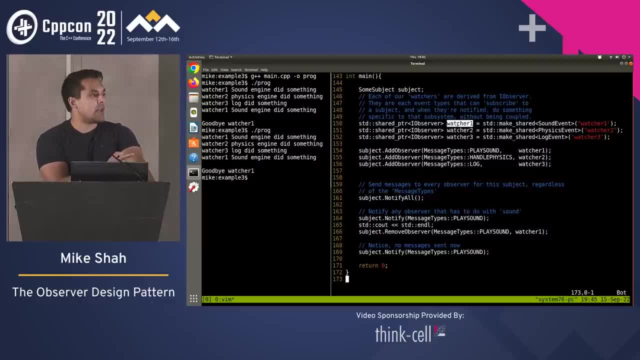 and lots of things are happening. you have to maintain that, but for the lifetime, especially in an environment- like a game too, where we have objects being destroyed, again destroyed, or maybe they're recycled. but using a weak pointer is not a bad idea. 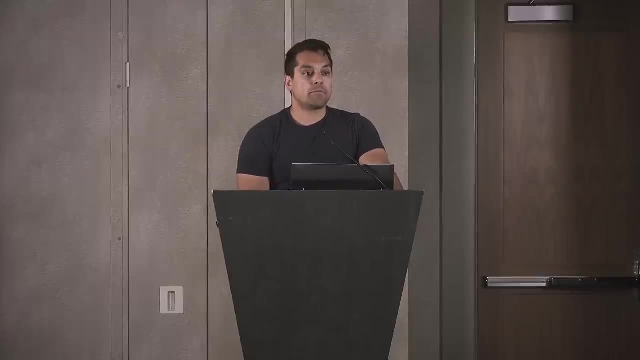 Yeah, I think with lifetime, I think that's fine. The boost signals too will. actually you can get a, an object that is kind of your position and you're the observer, and it kind of basically says: you put that in your destructor and say: 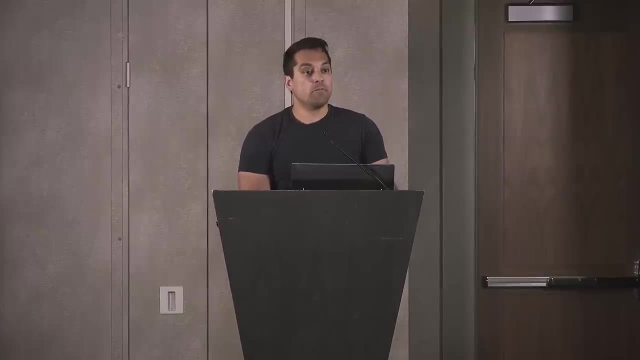 if I get destroyed, I'm actually gonna. it's like a callback. It pulls itself out of the subject, So you don't worry about the chance that your lifetime is getting misnamed. Yeah, So the comment was about looking at the boost library. 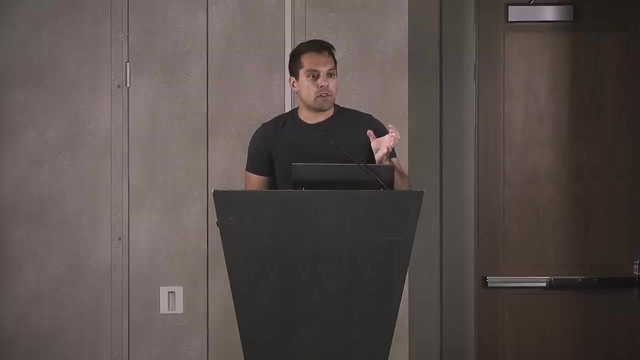 They've got a model for the observers are able to, I guess, get destroyed within the subject, to manage lifetime When you register. When you register, If you've got an object that says that's again, other side can manage. 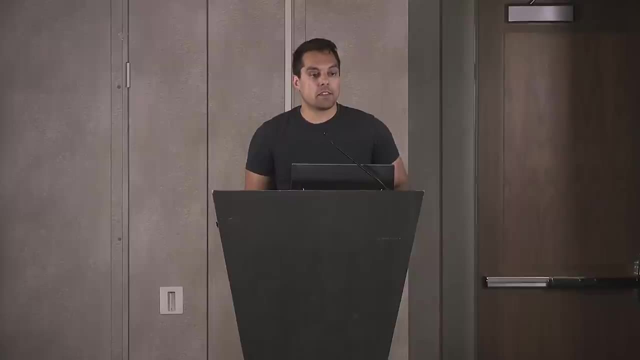 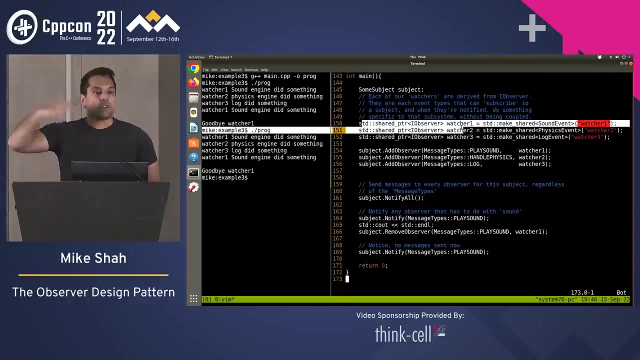 Oh sure, Then it's a way of controlling and even temporarily disconnecting a signal if you don't want to trigger it because it's smothered. Yeah, So we're not even creating, we're register, return an object and then it's already sort of maintained. 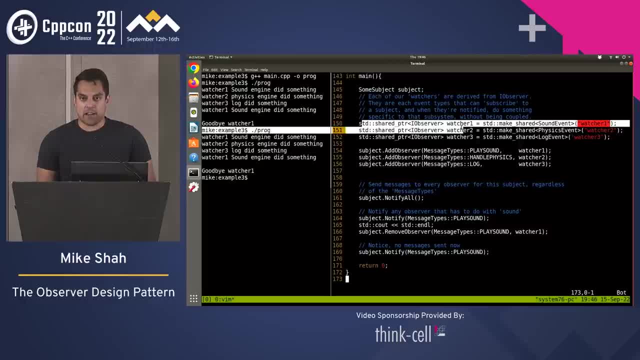 Yeah, There was something else I saw on. some folks make special observer pointer, smart pointer classes. That's something I wanted to dive into a little bit more to see what exactly those semantics look like, but it had me thinking about these sort of special use cases. 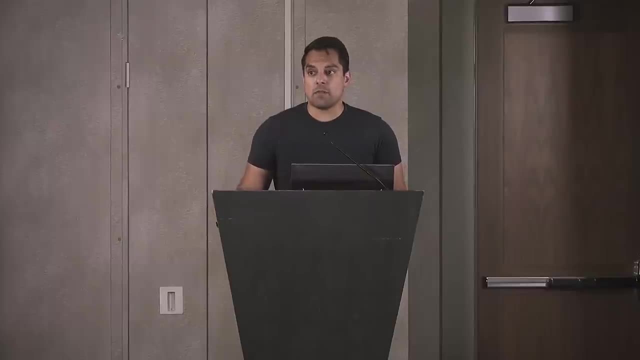 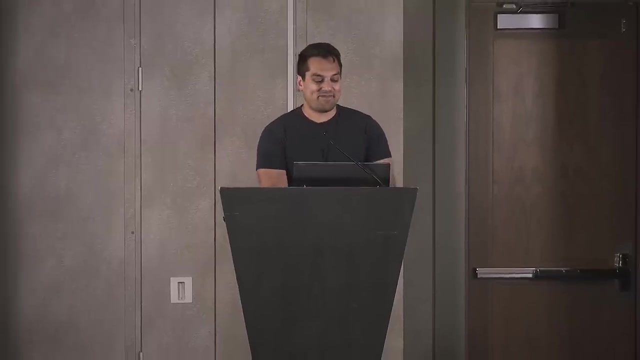 Yeah, So I think we're about at time, So I'll go ahead and thank you again and I'll hang around for questions as well. So, thank you, Thank you.